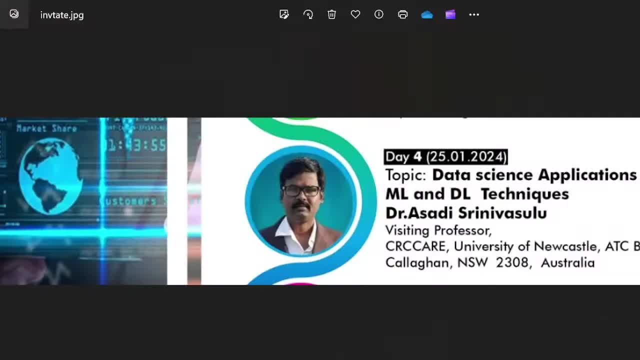 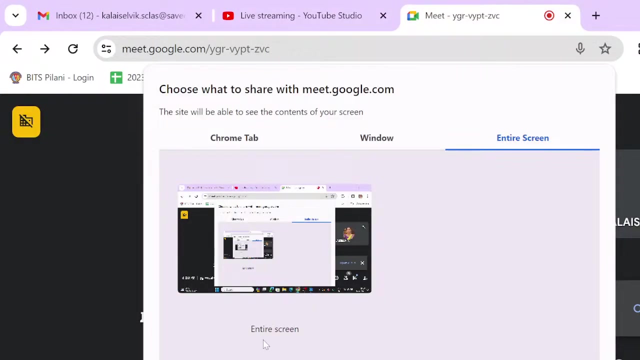 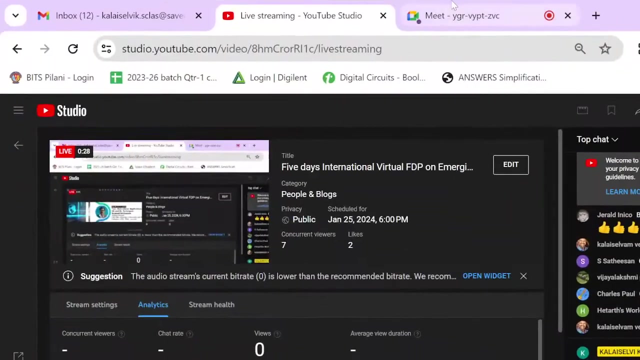 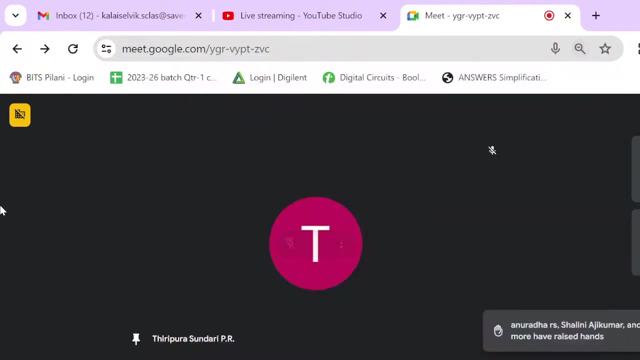 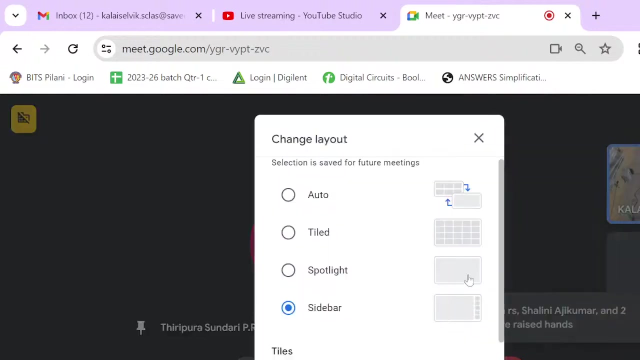 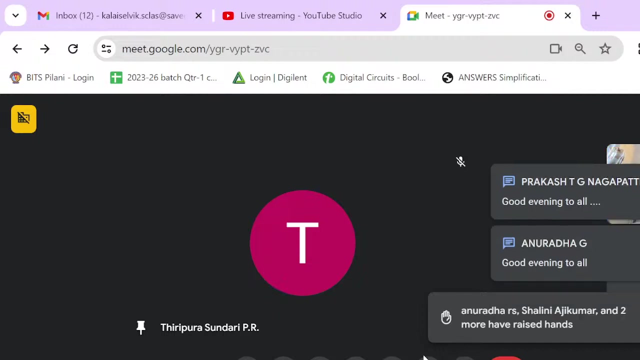 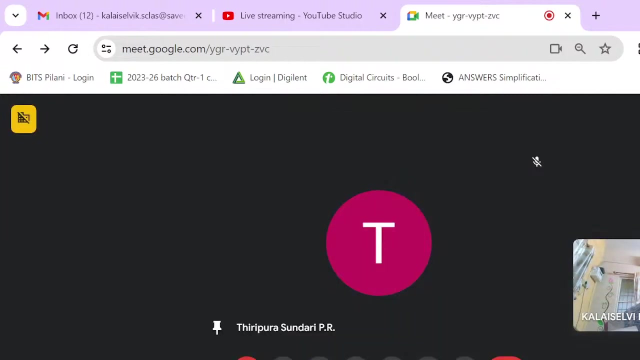 Thank you, Shall we start. Thank you, A warm, good evening to everyone present for the webinar on emerging trends in data analytics organized by Department of Data Analytics. I'm Dr Amita V, Assistant Professor, Savita College of Liberal Arts and Science. 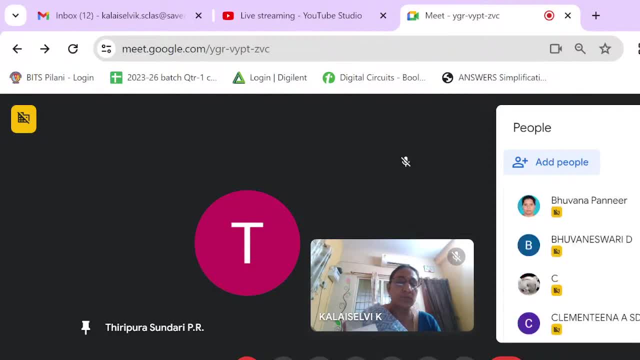 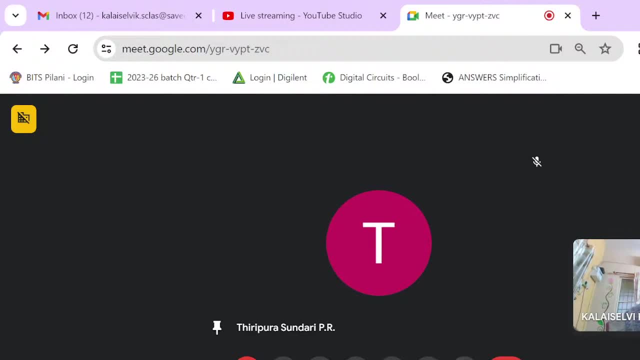 I feel privileged to extend our warm welcome to today's resource person, Dr Asadish, Universalist Sir, Distinguished Professor, Newcastle University, Australia. I also welcome all the participants from various reputed institutions to the five-day International Faculty Development Program. 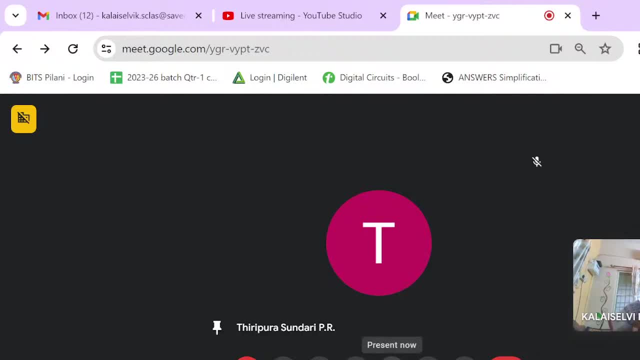 On behalf of our department, we extend our profound gratitude towards our respected Chancellor, Sir Dr N M Veerayan, Sir respected Director, Madam Dr Ramiya Deepak Ma'am, and our respected Principal, Ma'am Dr Gunita Arun Chandork Ma'am. 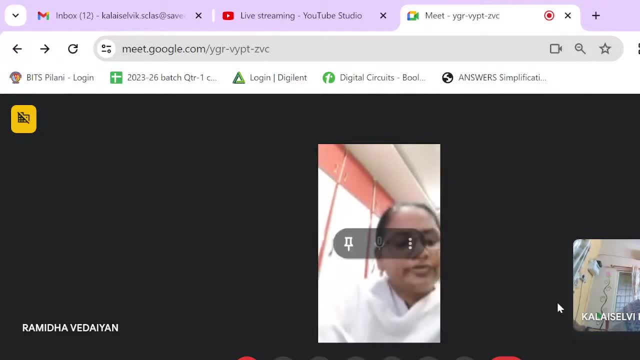 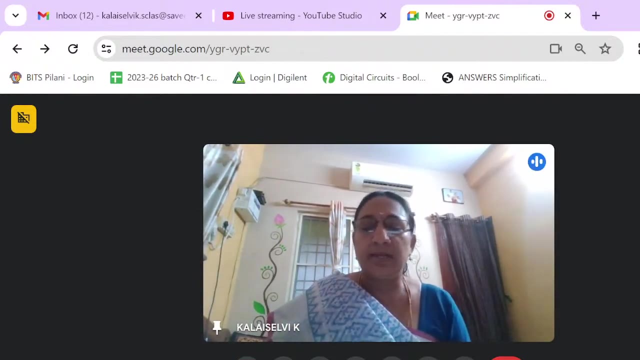 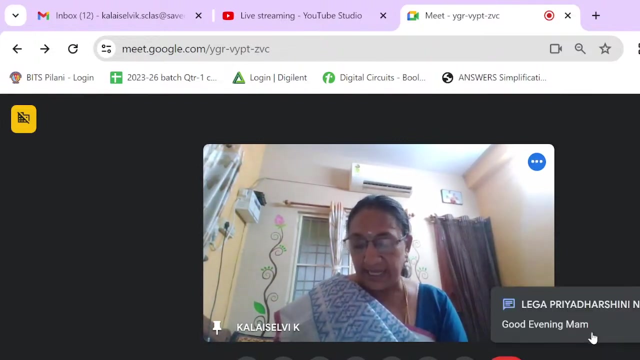 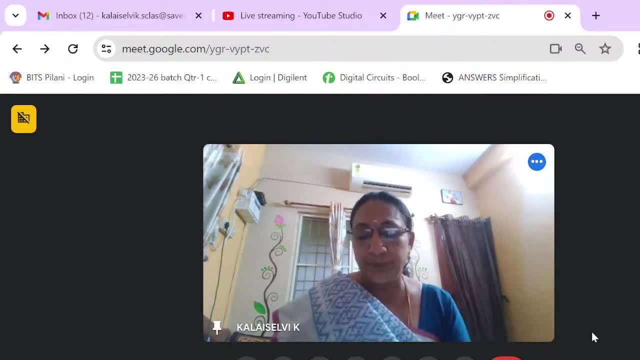 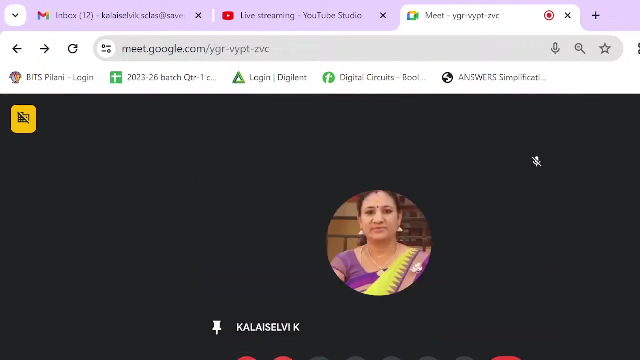 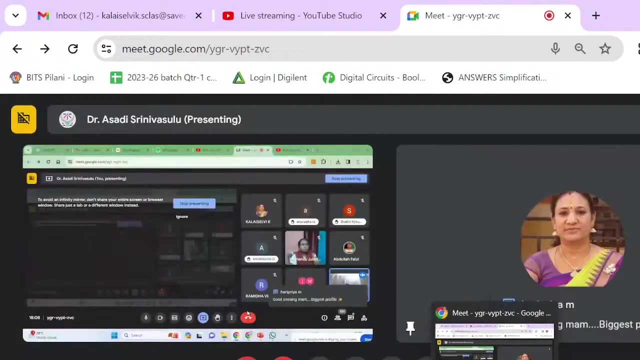 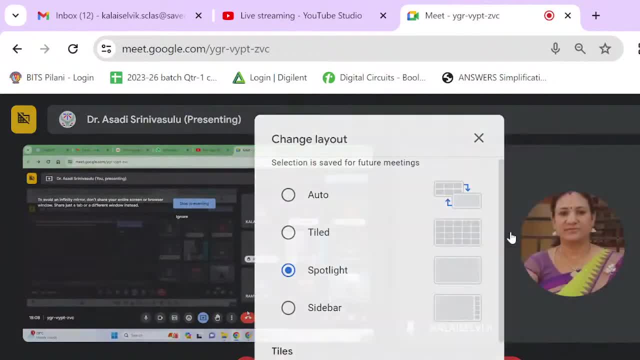 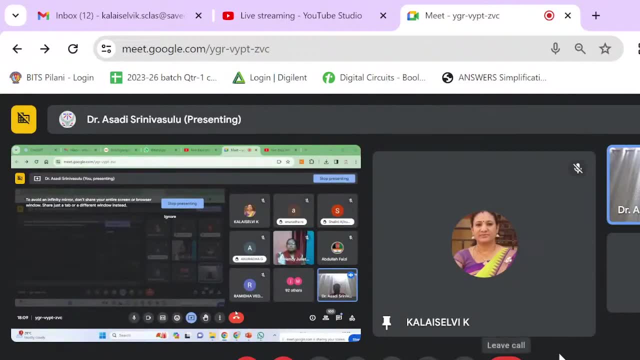 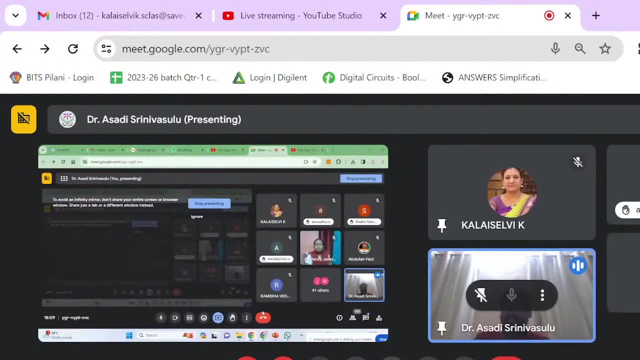 I started with data database management systems, data mining, big data and data science. Over the period, I learned many things, from raw data to refined data by using machine learning and deep learning and AI and statistical techniques. I have developed 150 projects. 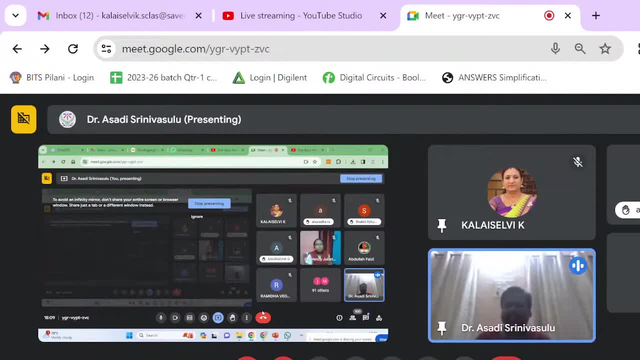 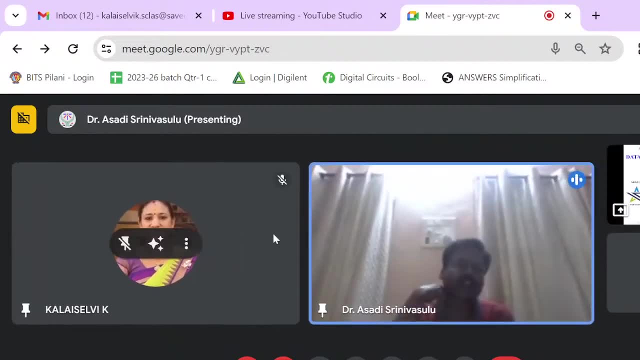 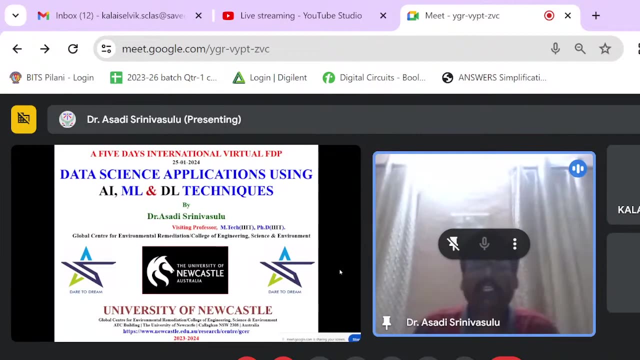 In my data science research laboratory with the help of masters and PhD students. Today, I would like to share my knowledge in the field of data science applications using artificial intelligence, machine learning and deep learning techniques. How do we develop a model? That model gives us a simplification of the reality. 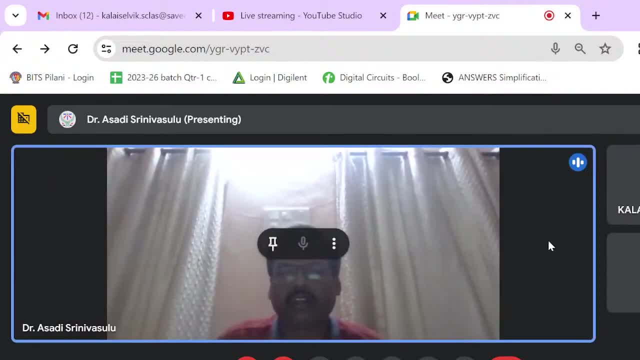 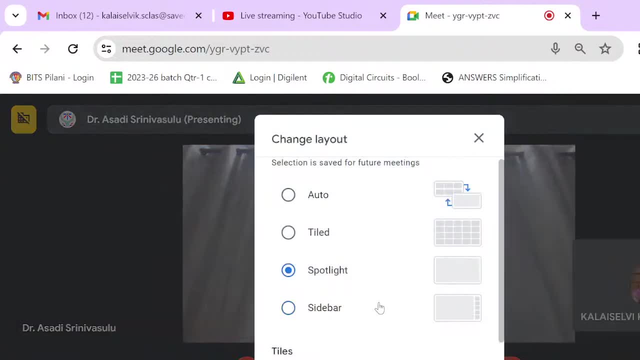 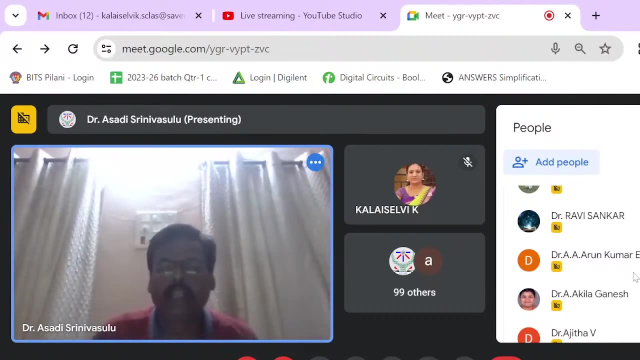 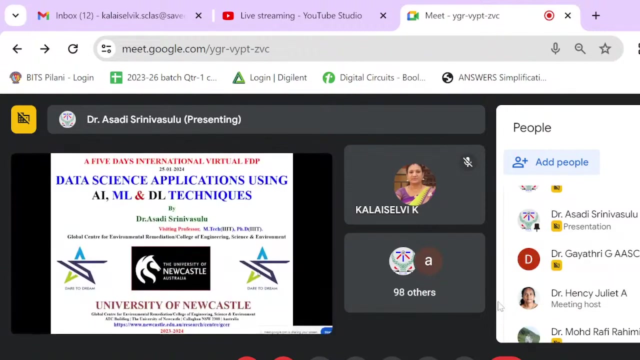 It gives the whether the data is right or wrong, With the help of classification, Structuring, association, rule, mining and outlier detection, And by using Python programming, various libraries I am using, like Pandas, NumPy, Scikit-learn, Tiano, PyTorch, TensorFlow, Keras, Pillow, etc. 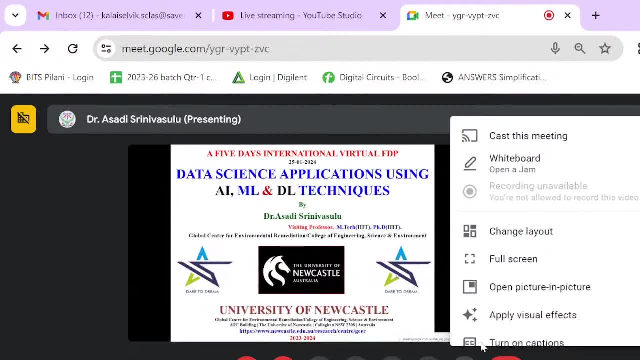 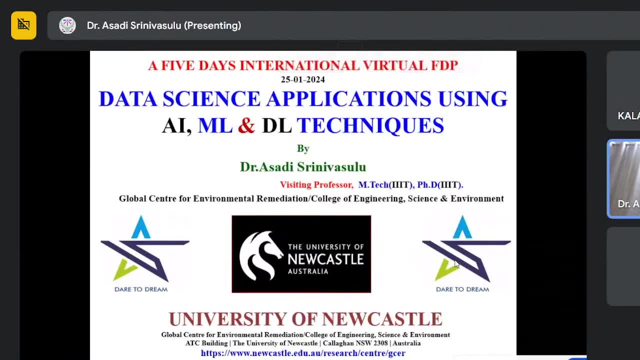 So, once again, a warm welcome to a five days international virtual faculty development program. My dear friends, Today, That day, you can clarify your doubts, Any doubts related to data database management system, data mining, big data and data science. 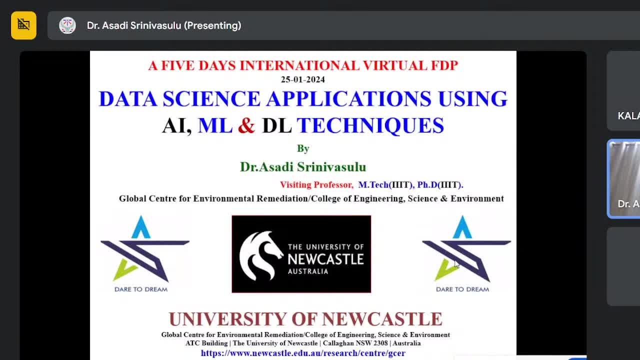 These are my expertized areas. Any doubt, any technique, any logic related to data science applications, especially in healthcare domain or insurance domain, weather forecasting domain, traffic and so on, And traffic analysis, SenseX, etc. Okay So, 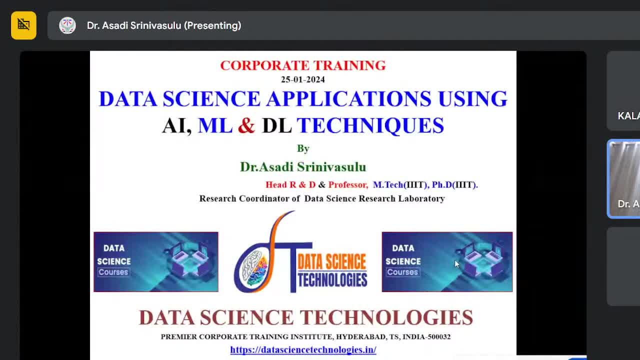 I'm a corporate trainer. Usually I'm demonstrating with the practical session on data science applications using AI, ML and DL Techniques. I used to give training for Google and TCS employees And cybersecurity and Internet of Things, blockchain technology- various. 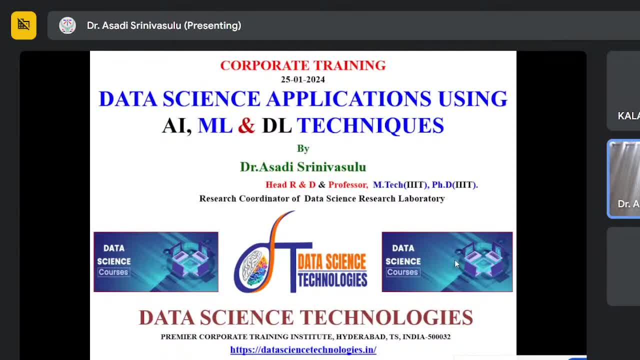 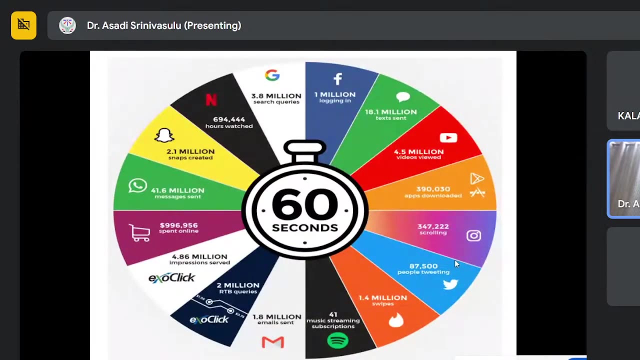 technologies, by using ai, statistical and mission and deep learning techniques. i'm using and i'm developing various models in order to predict or in order to detect, by using classification, clustering, association rule, mining, outlier detection. so, my dear friends, within 60 seconds, what is happening in this world, see how many users are connected to this internet world. 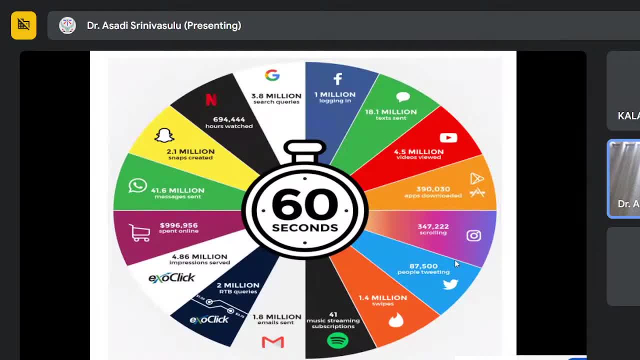 if you are using facebook netflix, see netflix 6 lakhs: 94,444 hours watched. 3.8 million such queries, 1 million logging in, 18. million text sent. a 1.8 million email sent. where the data is coming from? how to store the data? how many? 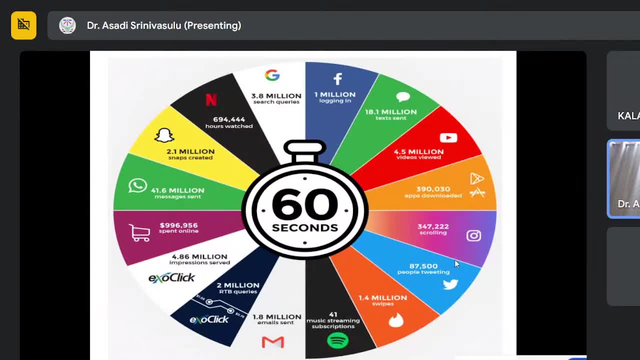 data is coming from, how to store the data. how many data is coming from. how to store the data. how many servers are required to store a huge volume of data, so you may get doubts, or how many servers are required. that's why we are going towards cloud computing. cloud computing is nothing but. 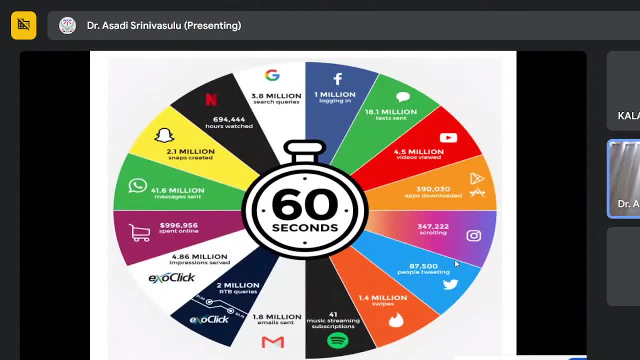 internet-based technology. so so every mnc having their own data center. data center is nothing but collection of high integrated servers at one place is called data center. data center. backbone is a virtualization and high computing servers see even cloud computing. backbone is data center and virtualization. virtualization is the ability to perform multiple tasks in a single system. 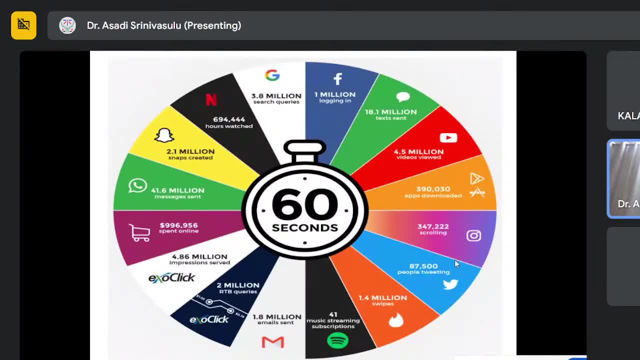 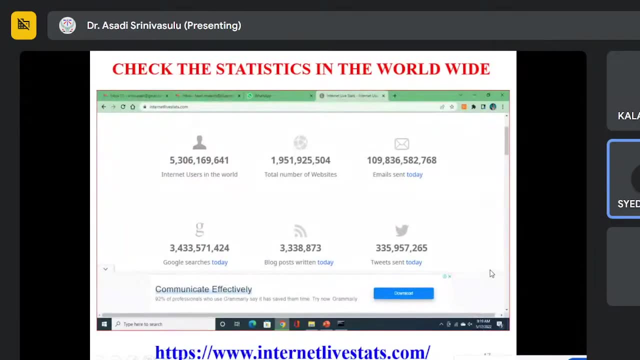 with the help of vmware, hypervisor, gen, virtual iron. these are the popular virtualization technologies we are using in order to store huge volume of data. i believe some voice, some noise is coming. please unmute yourself. so if you want to see the statistics in this worldwide, just go to wwwinternetlivestatscom. 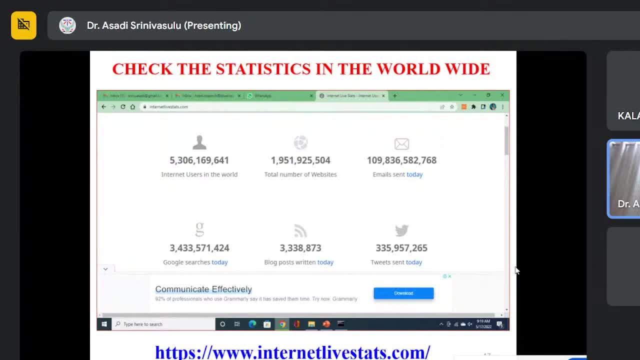 you come to know how many users are connected in this, in this second, in this minute, 60 seconds per minute. how many users are connected right now? can you, can anyone read this number? 5 billion 306 million 169 641? see by reading itself. we are feeling tough. that means per second. 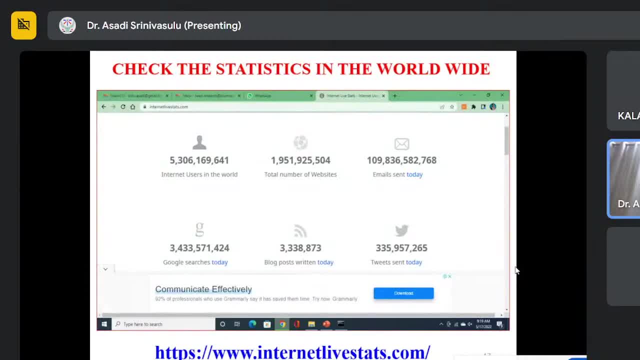 per minute. how many users are connected to this internet world? what is internet? network of networks? what is network? interconnection between the systems in the fashion of local area network, wide area network, metropolitan area network. okay, so these are the statistics that we are getting here for the statistics of worldwide. through internet, we can see the internet live statisticscom. 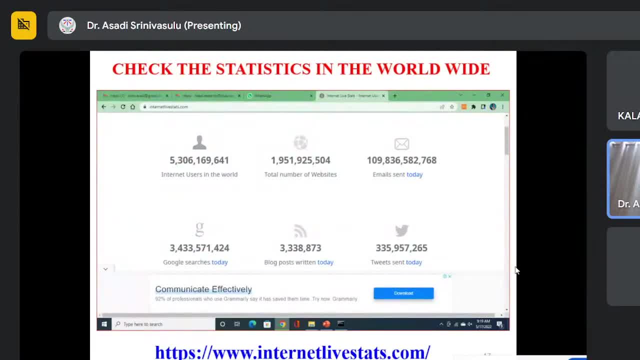 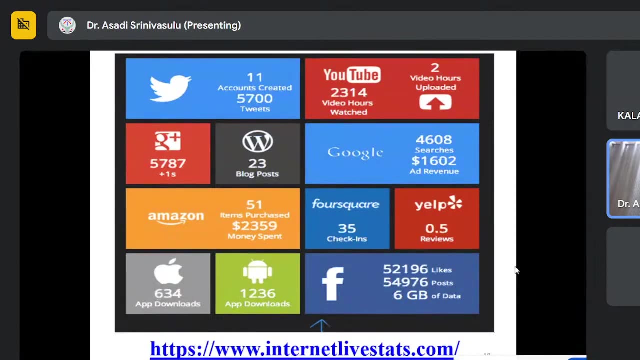 total number of websites opened in this one, so you may get out, sir, where the data is coming from and where the data is going, and how many servers are required to store huge volume of data. so that's why we are going for cloud computing. cloud computing is a 543 formula. 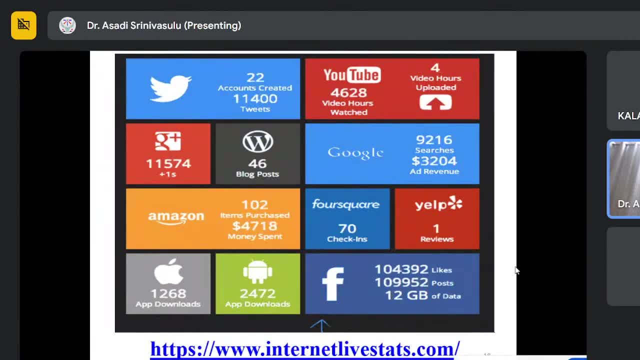 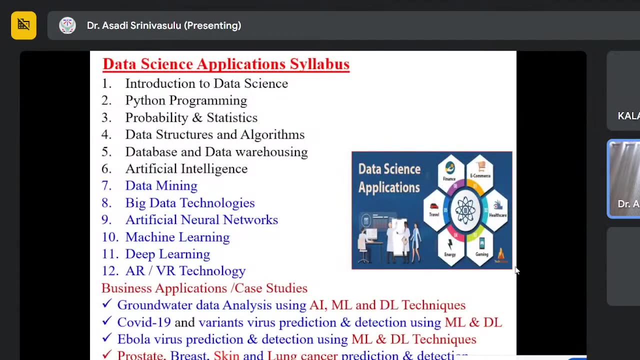 five characteristics for internet live statistics, infrastructure models and three services. so this one same i have incorporated in the slide also. the numbers are increasing, automatically. the data center also increases. so this is the syllabus today. i would like to give you a brief introduction about all the topics, what i am going to cover in 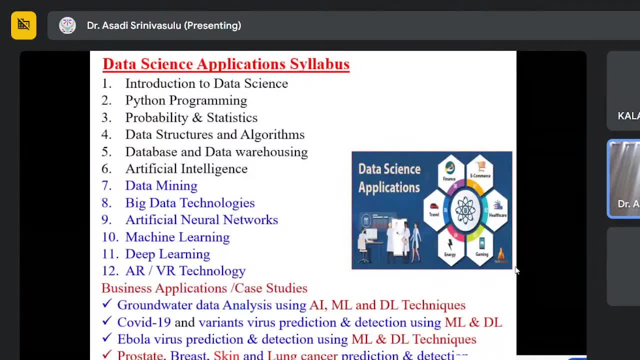 this data science application with the syllabus. usually this is a corporate syllabus. i'm a corporate trainer for all employees who are having 10 years of experience for them. i am going to demonstrate with the practical session by using python programming libraries like tensorflow, keras pythons, tiano, pandas, numpy pillow, etc. so here are 12 major components of data science. 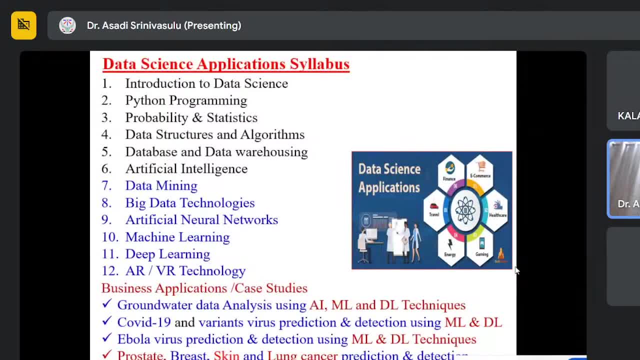 syllabus introduction to data science, what i am going to cover. so what are the dimensional functions of data science? what are the characteristics, what are the tools and techniques we are using in order to predict and detect various scientific applications? then python programming. there are two types of python programming we are using. 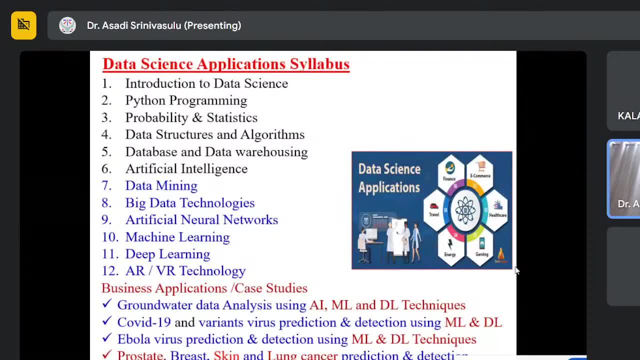 core python programming and advanced python programming. so everybody knows core python programming. if you know basic mathematics, you can learn very easily. if you know advanced mathematics knowledge and statistical knowledge then you can go for advanced python programming like numpy, pandas, scikit-learn, sklearn, tiano, pytharch, keras, tensorflow pillow, etc. seaborn. 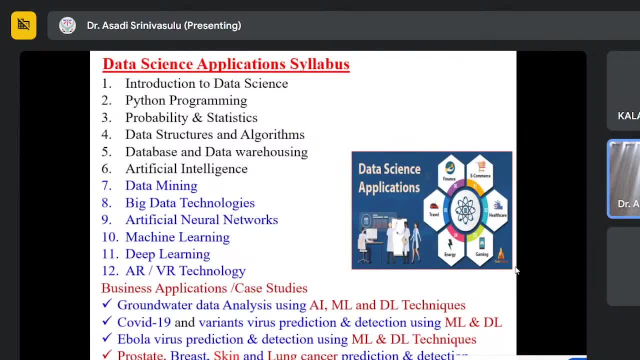 matplotlib, etc. these are the various libraries we are using under advanced python programming. probability and statistics is the pre-requisition for data science. if you know probability and statistics, you can do the wonders in order to extract the meaningful insights from the huge volume of data by using statistical and artificial intelligence. 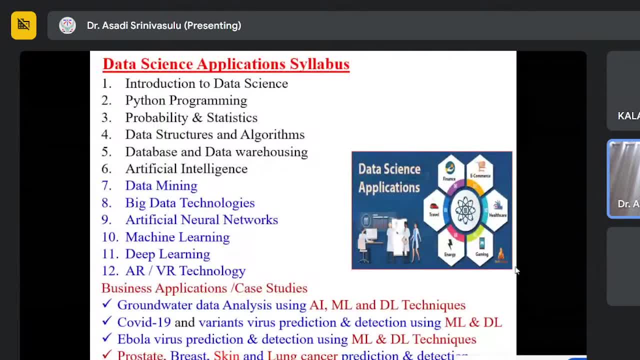 and machine and deep learning techniques, then after that, data structures and algorithms. data structure is a systematic way of organizing data and accessing the data and representing the data and organizing the data a bit differently than those which we are using at the moment. well, thanks a lot, katya. thank you very much for your time. you are welcome, all right, so. 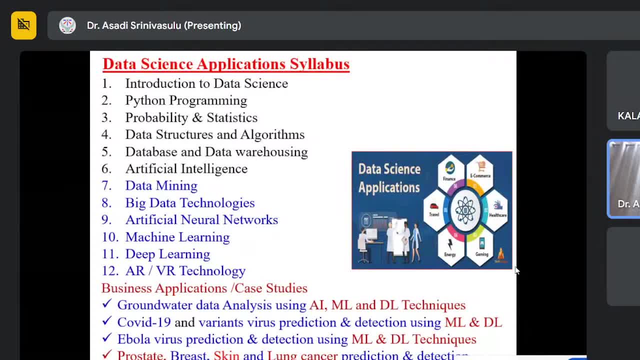 in the fashion of linear and non-linear fashion, by using sorting, searching and data structure approaches like dynamic programming, greedy approach, branch and bound, and these are the various approaches we are using. Then, after that, database and data warehousing. Database is a collection of interrelated data. 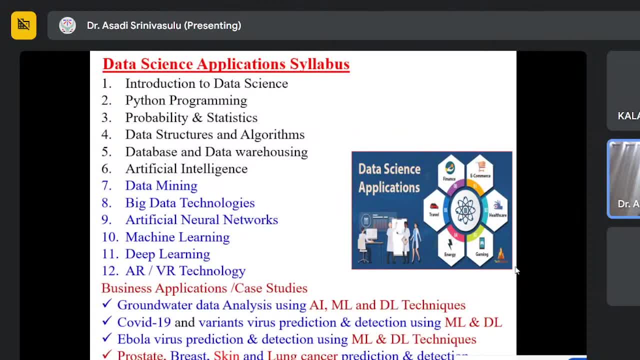 To manage the data, we are using relational database tools like SQL, MySQL, Teradata, DB2, MS Access. In order to store a huge volume of data with help of tables is called database. Collection of tables is called database. In order to store a huge volume of data with help of data cubes, we are going for data. 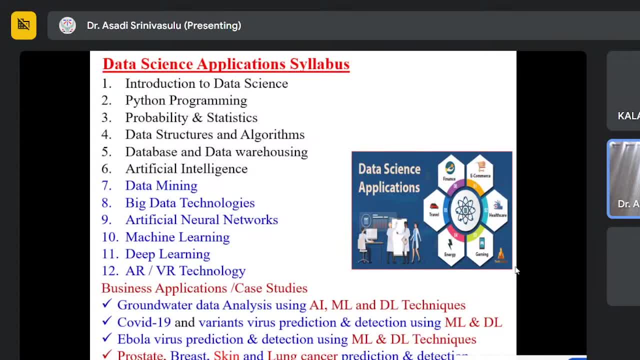 warehousing. Data warehousing is used to store a huge volume of data in the server Collection of servers is called data center. Data center is the backbone for cloud computing. Then artificial intelligence- intelligent behavior in a machine- is called robot. We have voice recognition robots like Siri, Alexa. 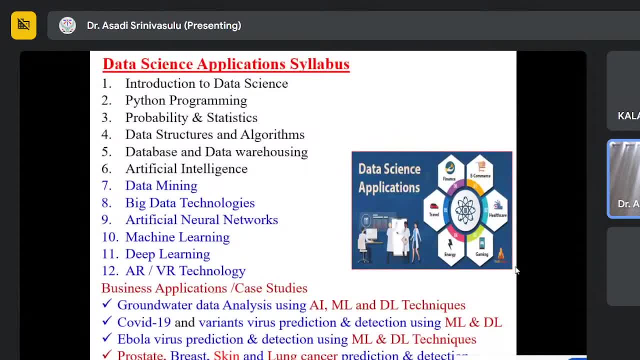 We have humanoid robots like Sophia, Asimo, etc. So science and engineering to develop intelligent applications by using AI models. After that, data mining. Data mining is the process of extracting meaningful interested patterns from the huge volume of data by using classification, clustering, association rule mining, outlier detection. 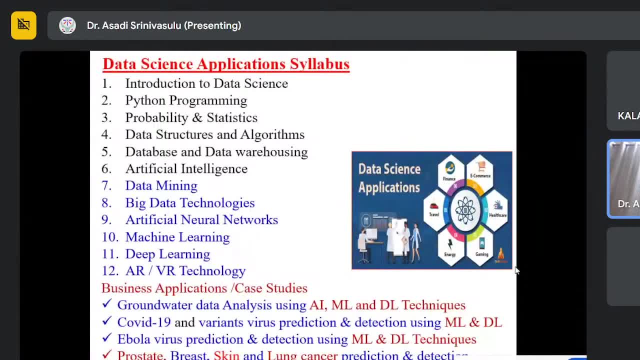 So, after that big data technologies, Which data we can call it as a big data? My dear friends, can anyone answer to my question: Which data we can call it as a big data? I'm giving the answer: Traditional systems are unable to process the data. 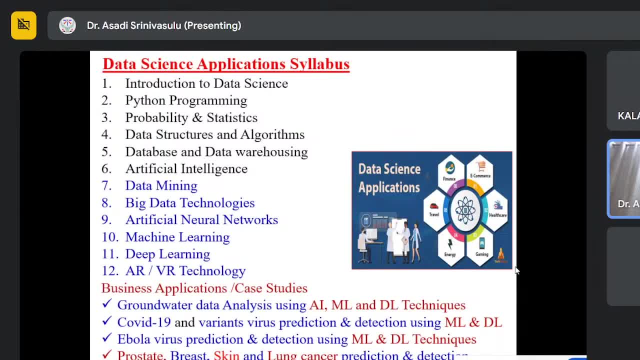 Such type of data is called big data. That's why we are going for high computing servers, like we are using MATLAB, Hive, HBase, Zookeeper, Scoop, Hive, etc. So, in order to perform Hadoop and MapReduce, MATLAB and Python programming, in order to 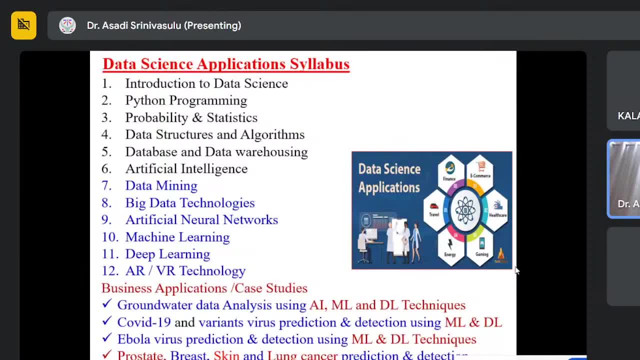 process, the major components Of big data technologies called HDFS and MapReduce. So we are using Java programming in order to perform classification, clustering, association, rule mining, outlier detection- By using Java, Python, JavaScript and Julia. these are the programming languages. 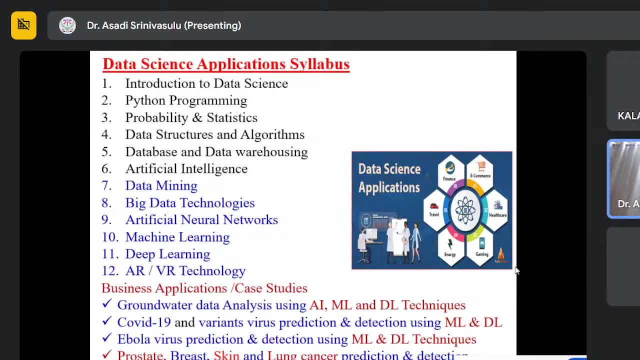 Then I'm going to explain artificial neural networks based on the biological neuron. how to create artificial neural networks By using ANN, CNN, RNN and LSTM- long short-term memory. These are the various advanced artificial neural networks we are using in order to perform. 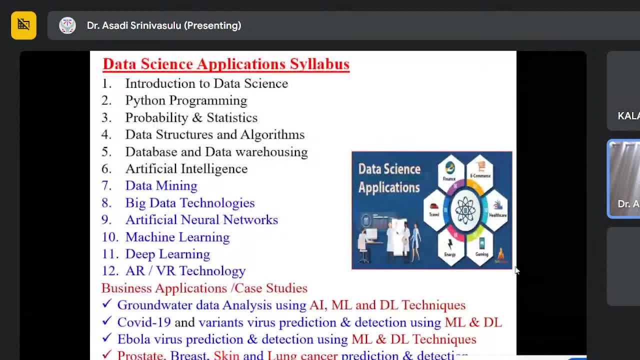 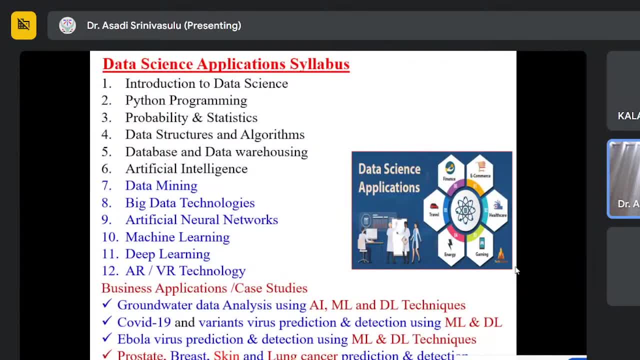 Machine learning, like supervised learning, unsupervised learning and semi-supervised learning or reinforcement learning. What is meant by supervised learning? There is a label, there is a target class. Based on the target class, we are classifying the data. 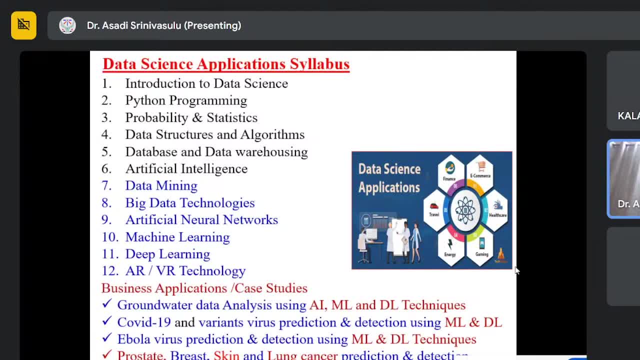 That is called classification by using SVM technique, decision tree, neural networks, Bayesian networks, etc. Then unsupervised learning. So There is no label, there is no target class, but based on the similarity measure we are classifying the data. 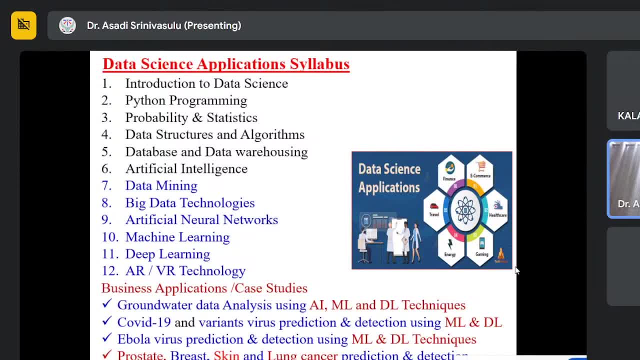 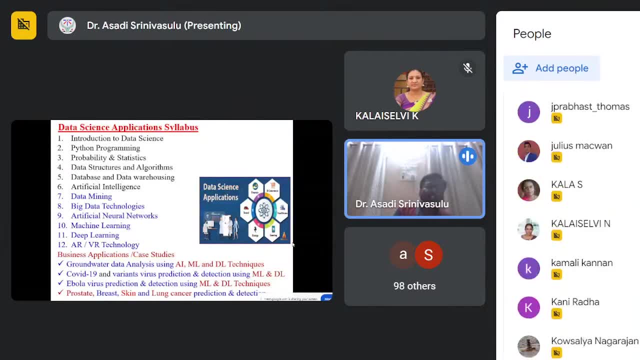 That is called clustering. There are clustering is nothing but based on the similarity measure. the objects are behaving similarity between among the objects. So similarity measure: how to find out square root of X1 minus X2, whole square, plus Y1 minus Y2 whole square. 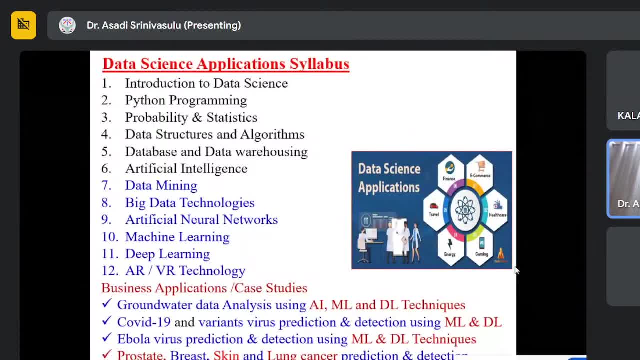 Y1 minus Y2, whole square. Then Then reinforcement learning is nothing but based on the punishment and reward. we are solving the problems, especially in gaming applications. we are using reinforcement learning. There are various techniques under reinforcement learning. I am going to demonstrate. 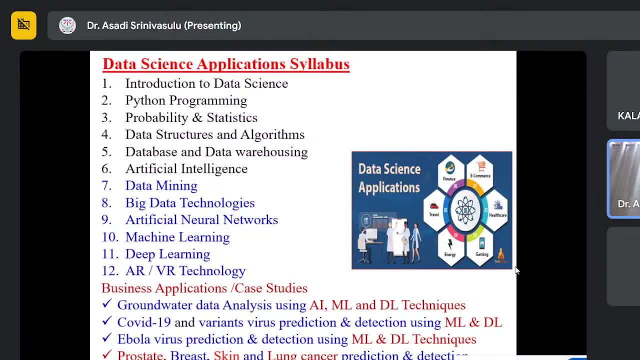 Then deep learning: Learning from the observational data with a deep manner by applying various input and hidden layers, By using convolutional neural networks, Recurrent neural networks, long, long shorter memory techniques, and there are various frameworks we are using in deep learning techniques like tensorflow, Keras, PyTorch and matplotlib. 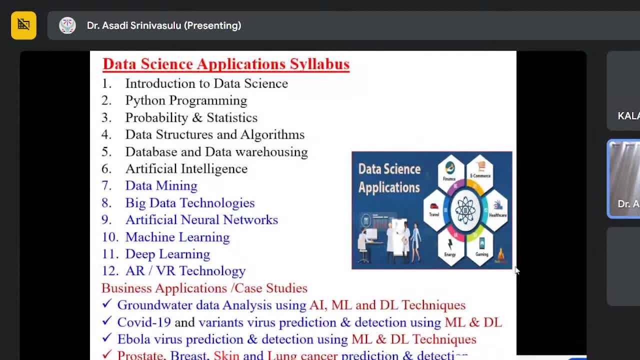 piano and sklearn, scikit-learn and NumPy, Pandas, Pillow, etc. Then augmented reality, virtual reality. Nowadays, This is the latest trend, Latest technology in the field of audio and video applications in order to perform we. 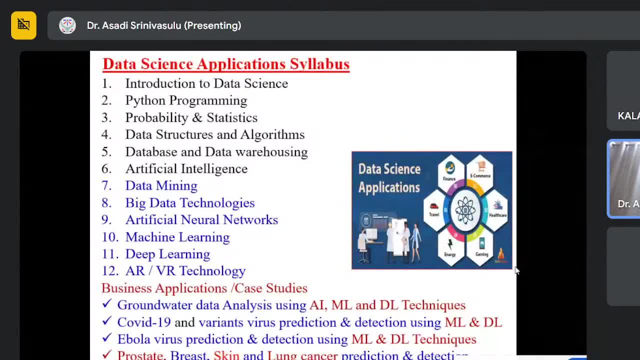 are using AR and VR technology. So these are the 12 topics I am going to demonstrate and business applications and case studies. So right now I am doing groundwater data prediction and detection by using artificial intelligence, statistical and mission and deep learning techniques Under my GSER language. 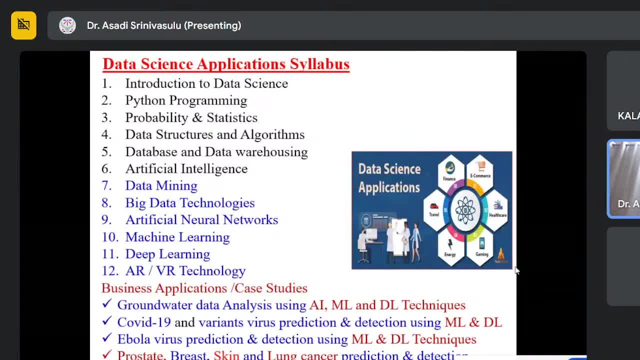 Under my GSER laboratory at the University of Newcastle, Australia. Actually, I got Australia government groundwater data data. There I'm using pre-processing techniques like binning and box-blast technique. After that I am applying various models, like statistical models, like linear regression. 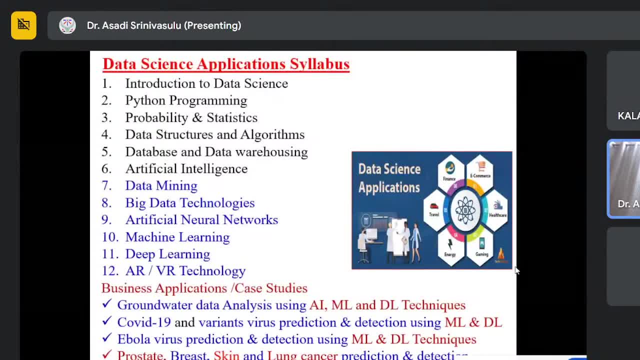 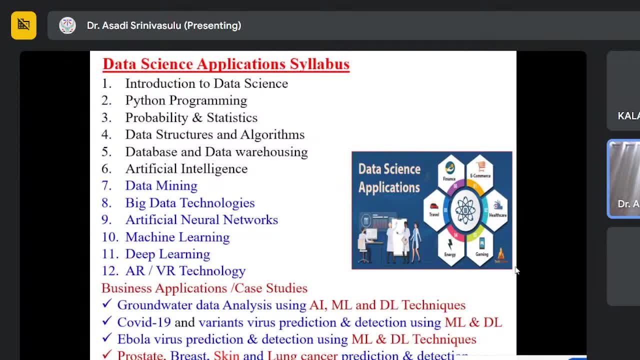 Then COVID-19, virus prediction and detection variants are coming nowadays still Variants. you can see nowadays also these kind of viruses. So virus expansion is vital information resource under C's that is computer related virus and COVID-19 virus is different. 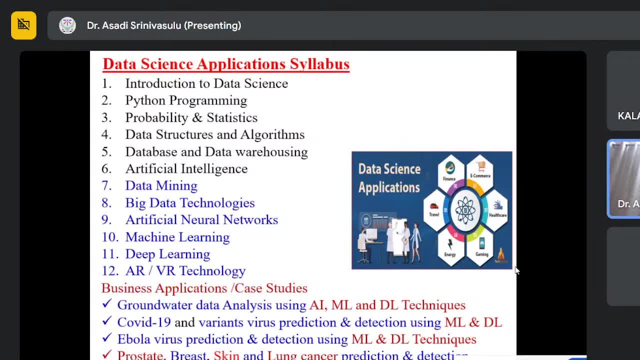 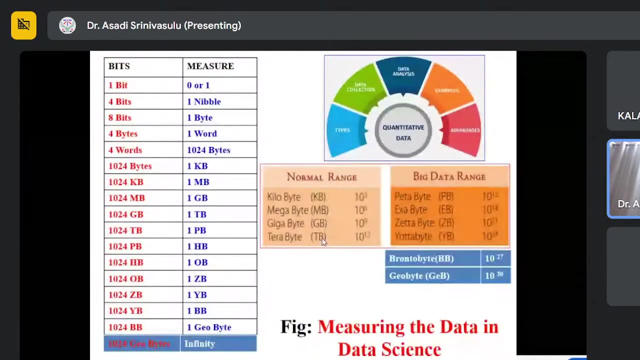 And by using various ML and DL techniques, we are predicting and detecting health data analytics: Ebola virus prediction and detection using ML and DL techniques, then prostate, breast skin and lung cancer: lung cancer prediction, detection by using various techniques. So so, my dear participants, any doubts? 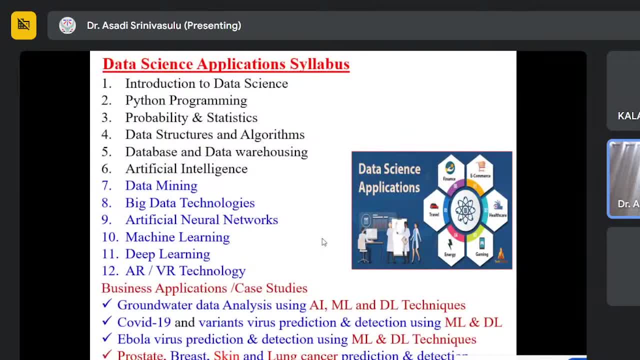 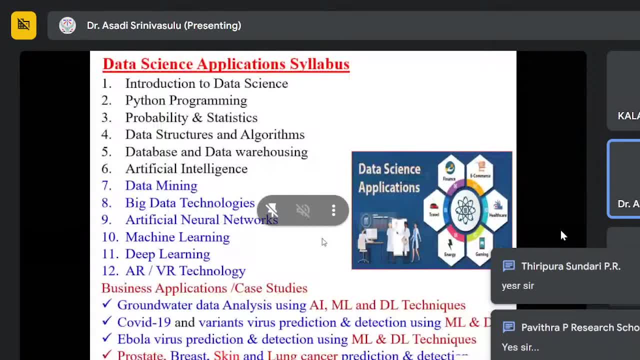 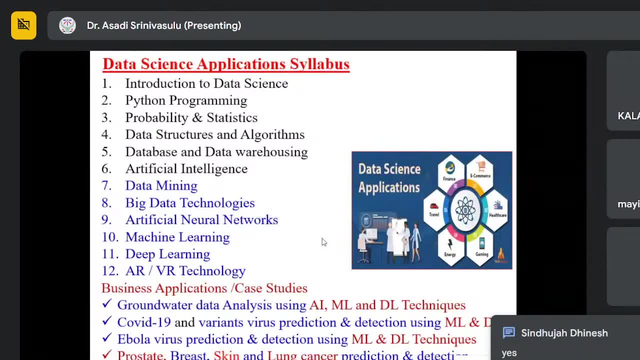 Yes, sir, Any doubts If you are having, please, if you are unable to ask, just give in the chat box. I'm going to clarify the doubts. Thank you, sir. If no doubts, I'm going Okay. 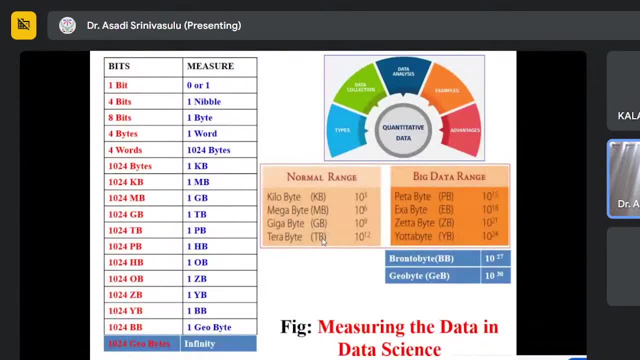 Okay, So measuring the data in data science, Sir, a huge volume of data is there. I don't know the measurement of in server and data center. See, if you press capital, A system cannot understand. Is it right or wrong? 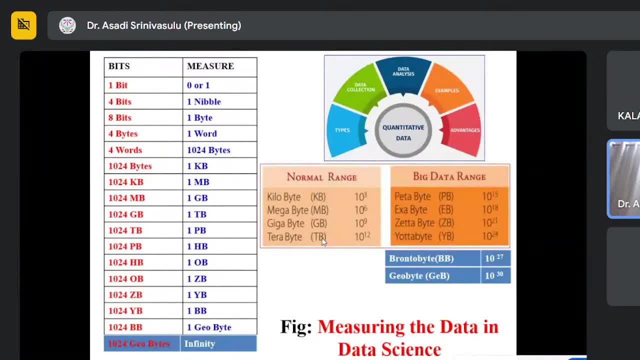 System cannot understand Internally, it converts into ASCII format. ASCII stands for American Standard Code for Information Interchange. ASCII stands for American Standard Code for Information Interchange. In the keyboard, total 106 to 108 keys are there, Every key having its own ASCII value. 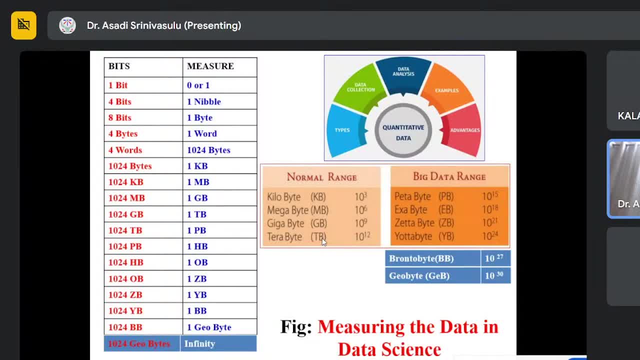 Okay. So if you press capital, A system cannot understand. Internally it converts capital A value is 65.. If you divide it by 2, it gives the binary equivalent number is 10001.. This is the binary equivalent number internally, within fraction of seconds. 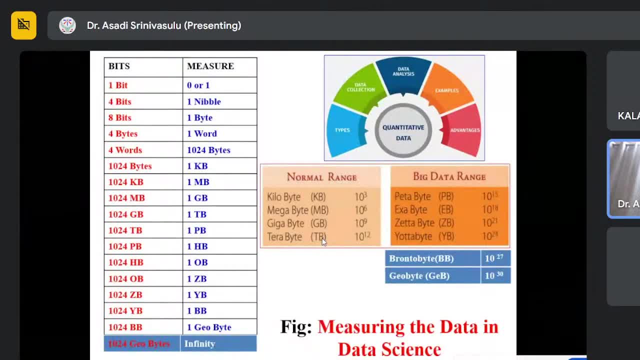 It is giving. it is typing in our monitor capital A. Oh, you have pressed capital A Like: 1 bit is equal to 0R1.. 4 bits is equal to 1 nibble. 8 bits is equal to 1 byte. 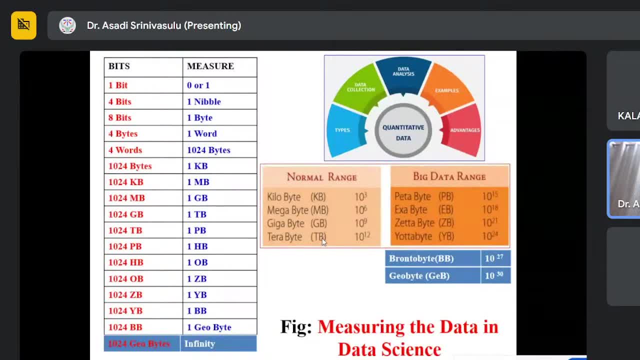 4 bytes is equal to 1 word. 4 words is equal to 1024 bytes. 1024 bytes is equal to 1 kilobyte. 1024 kilobytes is equal to 1 megabyte. 1024 megabytes is equal to 1 gigabyte. 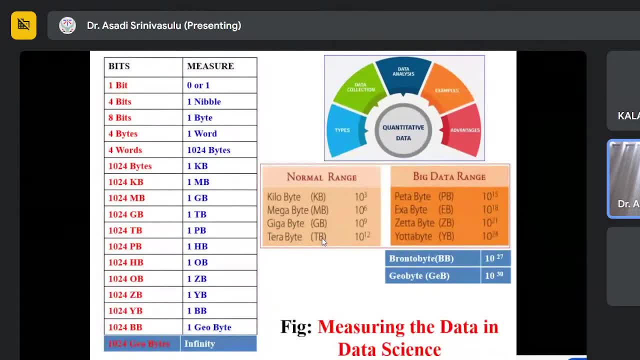 1024 gigabytes is equal to 1 terabyte. 1024 terabytes is equal to 1 petabyte. 1024 petabytes is equal to 1 hexabyte. 1024 exabyte is equal to 1 octabyte. 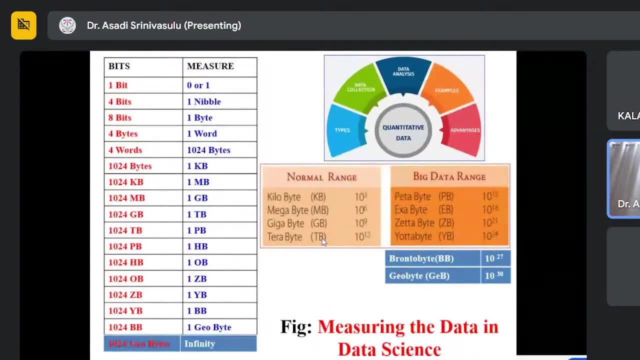 1024 octabyte is equal to 1 zettabyte, 1024 zettabyte is equal to 1 yottabyte And 1024 yottabyte is equal to 1 brontobite. See before RoboMovie. even I don't know and we don't know. 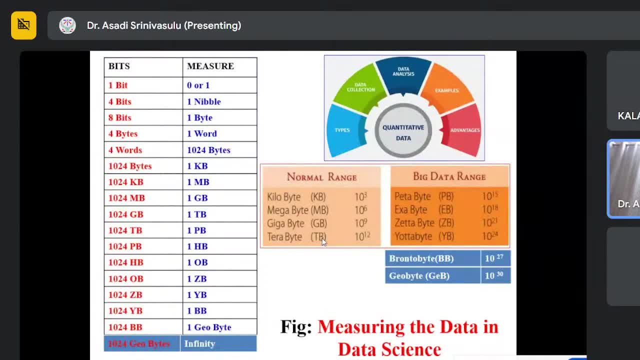 The terminology is there or not. How do we measure the data in data science or data mining? After that RoboMovie, we came to know there is a terminology to measure the data Like: hi, I am Robo, My speed is 1 terabyte. 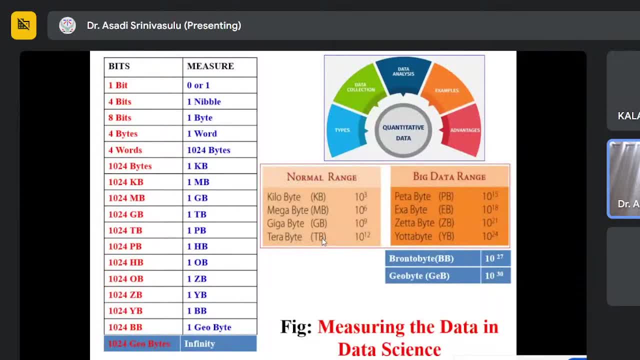 My memory is 1 zettabyte. After that movie only we came to know this is the terminology we are using to measure the huge volume of data in data science. So yesterday night I searched. There are two more terminologies presented. 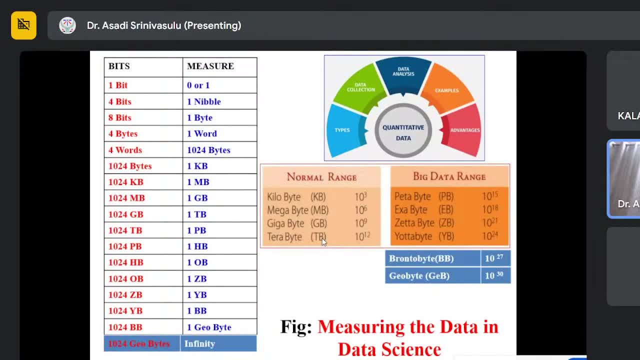 1024 yottabyte is equal to 1 brontobite BB. Keep in mind, my dear friends, 1024 brontobite is equal to 1 geobite. 1024 geobite is equal to infinity. 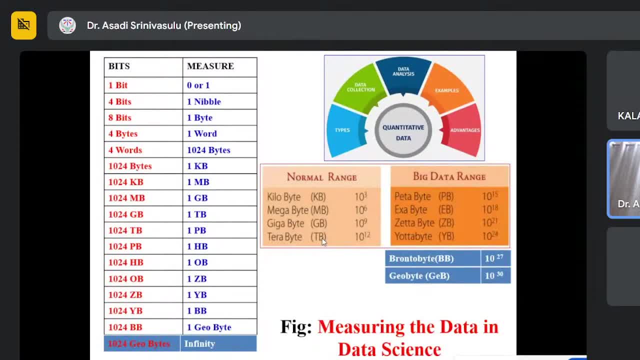 If you ask me after that, there is no terminology, See same terminology. if you see the normal range and big data range: 1 kilobyte is 10 power 3,. 1 megabyte is 10 power 6,. 1 gigabyte is 10 power 9,. 1 terabyte is 10 power 12.. 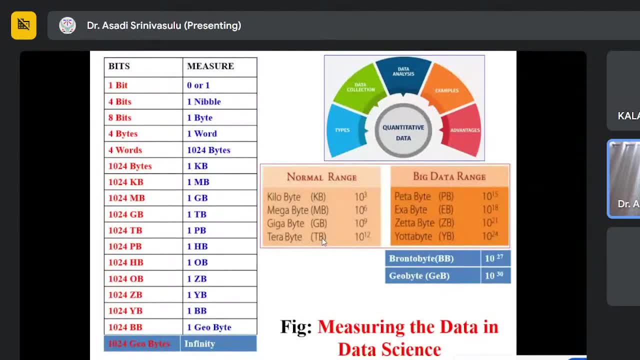 In big data range: petabyte is 10 power 15,. hexabyte is 10 power 18,. zettabyte is 10 power 21,. yottabyte is 10 power 24,. brontobite is 10 power 27,. geobite is 10 power 30.. 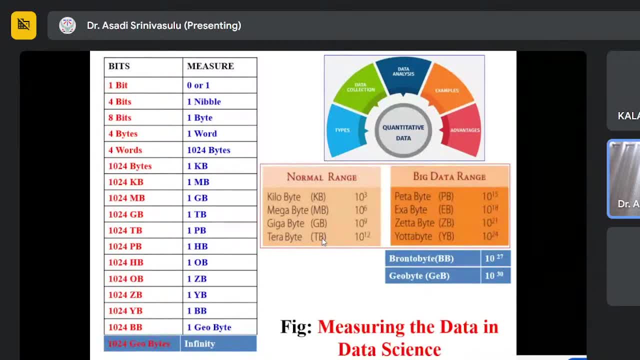 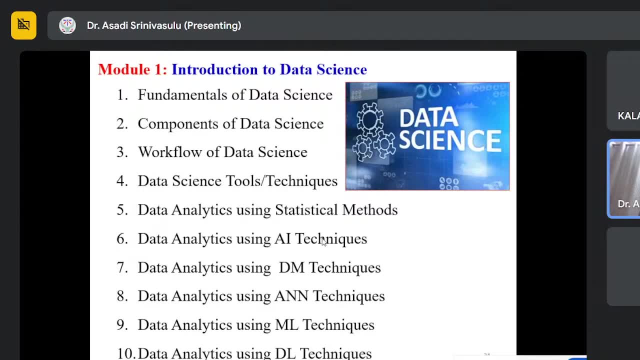 This is the way we are measuring the data in data science. So this is the syllabus I am going to cover. I have explained already fundamentals, components, workflow of data science and what are the tools and techniques And what are the AI techniques. 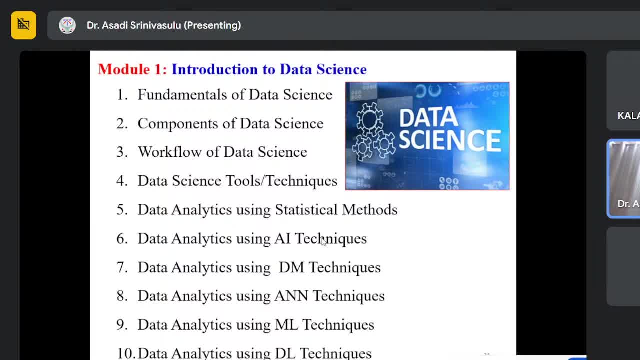 In order to perform data analytics using statistical methods like linear regression, nonlinear regression, logistic regression, etc. Data analytics using AI techniques like A star algorithm and various statistical AI ML techniques. we are integrating in this AI techniques. Data analytics using data mining techniques like classification, clustering, association rule mining, outlier detection, etc. 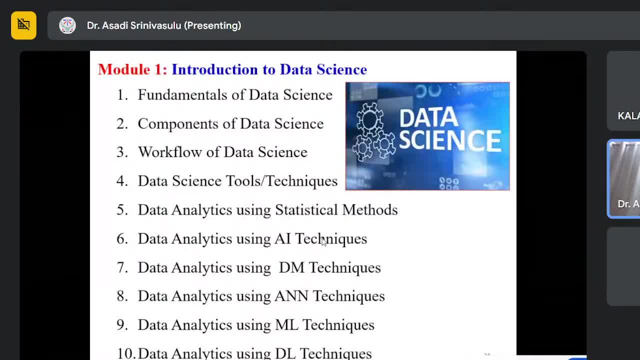 And data analytics using artificial neural networks. it is a classification technique And here we are using various hidden and input layers and various activation functions in order to predict and detect of any data. Data analytics using machine learning techniques like supervised learning techniques, unsupervised learning techniques and reinforcement learning techniques. 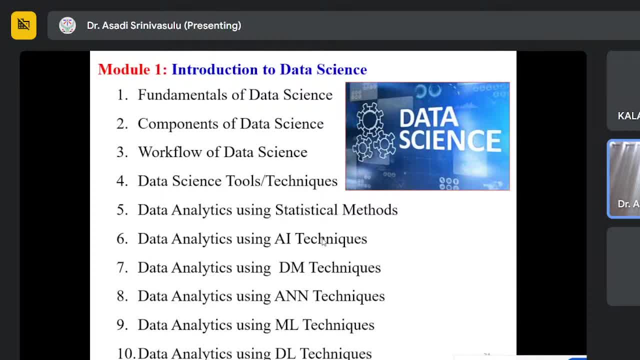 Then data analytics. Data analytics using deep learning techniques, like learning from the observational data with a deep manner, by using ANN, CNN, RNN, LSTM, TensorFlow, Keras and SKlearn, Scikit-learn, Theano, PyTorch, Matplotlib, Pillow Pandas, NumPy. 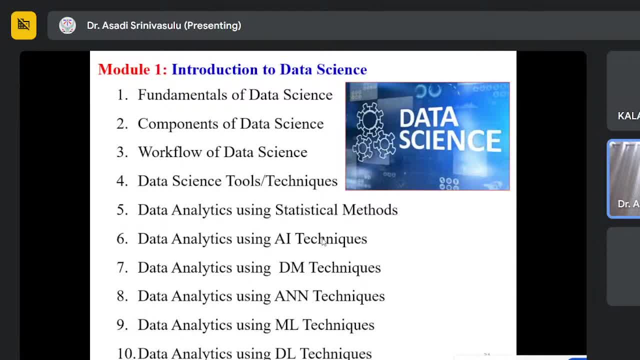 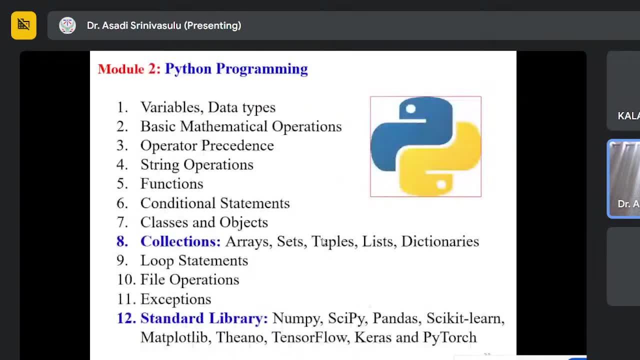 Various frameworks. we are integrating and developing various models in order to predict and detect the various applications, And so Python programming. I have explained already, So core Python programming and advanced Python programming. In core Python programming everybody knows variables, operations, operator, precedence, string, functions, conditional statements, classes and objects. 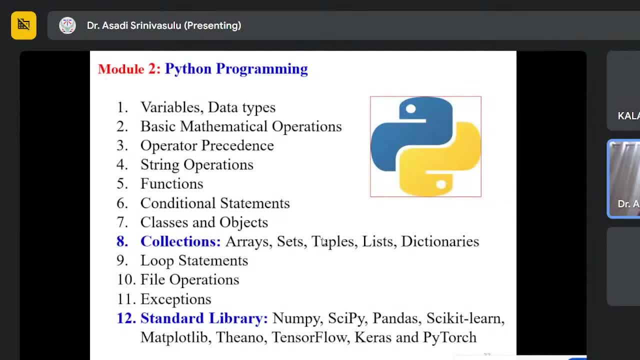 Python collections like array sets, tuples, list, dictionaries, loop statements, file operations and exceptions. Advanced Python programming: we are using NumPy- SciPy See. NumPy means numerical Python, SciPy means scientific Python Pandas in order to describe about data sets like tables. 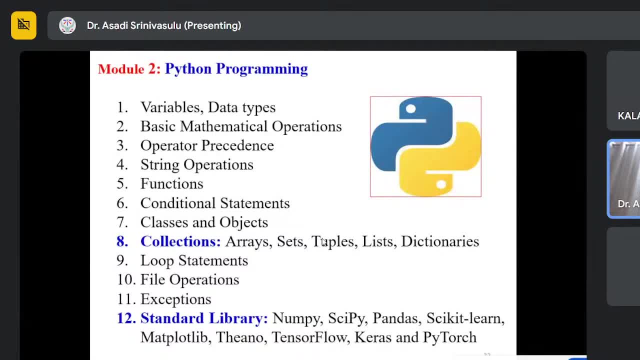 Okay, Then Scikit-learn for machine learning algorithm purpose. we are using Matplotlib for generating visualization graphs, Theano for big data analytics, TensorFlow for artificial intelligence and big data applications, Keras especially for deep learning and machine learning applications. Okay, 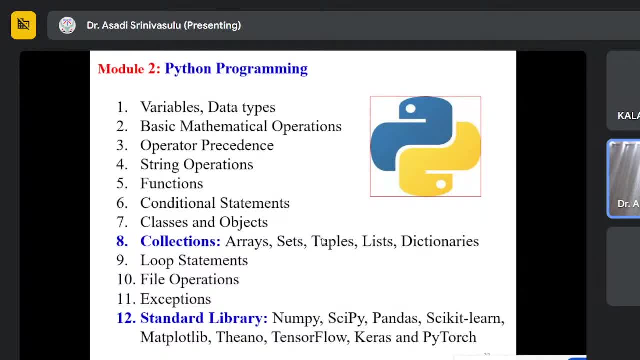 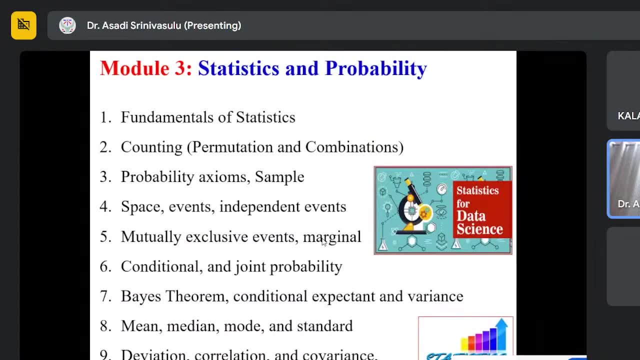 PyTorch for only machine learning applications. These are the frameworks, or libraries or packages. Then statistics and probability. We know various operations we are using, like addition, subtraction and count: total, maximum value, minimum value, mean, median mode, standard deviation, covariance, correlation. 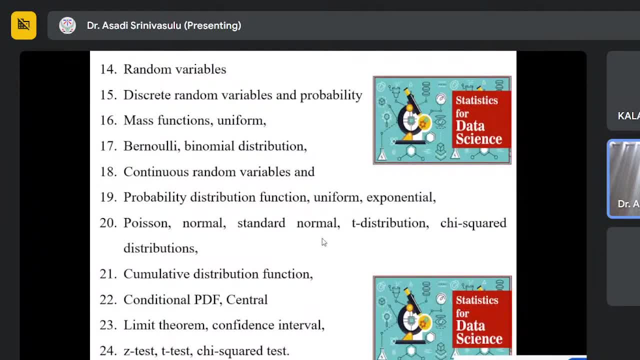 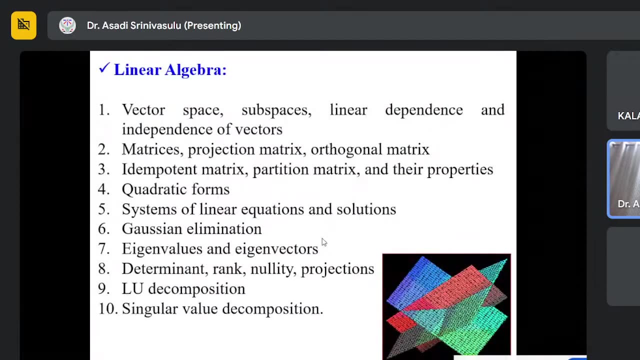 Various operations we are using And various testing methods we are using, like z-test, t-test, psi-square test, etc. In order to check our model is correctly classified or not, And various statistical methods like linear, non-linear logistic regressions, we are using. 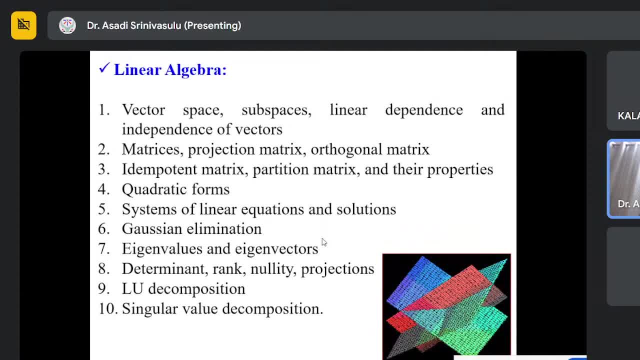 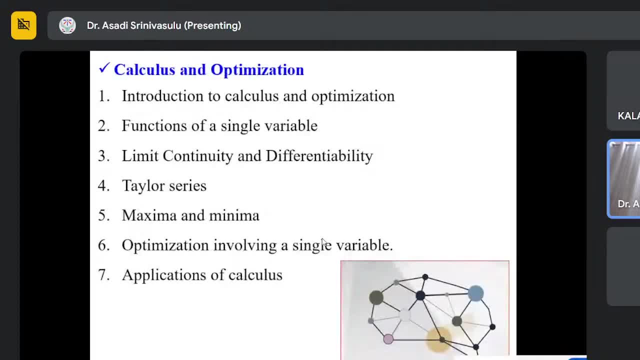 In linear algebra we are using Lagrange's method and matrices And various quadratic forms. We are using Then calculus and optimization. We are using Taylor series, maxima and minima And functional of a single variable, Limit and continuity and differentiability. we are using 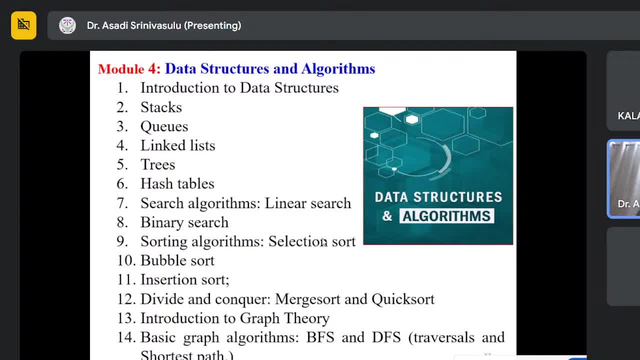 Then followed by the data structures and algorithms. So, data structure approaches: we are using four approaches, like divide and conquer approach And dynamic programming, greedy method, branch and bound. Here we are using sorting, searching, various algorithms. we are using A systematic way of organizing data, representing data and accessing the data and storing the data in the fashion of linear fashion, in the fashion of non-linear fashion. 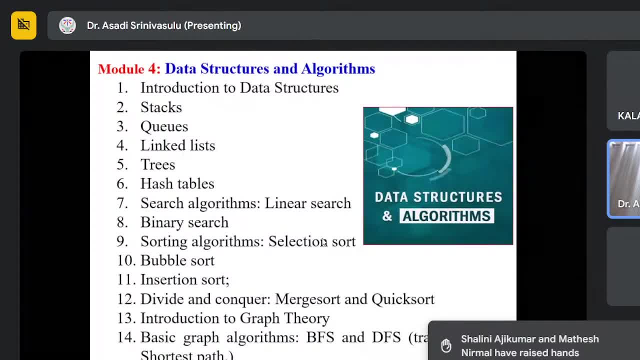 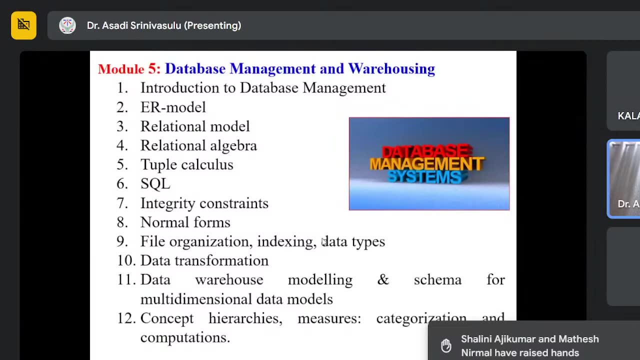 Like linear fashion. we are using arrays, stacks, queues, linked list, etc. Non-linear data structures like trees and graphs, etc. So this is about data structures and algorithms, Database management and warehousing, Collection of interrelated data, And we are using storage of a huge volume of data in the servers and data centers. 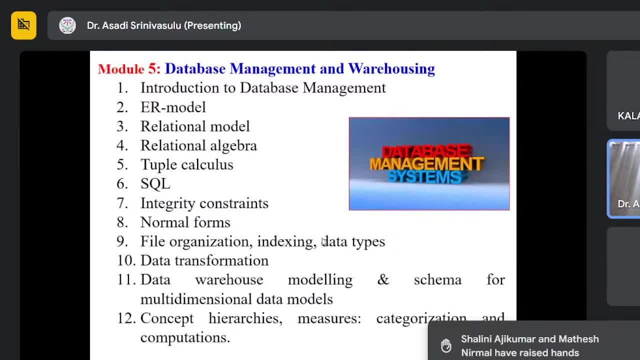 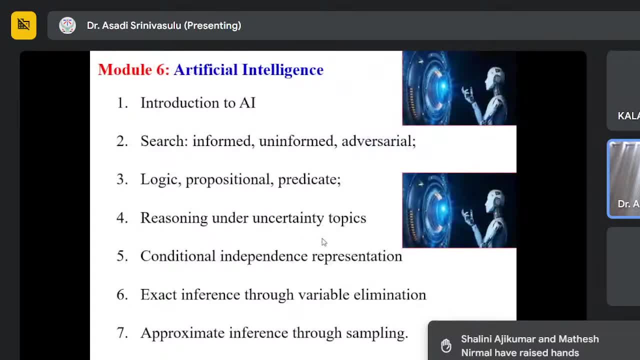 We are using AR model SQL And no SQL databases. we are using Like Hive, HBase, Zookeeper, Scoop, etc. Then artificial intelligence: Intelligent behavior in a machine That is called robot Robots, humanoid robots like Cosimo Sophia. 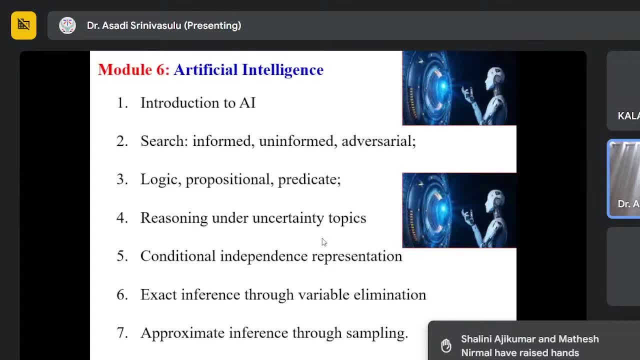 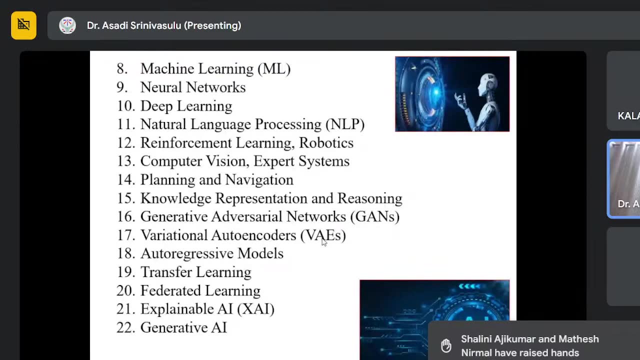 Sophia recently took the citizenship of Saudi Arabia. Here I am going to explain logic and propositional predicates: reasoning under uncertainty. topics: A-star algorithm, approximate inference through sampling and machine learning, neural networks, deep learning and GANs. generative adversarial networks. 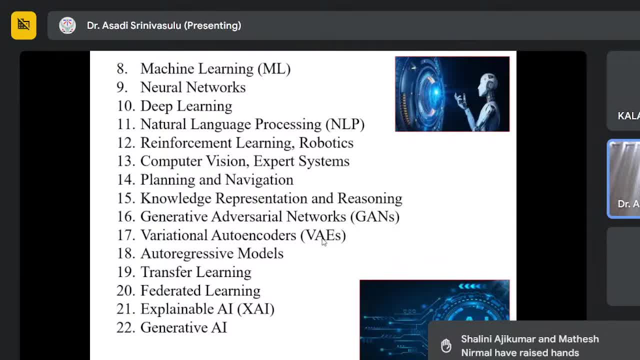 I would like to mention one small interesting story. Recently, Japan, one of the scientists has released his facial expression over the period Like baby One year, baby Five years, Ten years, Fifteen, Twenty, Thirty, Thirty, Thirty-five years. 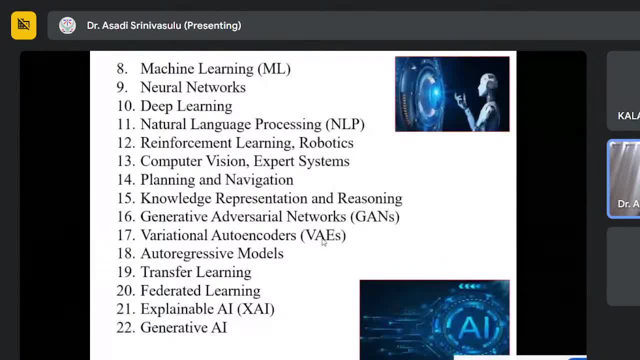 How our face, over the period, changes. Facial expressions: How do we become in the old age? So such type of facial expressions app developed Japan scientists by using generative adversarial networks, GANs, My dear friends, keep in mind. 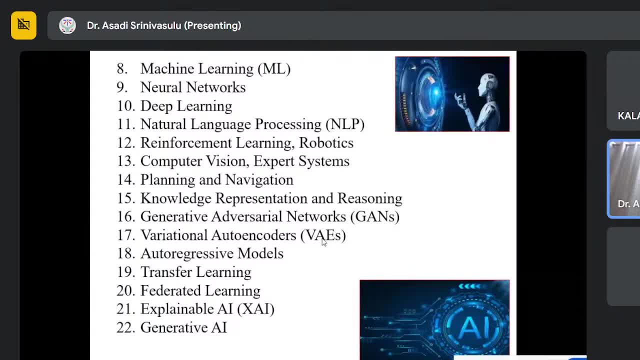 GANs are powerful technique in order to develop facial recognition, Facial expressions, facial emotions, such kind of applications, video, audio applications. in order to develop, by using GANs, networks, then a variational autoencoders, transfer learning, federated learning, explainable AI, generative AI. 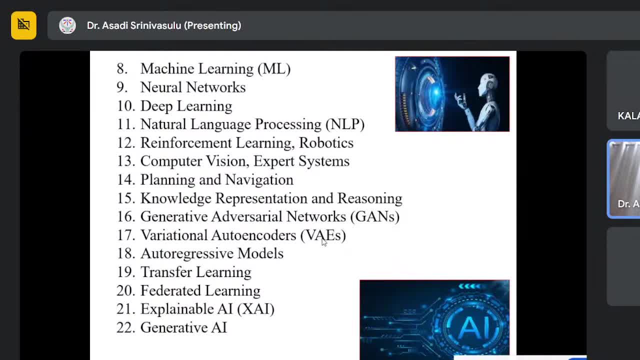 See. recently I have started corporate training on generative AI. Here I am going to explain various new concepts like explainable AI, federated learning, transfer learning And machine learning, deep learning by default, generative adversarial networks and variational autoencoders. 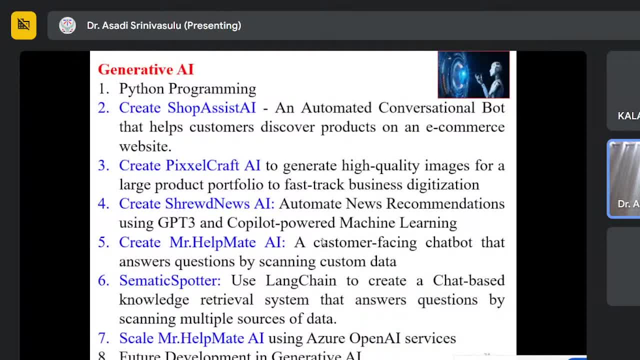 And auto-regressive models we are using. This is a corporate training syllabus, So by using Python programming I am developing various generative AI applications like create shop assistant AI. create pixel craft AI, create shred news AI, create Mr. 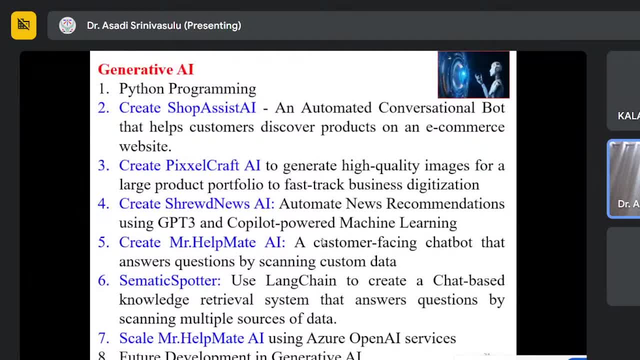 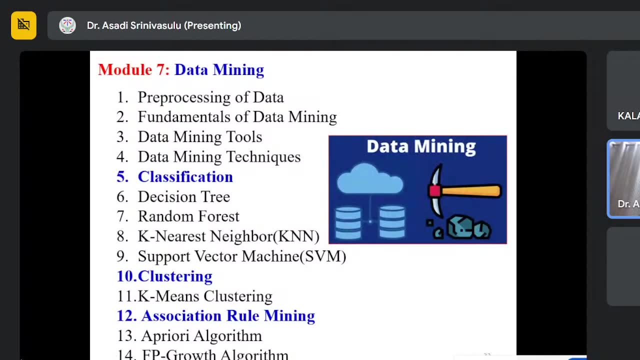 Helpmate AI semantics portal scale. Mr helpmate, ai further development in generate ui. whatever the new applications, if you want to develop by using python programming, we are, i'm developing. so then data mining: the data mining is the process of extracting meaningful interested patterns by applying classification. 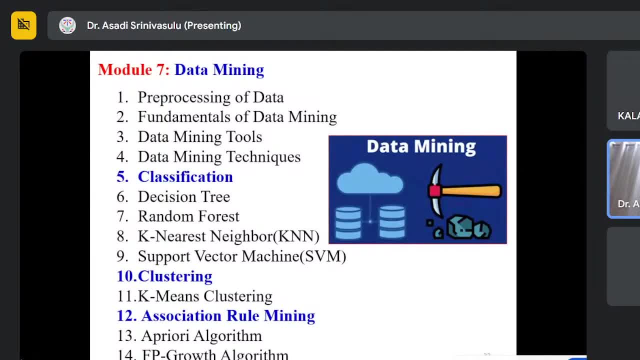 clustering, association rule mining, outlier detection. in classification we are using decision tree, random forest k, nearest neighbor, support vector machine, neural networks and etc. in clustering we are using k means clustering, c means clustering, fuzzy c means clustering, agglomerator clustering, density based clustering, etc. in association rule mining i would 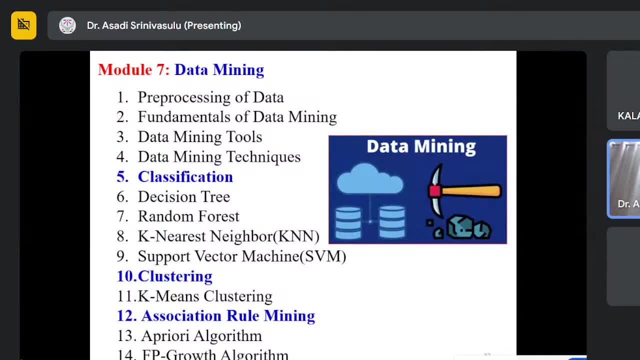 like to give you a small story. han and kambar: they have developed one textbook called data warehousing and data mining. so, han and kambar, they are the uh, they are uh, they are pursuing their master's and phd at stanford university. they have collected. 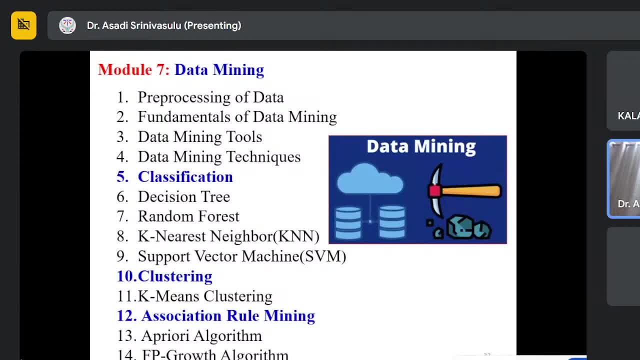 10 years old legacy data and kept in the server and they applied association rule mining techniques like apriori algorithm and fp growth algorithm in order to find out frequent pattern items. so here is a small story. uh, us people- usually they are outing with their family and children. 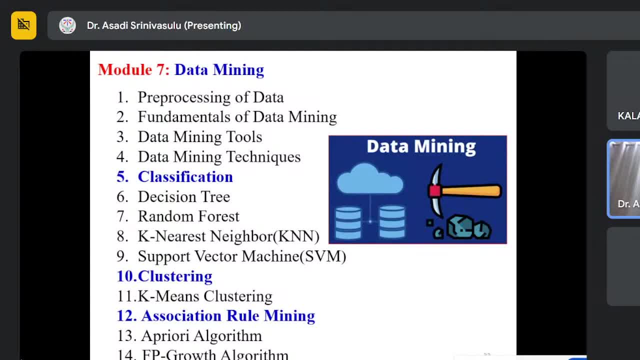 and every certain time, they are outing with their family and children and they are outing with their. and every certain time, they are outing with their family and children and every certain time, they are going out with other children, uh, and their family has different relationships, like, remember that they use to reach products, uh, which they did on saturday and sunday. what are the items they use to? 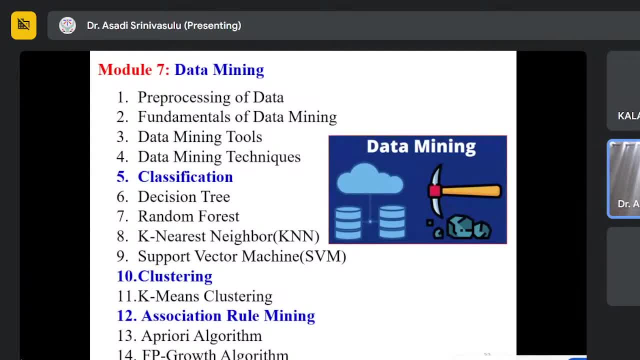 purchase in the walmart and they are enjoying uh saturday and sunday with their family members. so 10 years data they have collected, han and kumber. they kept in the server. they have applied pre-processing techniques like box plot beginning techniques. after that they have applied association rule mining technique like apriori and freep growth. surprisingly, 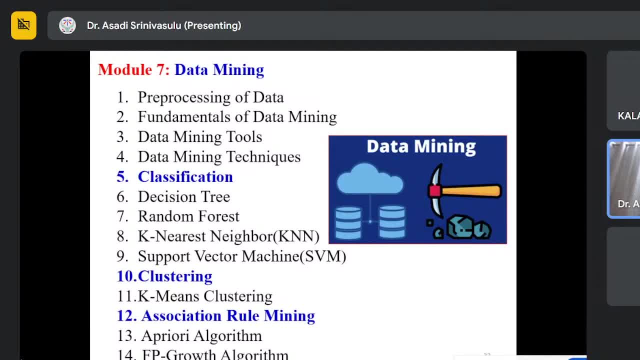 two items are heavily sold out. can anyone give answer? what are the two items are heavily sold out? you? can you, canaman, give answer? what are the two items are heavily sold out? so you can give us your answer. basically, get started. so the first item i am going to tell you they are normally sold. both rhyme, andresite and scenario work is by: 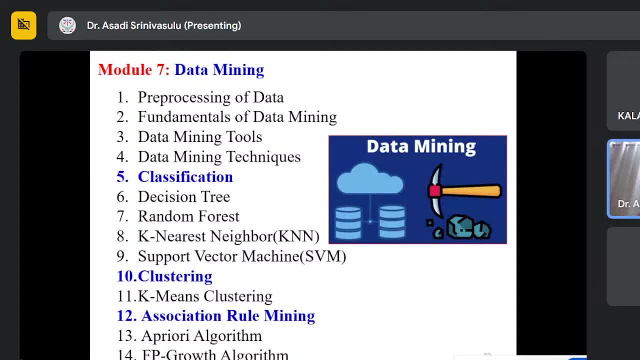 the two items are heavily sold out in the Walmarts. Any answer from chart box. I would like to see Anyone. Bread and butter is in the top 10. association rule mining: Yeah, your answer is correct, but not correct. accurate answer What I am expecting from the 10 years. 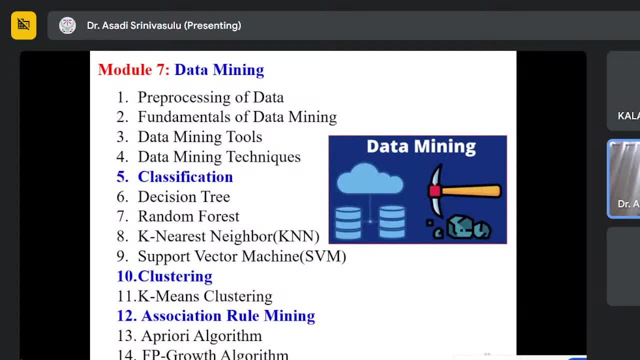 legacy data- they have applied Apriori- and FP growth algorithm. Surprisingly, they found two hidden patterns, two interested items from the 10 years old legacy data. Can anyone answer, Madam? what is your name? You have given wonderful answer, but not correct Is. 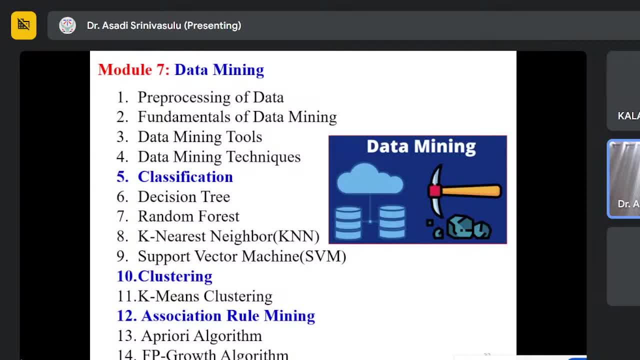 there any other faculty members, please? What is your answer? Milk, Milk And combination Chocolate combination. So milk and chocolate. No, sir, It is a completely wrong answer. sir, I am expecting association rule mining frequent item sets in the Walmart. 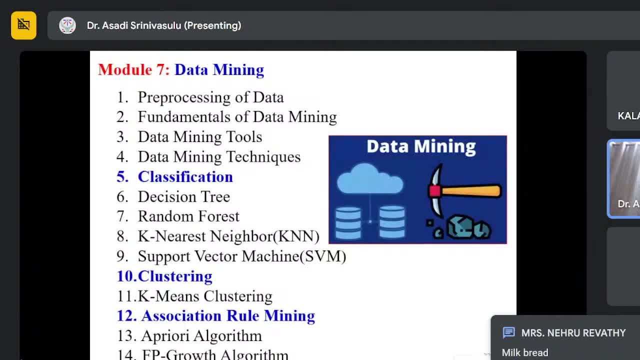 Two items- I am mentioning clearly two items- are heavily sold out within the 10 years legacy data. Can anyone answer? Try, Sir, you tried. very well, sir, I am appreciating you. Milk and chocolate. Milk and bread. Maybe that one of the one more best association rule. one more, Madam. 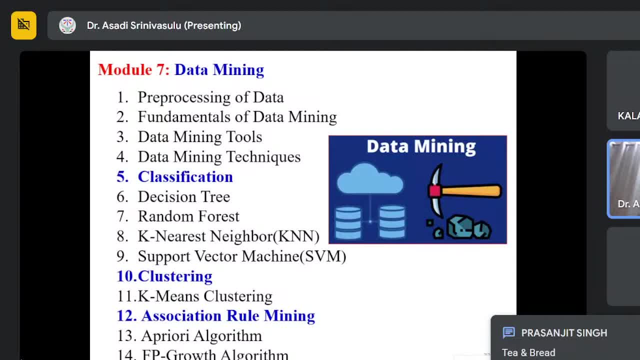 told bread and junk. That is one more association rule: Baby wipes, sir, Baby wipes, Baby Wipes and diapers, Oh, diapers. Then what is the combination? One answer you have given: Wipes, wipes, wipes. No, My dear friend, what is your name, Dr Barani? sir Barani, congratulations. 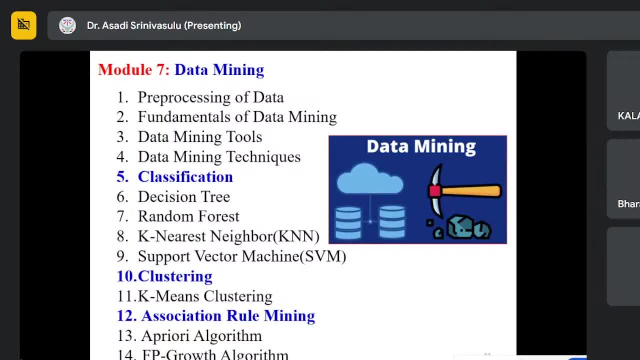 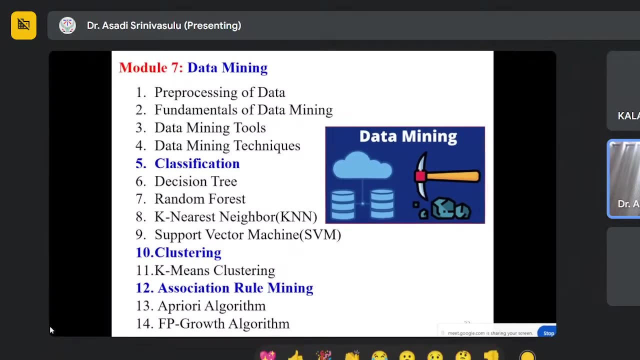 Only 50%. 50% answer is correct. Can you try for 50% combination? frequent item set: Wonderful answer. Wonderful answer. Barani, try. Diaper is correct answer. Fantastic, Give him big round of applause And one more answer. Can anyone please try? 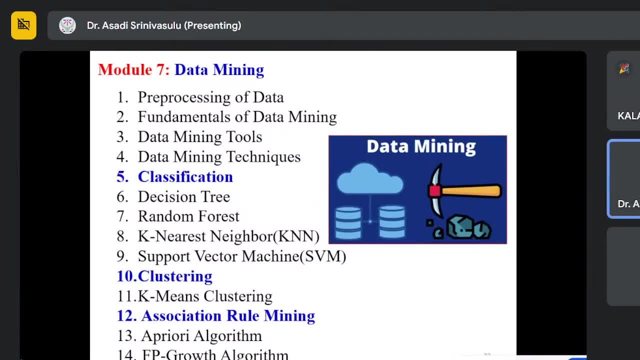 Strawberry, Strawberry. No, madam, Absolutely wrong answer. madam, Sorry to say you. Can anyone try Diaper is correct answer. I have given 50%. What about remaining 50% Can anyone? Frequent items means two items. 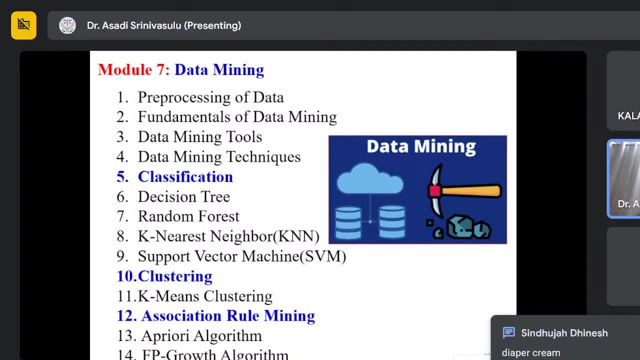 only Heavily sold out within 10 years. legacy data- Can anyone? Very interesting. I am going to demonstrate this application by using Aprior and FP growth algorithm. now I will start immediately after explanation of my syllabus. Directly I am going to demonstrate. Can anyone? 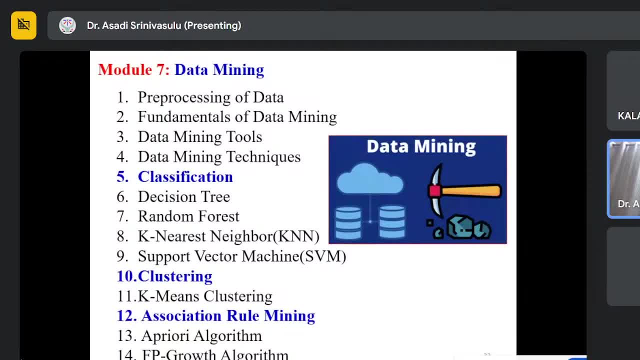 give answer Please. If you don't know, can I give the answer Please, My dear faculty members, Any guess, Any guess? Oh, sorry, Sorry to say you. So, Diaper Barani, I am giving one goodie one. 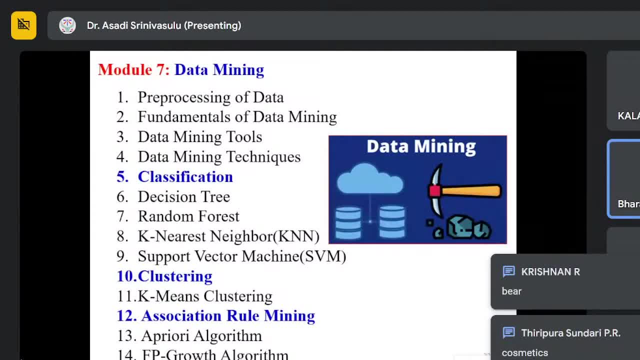 chocolate for you. Thank you, sir, Thank you very much. Yeah, Diaper and beer is the combination, Hidden patterns. even now the scientists are surprised What a combination this one. Usually US people are outing with their family. They are picking one diaper, one beer, Like that combination. See Surprising item That's. 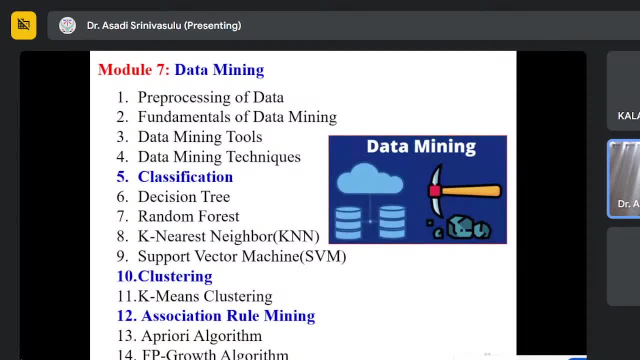 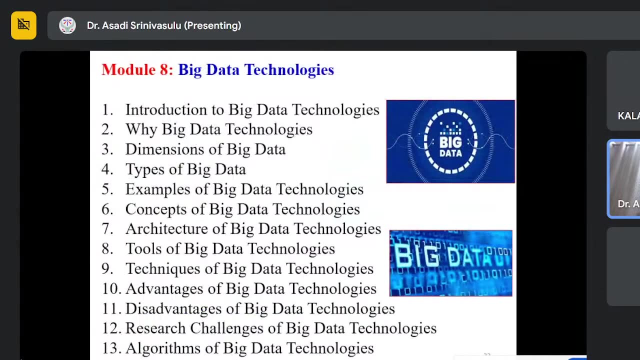 why we are studying data mining. Data mining is the process of extracting meaningful, interested insights and interested analytics. we are generating with the help of association rule mining, like Aprior and FP growth algorithms. Then big data: I have explained already So which data we can call it as big data. Traditional. 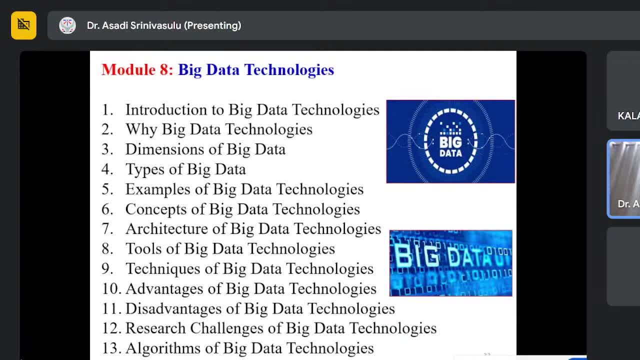 systems are unable to process. the big data is called big data. Maybe terabytes, petabytes, exabytes, octabytes, yottabytes, zettabytes, brontobytes and geobytes, I don't know. That's why we are going for high computing, high computing frameworks like Hadoop and Spark. 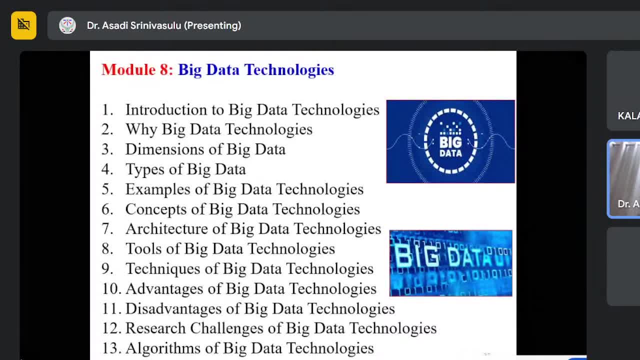 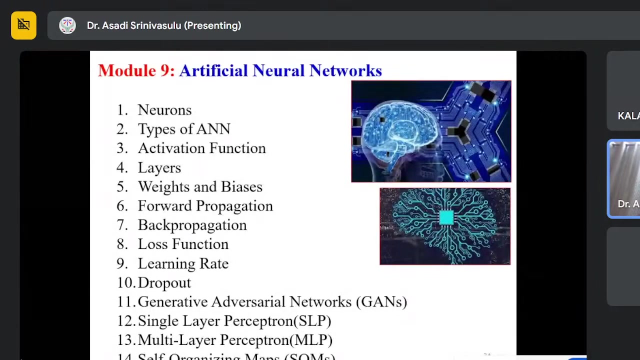 and and and, Matlab, Hive, HBase, Zookeeper- Various tools we are using in order to process the huge volume of data. What are the dimensions of big data? Volume, velocity, variety, veracity. There are seven more. Vs are also presented like value, validity, viscosity and variability, etc. Types of big data. We have three types of big data: Structured data, unstructured data, semi-structured data. 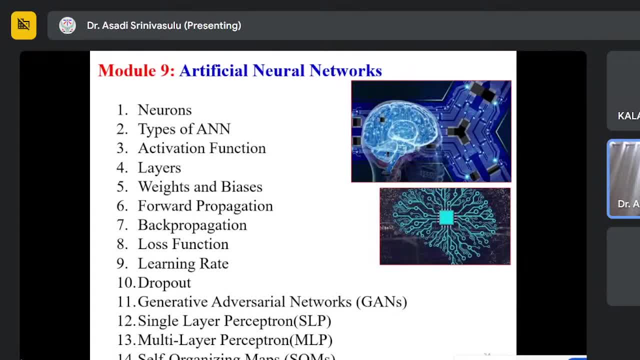 Structured data means with the help of relational database tools. There is a schema, there is a table, there is a relation. we are creating the tables with help of SQL, MySQL, Terra, data depri to MSS access. That is called structured data. So there is no. 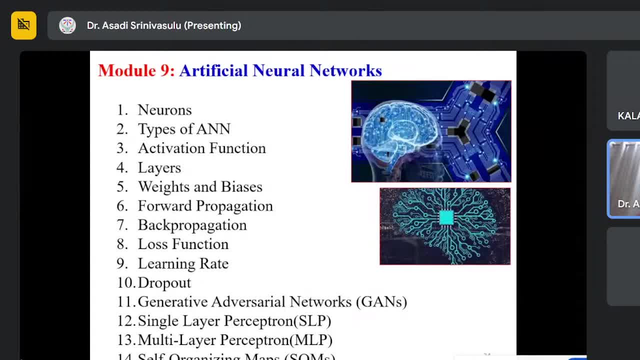 label. there is no, I mean there is no schema, there is no relation, there is no, there is no anything. but we are creating the tables, shake, creating the database with help of NoSQL databases such as Mongo database, Hive database, HBase. 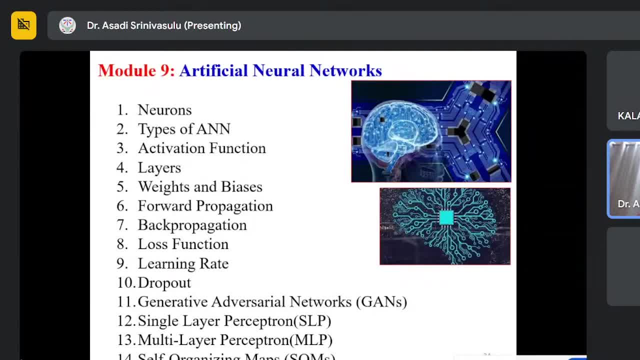 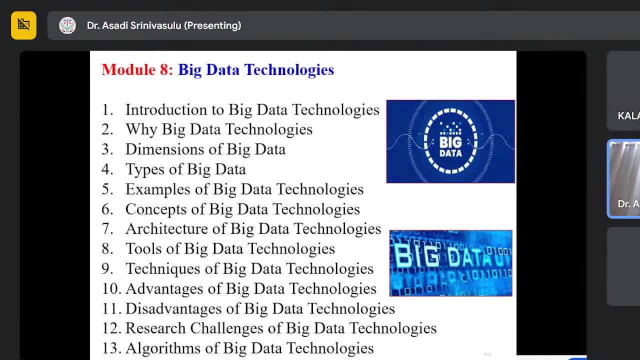 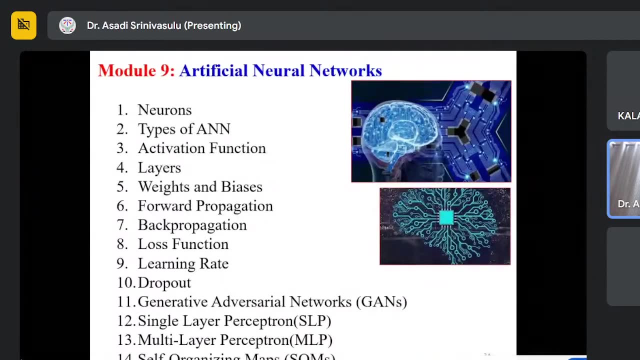 database, Zookeeper, Scoop, etc. okay, So, and there are various concepts we are using in this big data technologies, tools and techniques and various algorithms we are using. then artificial neural networks. So neuron is a biological expression in the biological pattern we are creating artificial. 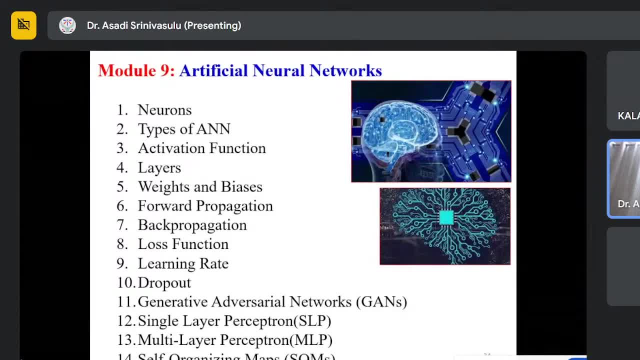 neural network with help of input and hidden layers. we have various activation functions and learning rate and dropout, and layers like weights and biases, generative adversarial networks, SLP, single layer, perceptron, multilayer perceptron, self-organizing maps, etc. 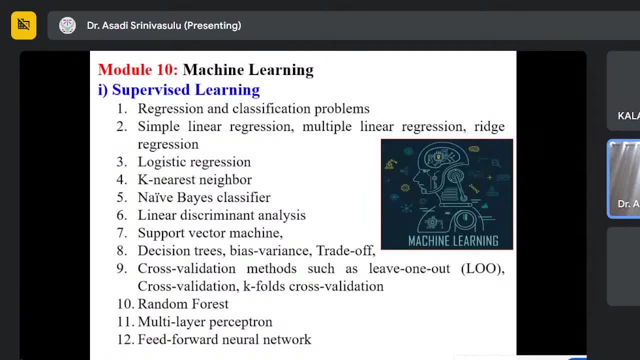 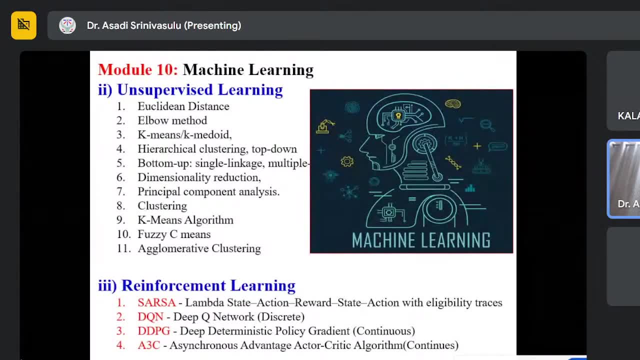 So then, machine learning, There are three approaches, like supervised learning, we have n number of techniques. I have explained already. Unsupervised learning, we have various techniques like agglomerative Fudgy, C means, K means, etc. In reinforcement learning, I have explained, based on the punishment and reward we are 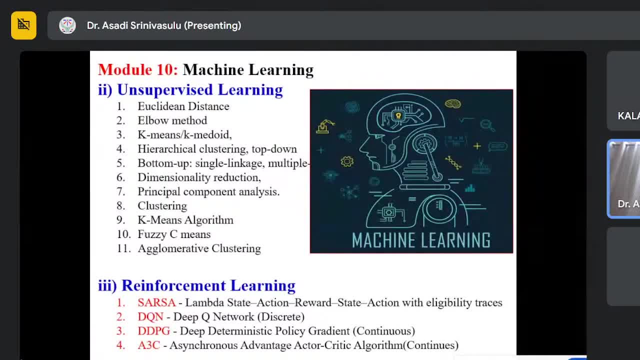 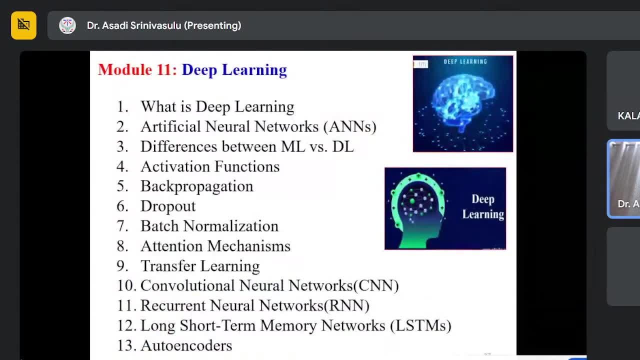 solving the problems, like by using a SARSA, DQN, DDPG, A3C. these are the gaming algorithms in order to develop your own game. you can use it. Then deep learning, Learning from the observational data with the help of a huge number of input and hidden. 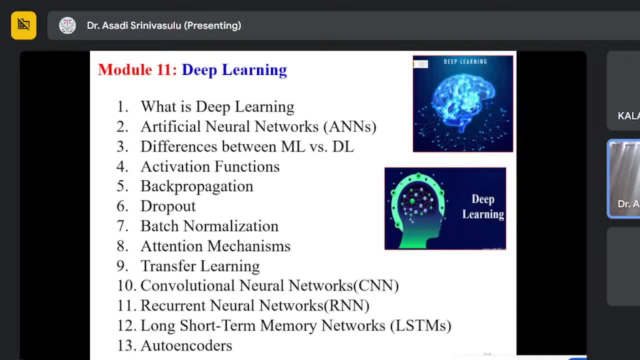 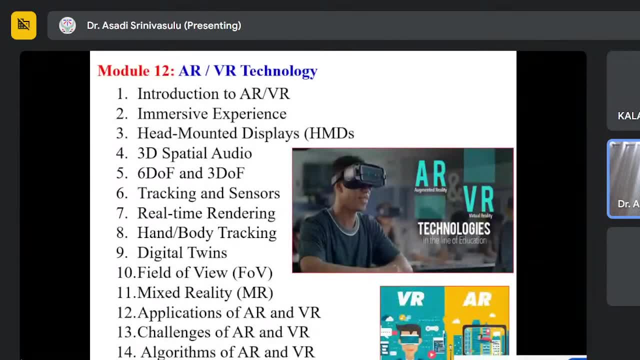 layers like ANN, CNN, RNN, LSTM and auto encoders, etc. Then augmented reality, virtual reality. we have various tools like head mount display, HMD and digital twins, real-time rendering and we have a mixed reality also, field of 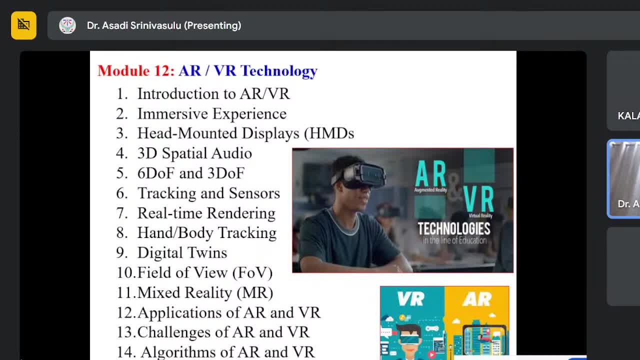 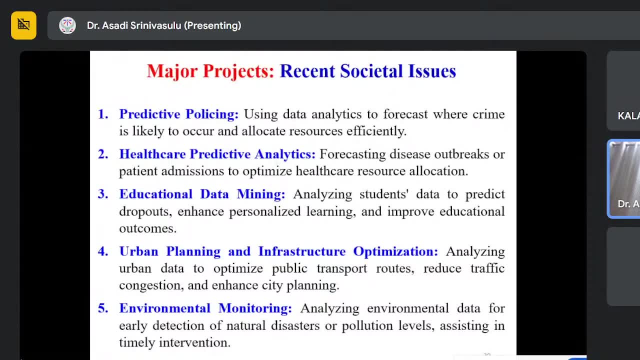 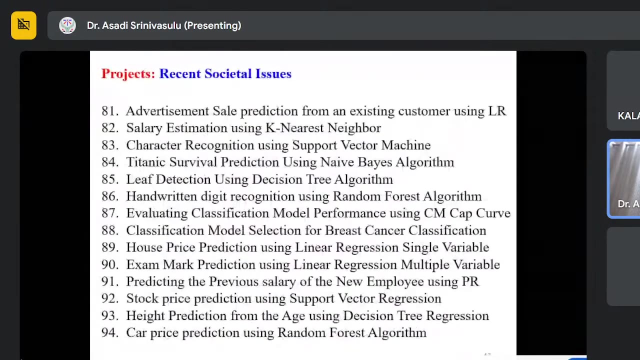 view, Various concepts in the case of audio video we are developing. So these are the various projects I have developed in my research laboratory and GSER. and GSER is the research laboratory at the University of Newcastle in my research laboratory. So these are the 150 projects I have demonstrated under data science research laboratory. 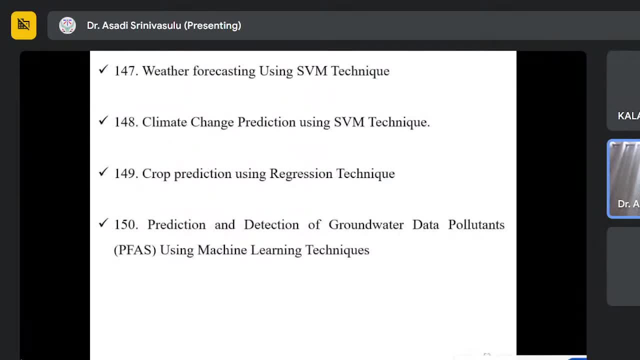 These are the 150.. Prediction and detection of ground work. So these are the 150 projects I have demonstrated under data science research laboratory. So this is the 50 which I will be talking about. This is the most recent project proposal I am implementing, like prediction and detection. 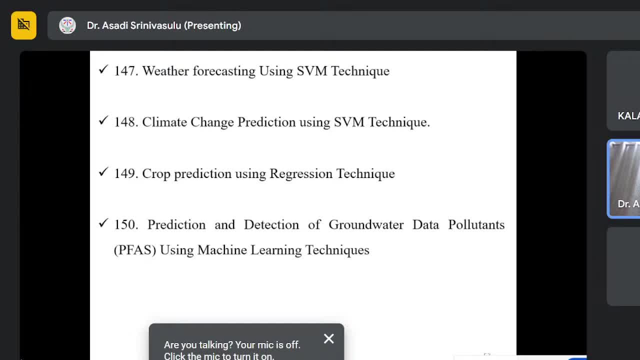 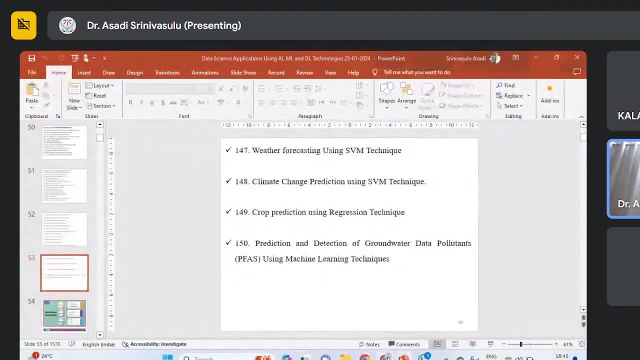 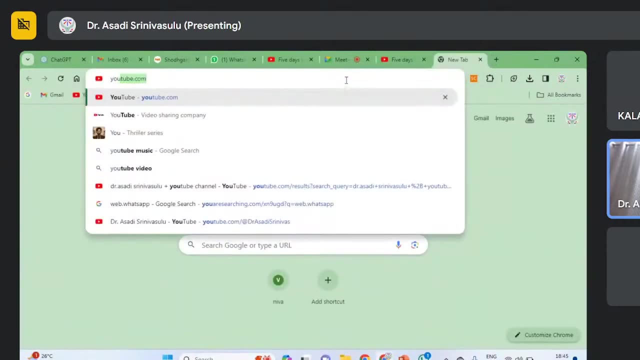 of groundwater data pollutants, that is called PFS, using machine learning and deep learning techniques. Okay, so how many of you know and see? if you want to see my videos, my dear friends, just please go to YouTube. I have explained in. nearly 253 videos are presented. 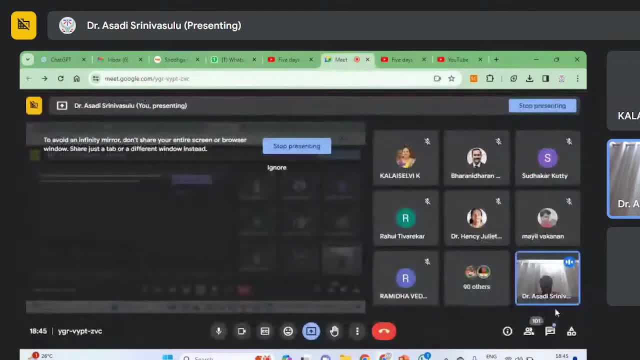 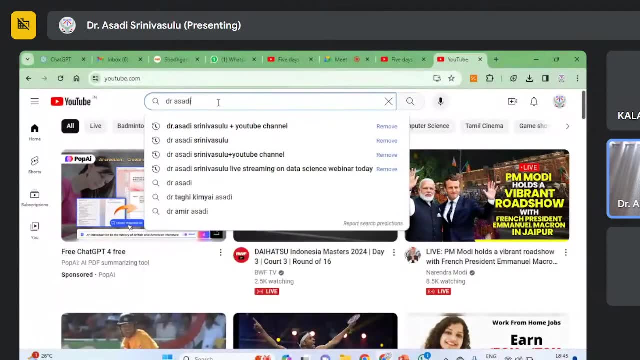 Yeah, here. How many members are there right now? 101.. Please open YouTube. So you type Dr Asadi, Please. if you are in mobile also, please type. just go to YouTube. Dr Asadi Srinivaslu. You can type. 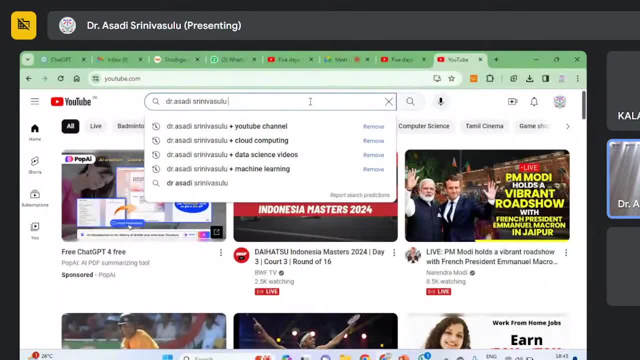 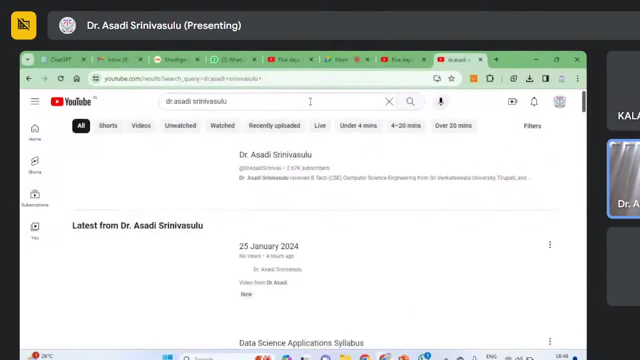 just Dr Asadi Srinivaslu. A, S, A, D. I Please type S, R, I, N, I V A S U L U. Please type just Dr Asadi Srinivaslu. After that press, just go to Dr Asadi Srinivaslu. See how many videos. 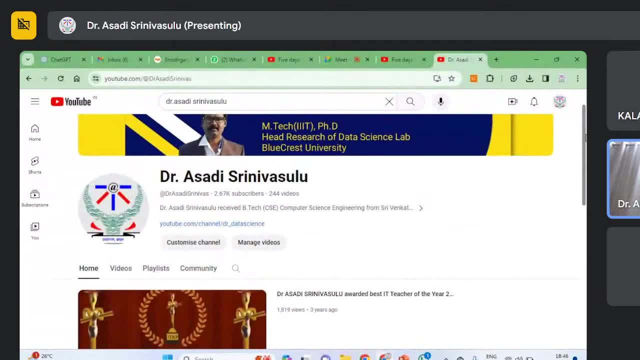 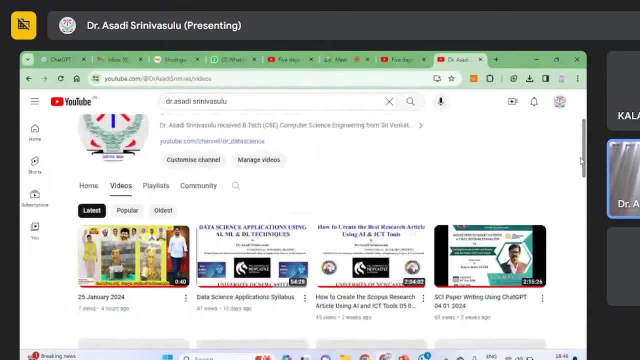 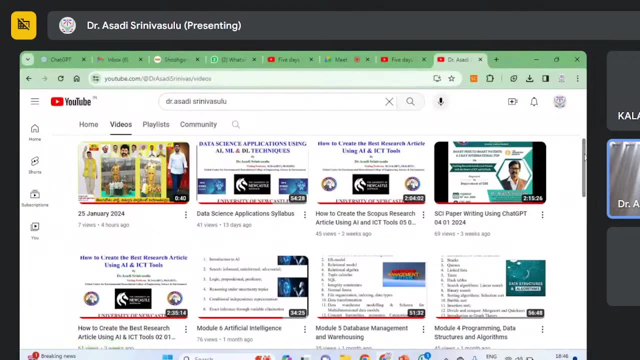 I have created. 244 videos are there. If you see all my videos- different technologies- I have explained. Please subscribe my channel and you can write your own comments. Take one minute time. How many videos are there? Please see here? Nearly 244 on various technologies. 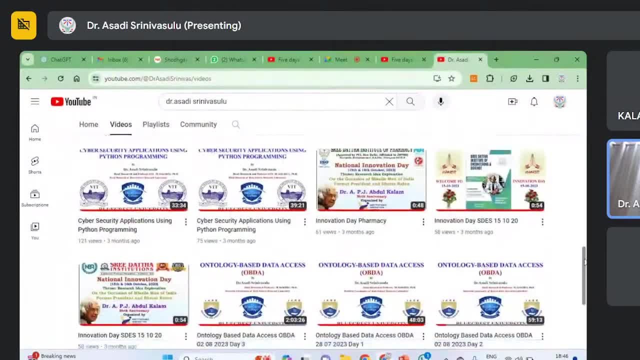 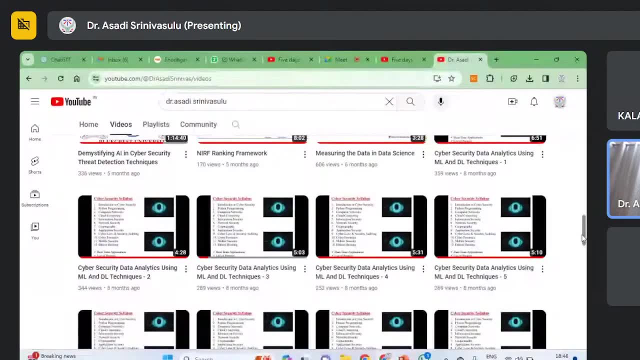 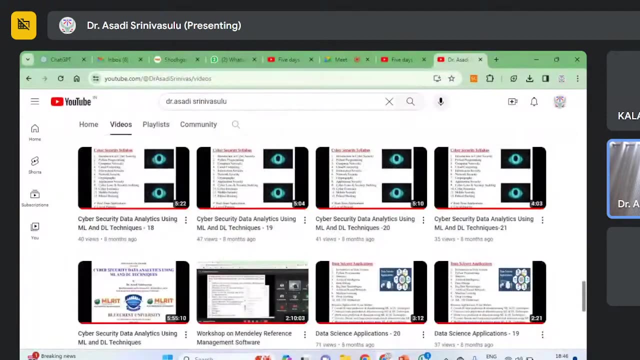 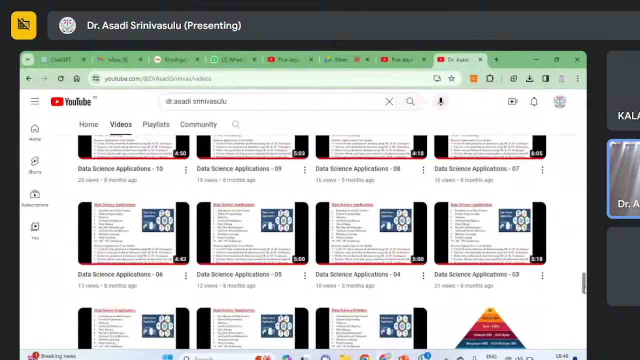 Technologies like data science, big data, artificial intelligence, ontology based and see- and cyber security. How many videos I have created for corporate training? actually, Cyber security and data science and machine learning, deep learning, internet of things, blockchain technology- See. here are the various videos. You can find the 244.. 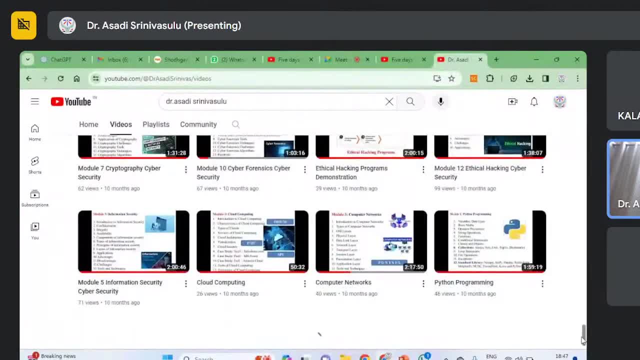 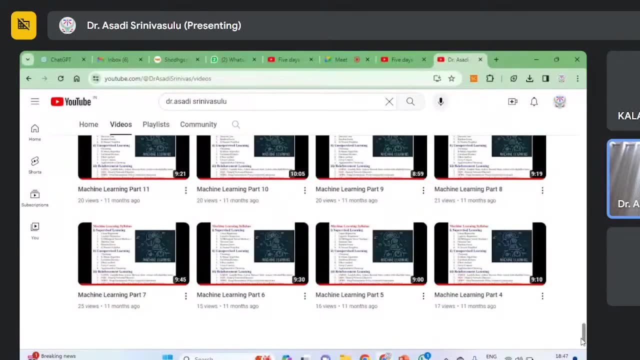 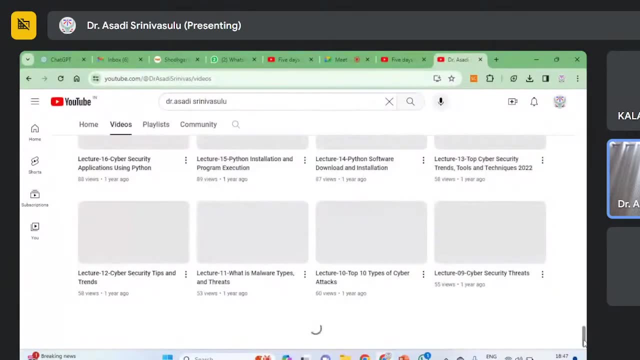 Videos: ethical hacking program demonstration and see cloud computing and here are machine learning, deep learning. These are all are my videos. Please subscribe and whenever you find the time, please, you can listen my videos and you can write comments on that. my videos. 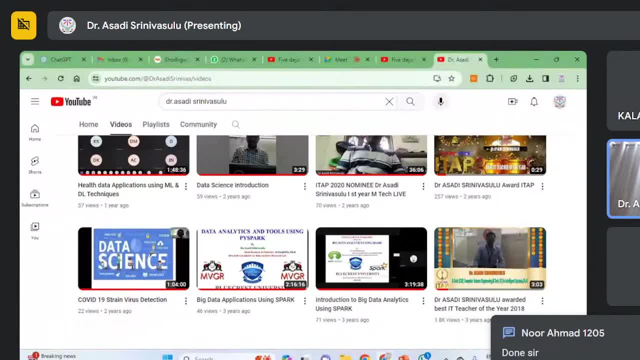 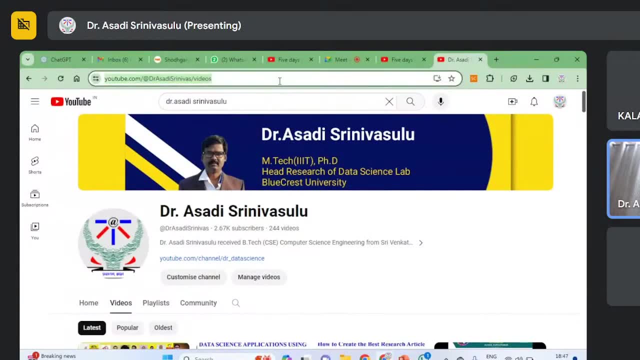 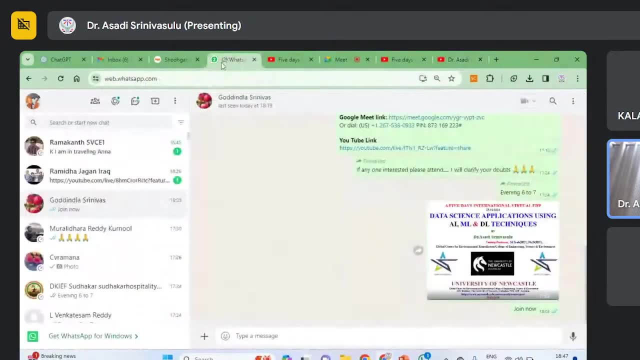 So now I am going to demonstrate all the practical sessions Now see, because of time. So how many of you subscribed, sir? Only 10 members are so far. Number not increase here. Please subscribe. At least subscribe one minute, sir, It is showing. 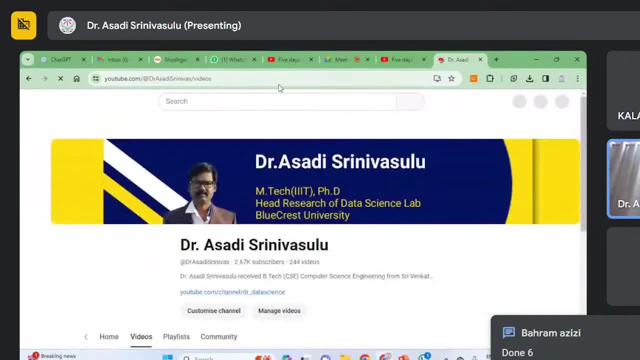 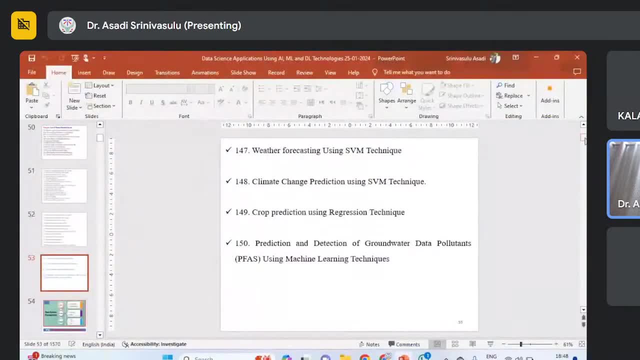 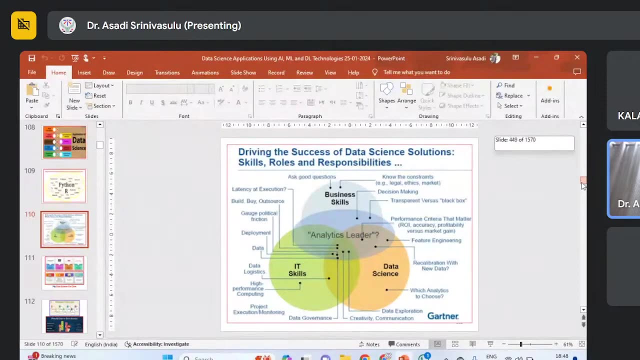 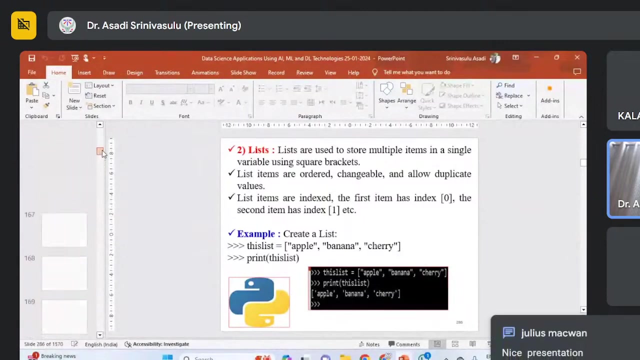 now 12 members. Now, only 12 members, sir. See, now I am demonstrating practical session on data science applications. These all are theory sessions. You may get bored. That's why I am going to demonstrate practical session now. Okay, So I am going to demonstrate practical. 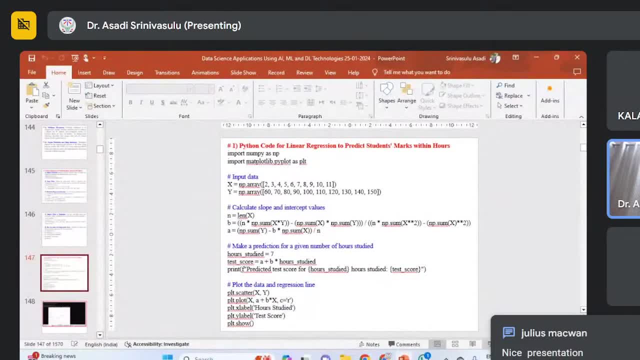 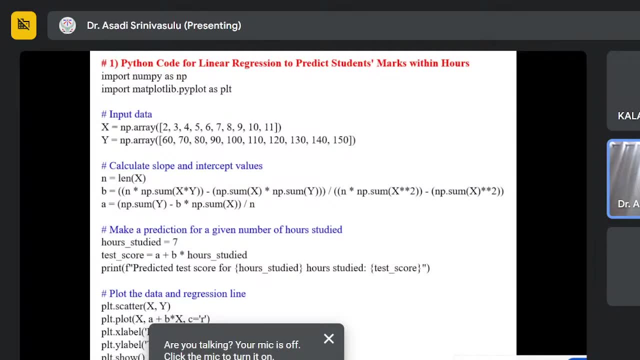 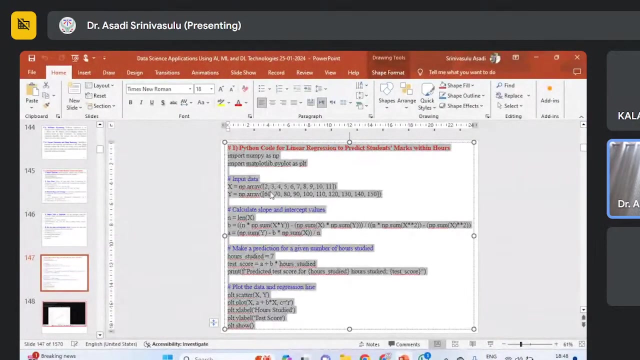 session now. See Python code. See here Python code. Linear regression to predict the student marks. Small application: How to develop, Please, sir. See, I am going to demonstrate this one. Okay, If you are having Python programming, you can directly, you can execute. Otherwise, see just control C. So go to CMD Once you have. 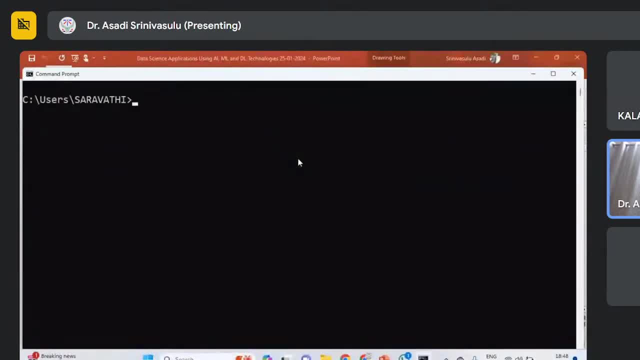 installed Python. check whether Python is there. My screen is visible, madam. Please. Can anyone? Yes, sir, Yes, sir, Yes, sir. 3.12.0 version I am using, So here also see. Python can be executed in two ways. 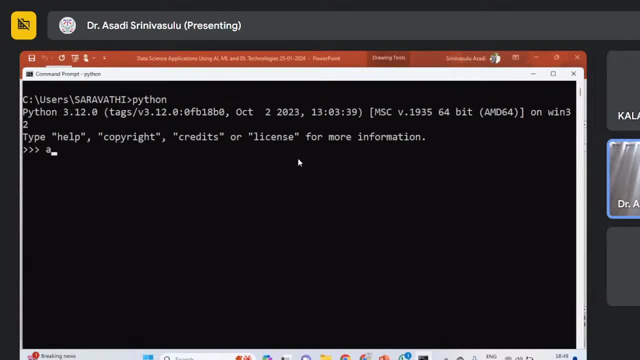 This is ideally integration development learning environment. a is equal to 3. you can check the A value. b is equal to 4. you can check the b value. Then c is equal to A plus B. you can check the c value. 4.3 is 7.. So this is simple manner to execute Python programming. 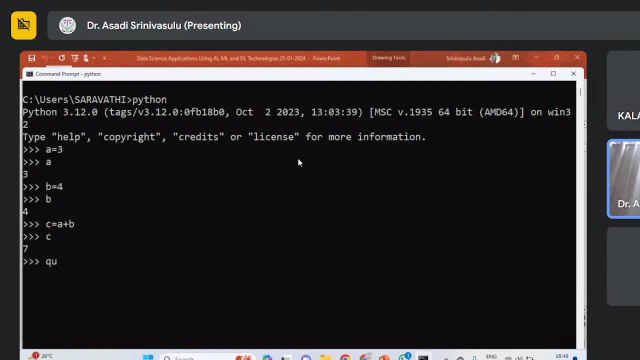 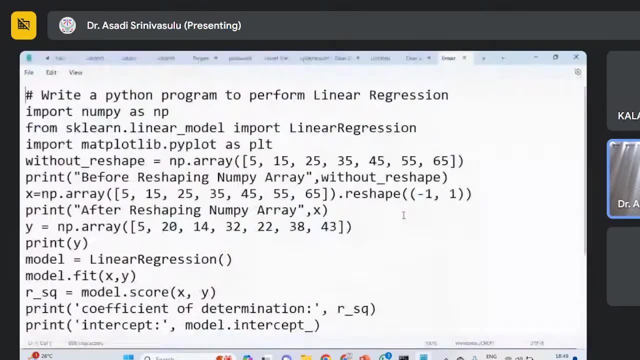 This is one more. This is one way. and one more way is scripting way. So scripting way, you can write your own script: notepad space, So linear. see, I have created already linear dot. this is the program I have created. write a Python program to perform linear regression. Okay, so I'm executing right now. 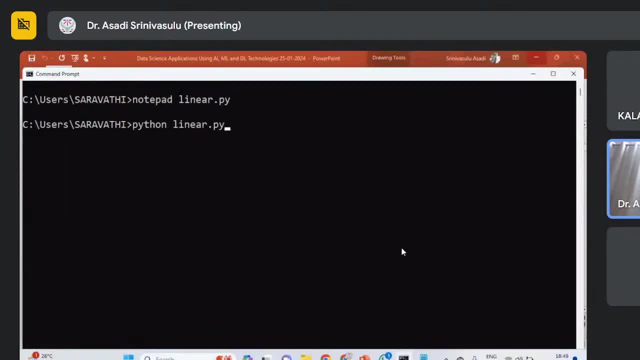 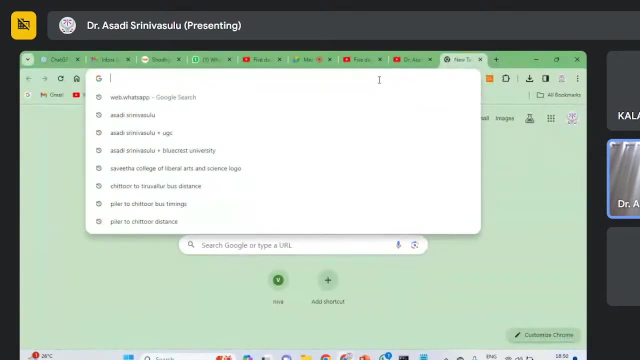 Python space linear dot py. So now see, because of see libraries and I need to install libraries, then only it can execute. That's why now I'm going for Google collab. See, if you, if you are, if you are having a in your system, you can execute. Otherwise, directly you can go to. 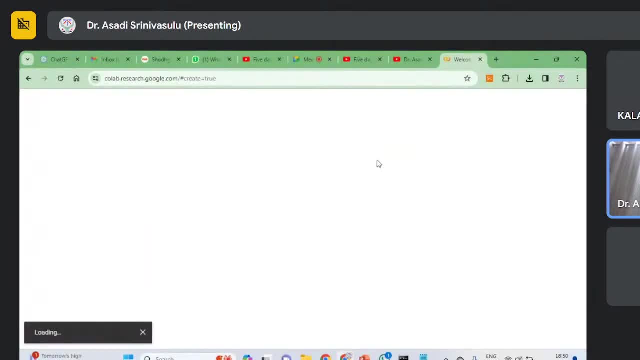 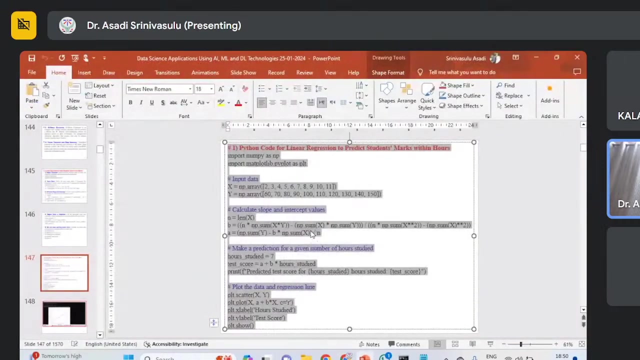 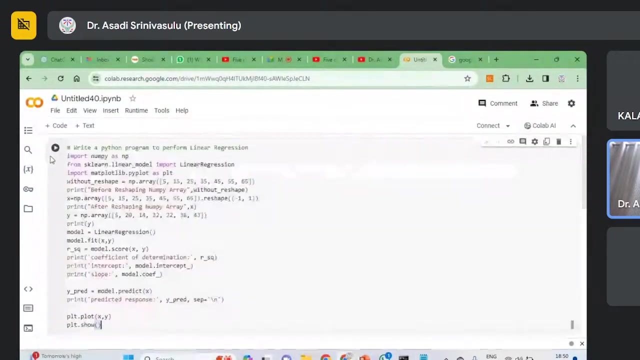 Google collaboratory. it is a execute in executed environment where you can execute your all Python program. See now I'm I'm executing here, just I'm copying this code. And see now I'm copying. See now I'm executing here. Now it is running. See left as my screen. 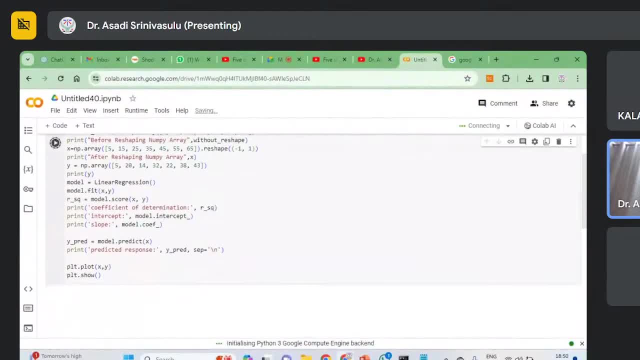 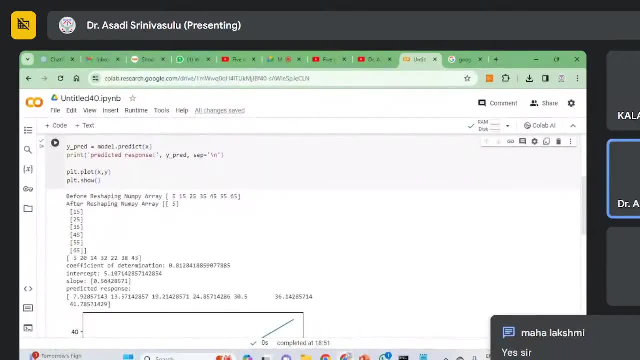 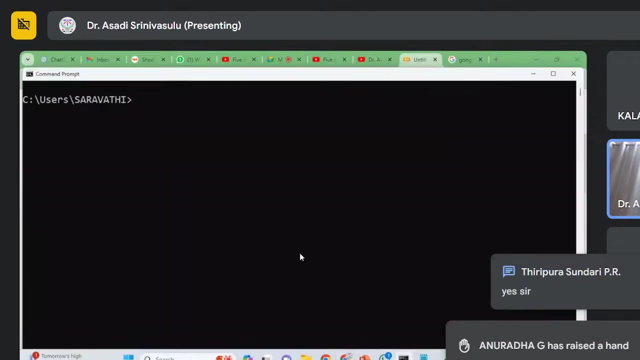 is visible, madam. Yes, yes, Yes, it's very visible. Yeah, it is visible. Yeah, now it is running. It is going to see now. see, now it is it produce results graph. Are you seeing my graph? Yes, sir, Yes, First program. next second program: see. go to notepad space linear. 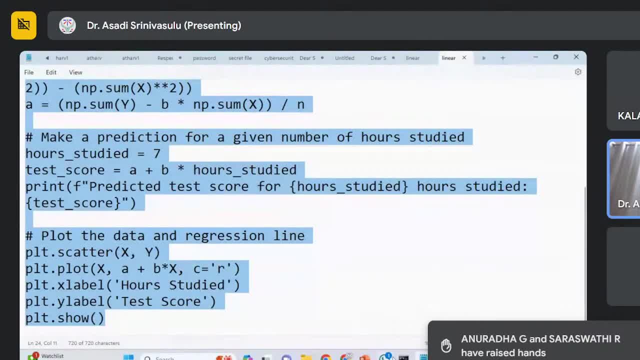 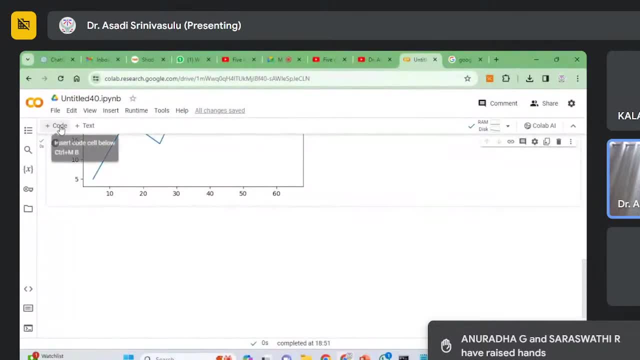 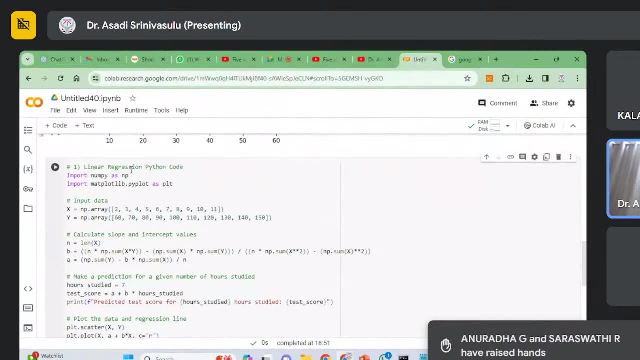 one. So this is one more program. student program. Now, see, I'm going to execute. So here I'm pasting: see, See, now here I'm pasting. second program: write a Python program to perform student marks. See, here I'm taking student marks like two hours. if student student reads 60 marks you will get. 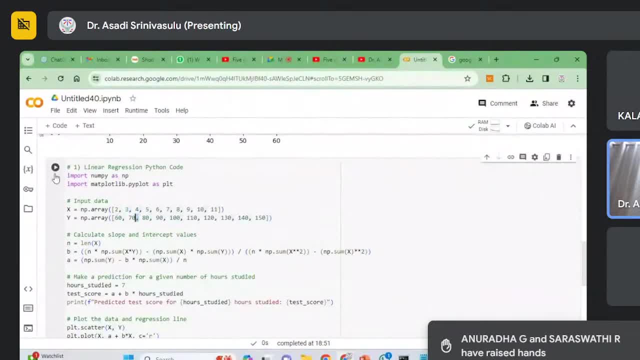 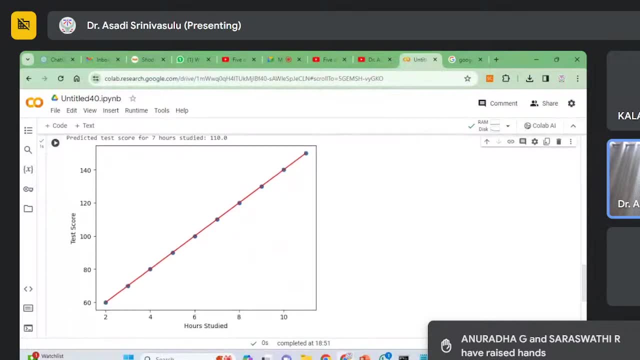 three hours read 70 marks like that. So by using linear regression, how to execute now? see now my program is running. See now, please check here. So here, seven hours, if you are studying, you are getting 100%. see here my screen is visible, sir. 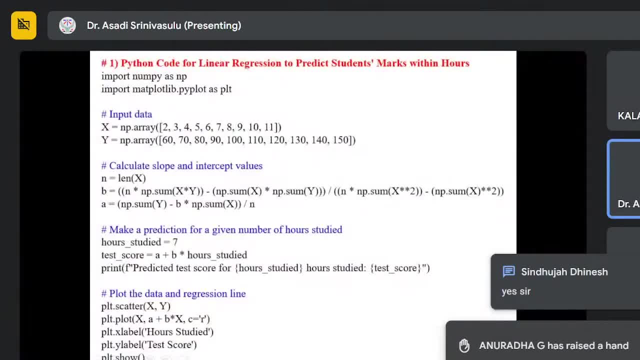 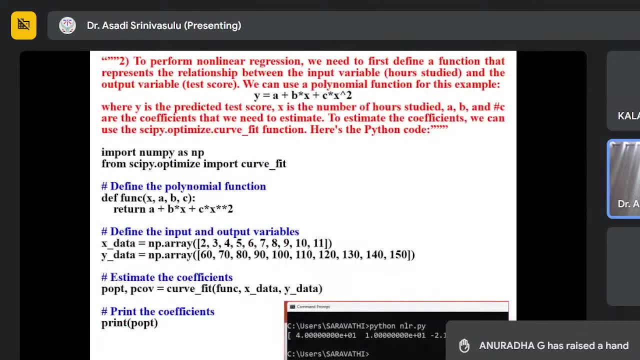 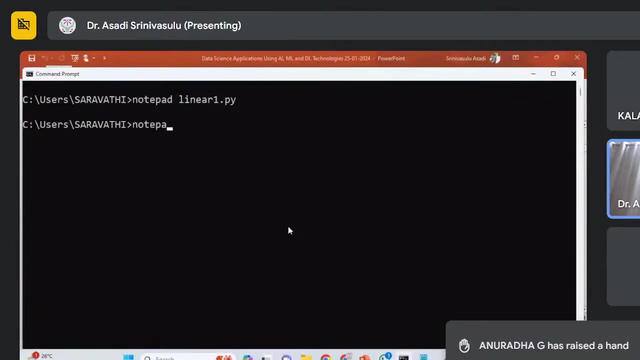 Yes, sir, Yes, sir, Yes, sir, Yeah. So now this is the first program, then a nonlinear regression. If you see nonlinear regression for same application, how to? we are going to execute now. see nonlinear regression Here. go to notepad space. I have already created. Okay, nonlinear. 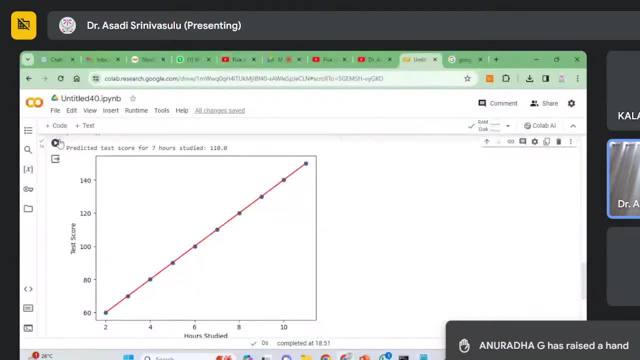 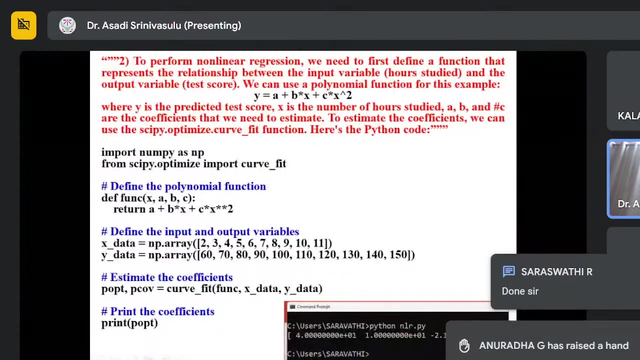 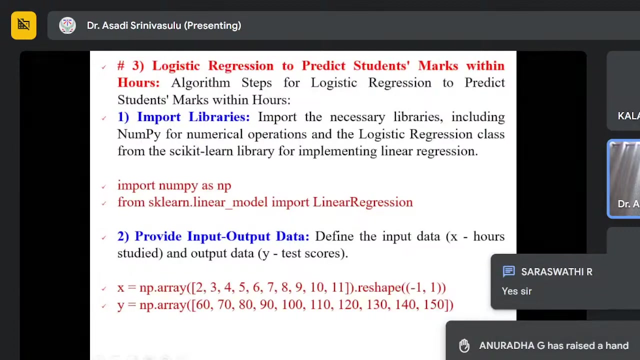 So this is the program. now code: Google Collaboratory. go to Google Collaboratory, now run. So here see, now this is the output. I got it. So nonlinear regression. then go to next logistic regression. See brighter Python program to predict the students marks within hours. So same two hours: 60 months. 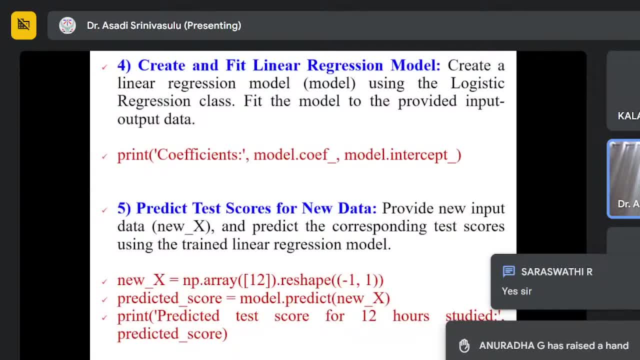 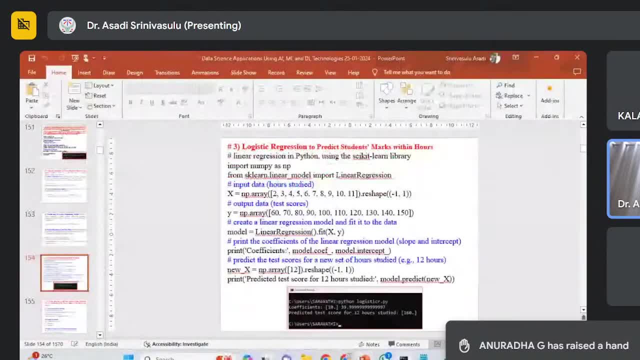 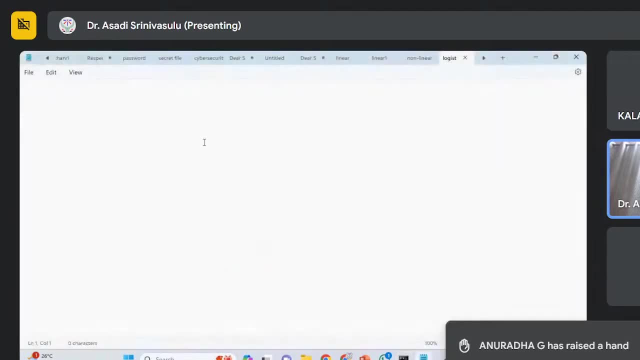 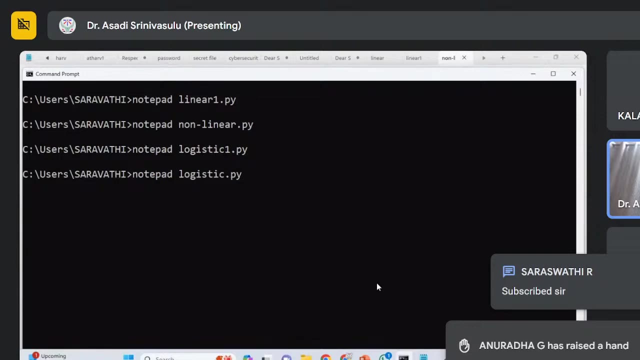 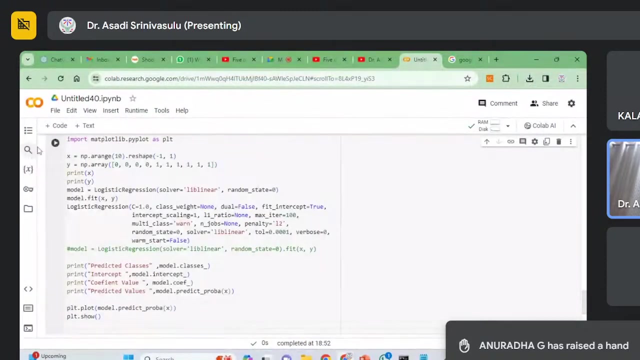 3 hours 70 marks. Now I am executing that program, logistic regression. What is the output we are getting See now? Now I am executing notepad space logistic. So this is the program, Sorry. So this is the program: control C. Now I am going to code here, Then paste it Now. 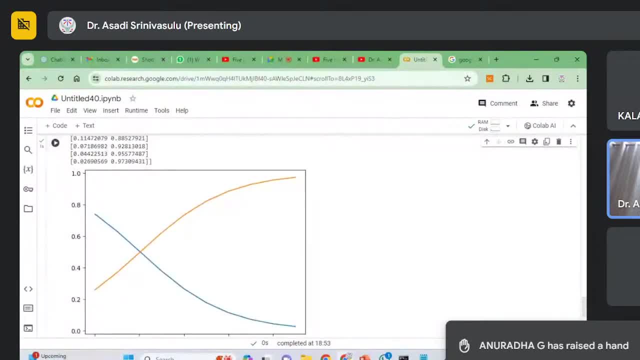 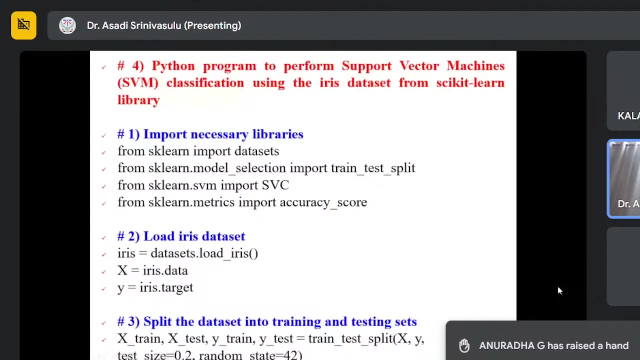 run. So here you are getting logistic. Now I got the logistic regression output. So here see, this is the program and this is the output. I got it. Next, support vector machine. So write a Python program to perform SVM classification using the iris data set from scikit-learn. 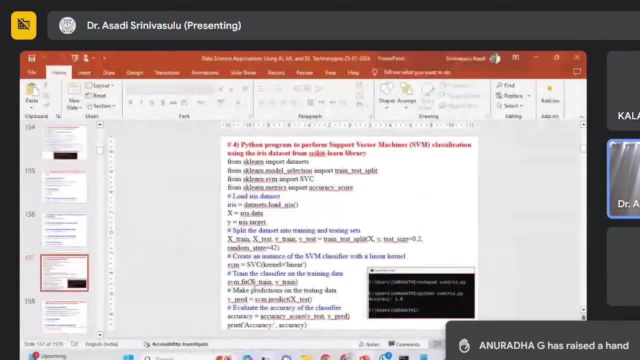 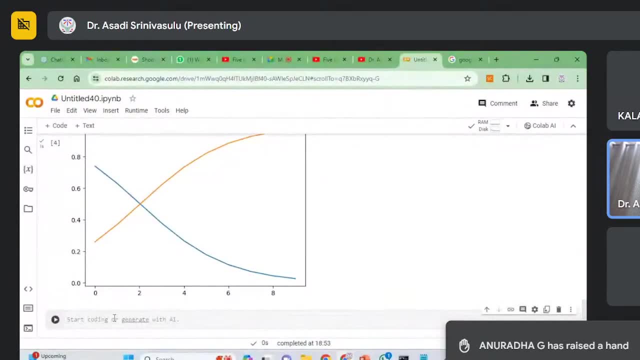 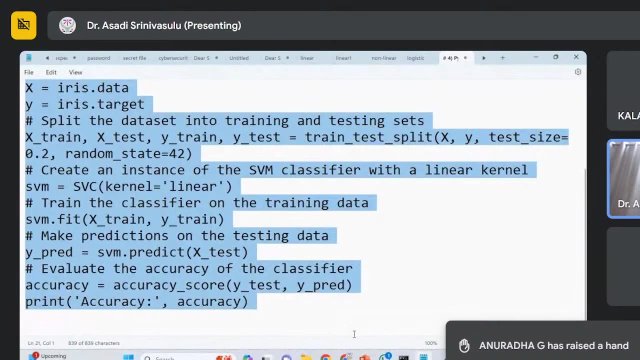 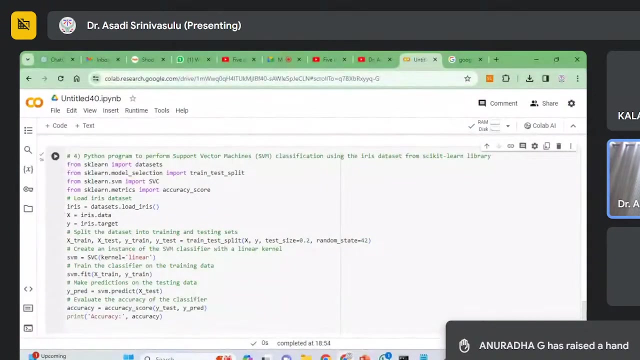 By using sklearn how to execute. This is the program I am going to demonstrate. now Control C: Go to Google collaboratory because all libraries are inbuilt. Okay, All libraries are inbuilt. So here you can paste. Now run the program. Now see Support vector machine. See, I got 100% accuracy here. Support. 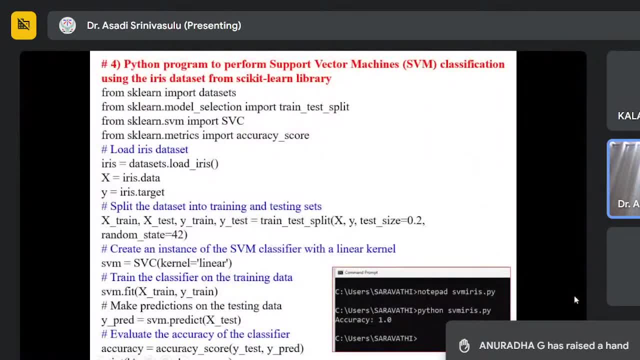 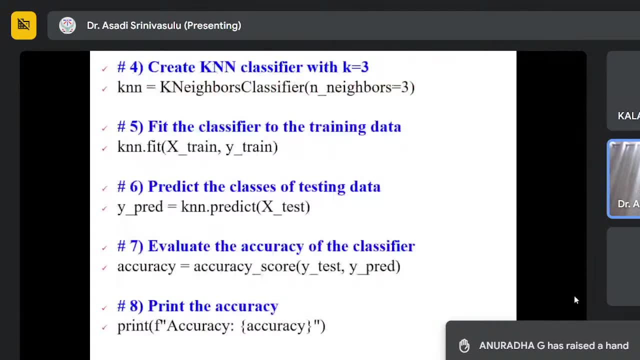 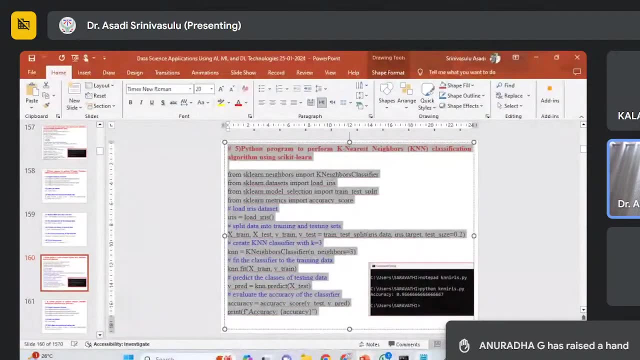 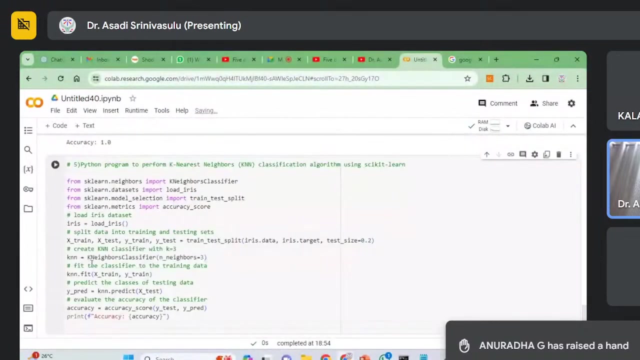 vector machine. Here is the output. Please check Next program: Python program to perform k nearest neighbor classification using scikit-learn. This is the output. I need to get it, So I am executing Next program. Okay, See Closest name. I am copying this 1 and pasting Write a. 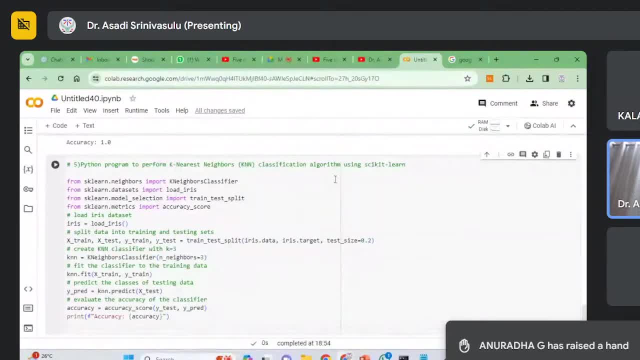 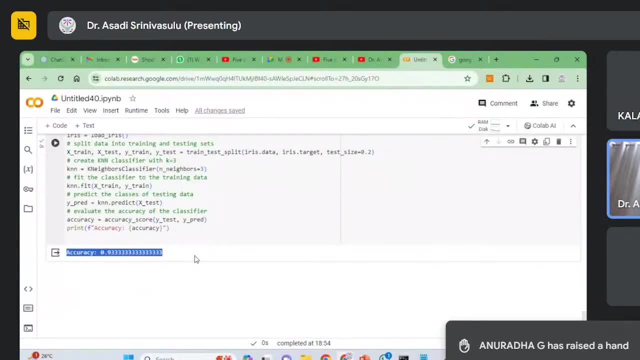 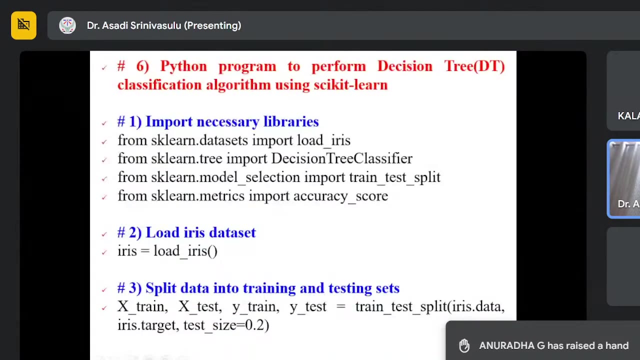 Python program to perform k nearest neighbor classification algorithm using scikit-learn. Now I am running the program. Now see the output. How much output? I got it: 93% accuracy. I got it. Same way. I have executed n number of applications. see decision tree. So decision. 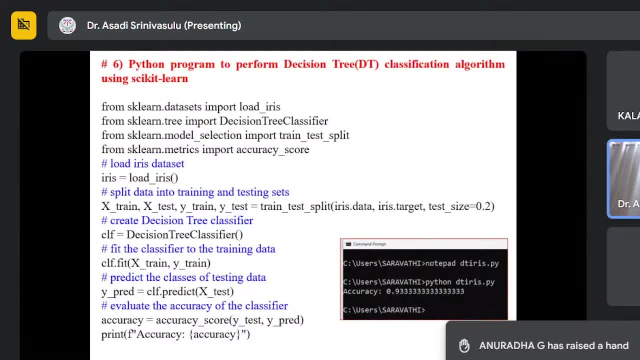 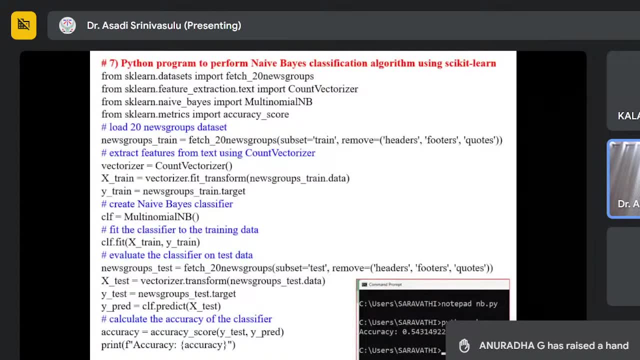 tree like Ad則 And bougاmarin Ist past captur And voor n graft een dan een a person a choose di connaaniędzyètgas var To model hope. I got 93.5%, and so Python programming by using Naive Bayes classification Python program. 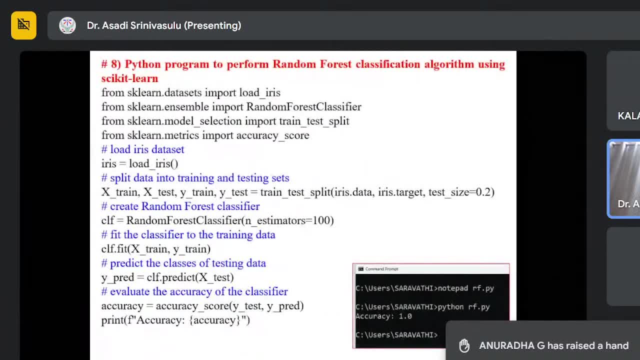 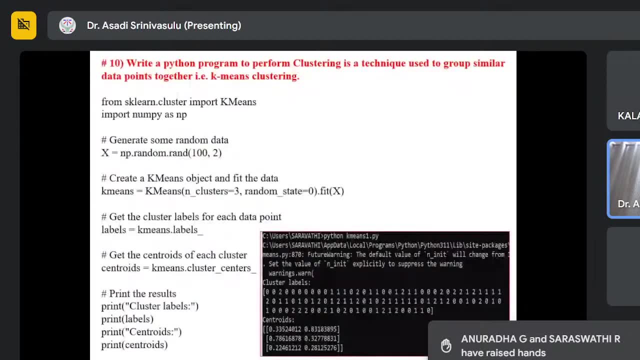 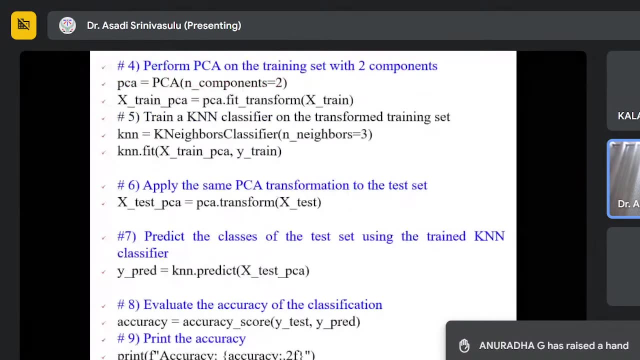 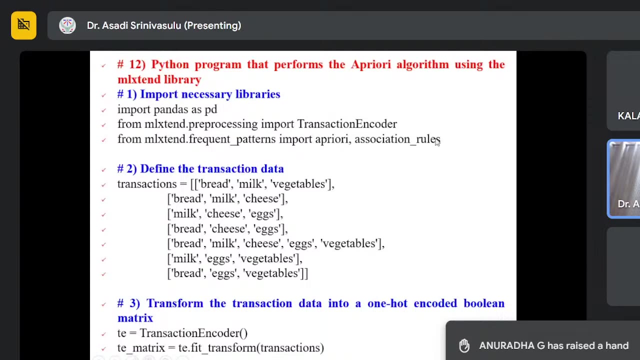 to perform random forest and random forest classification is scikit-learn neural networks. So this is a k-means clustering, and see. write a Python program to perform a k-means clustering- PCA- and see. this is the program I have explained like. write a Python program to perform Apriori. 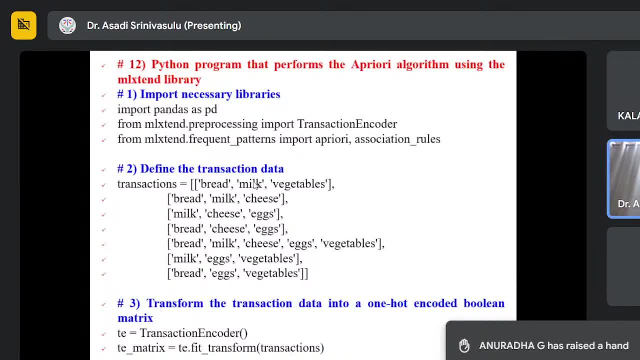 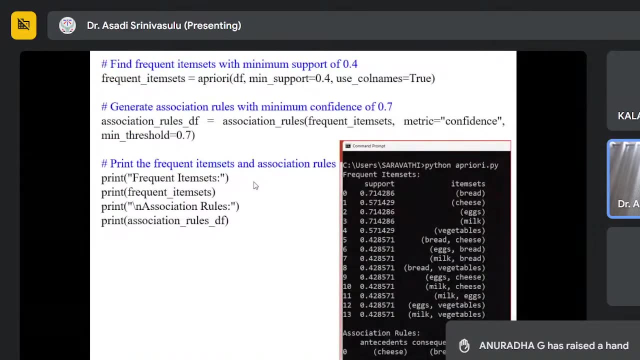 algorithm: See bread and milk. I have taken the data set like bread, milk, vegetables and bread, milk, cheese, eggs, vegetables, like that. Now I am predicting by using this algorithm. this is the combination- best combination- I am getting. 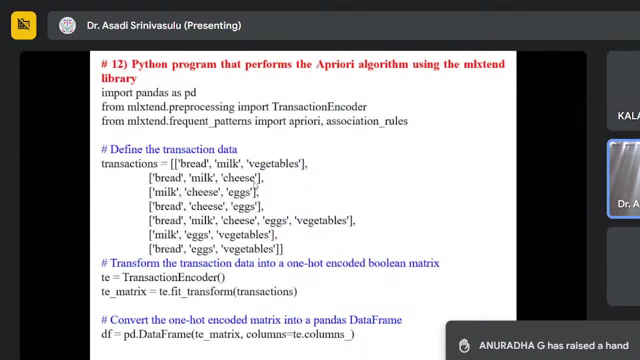 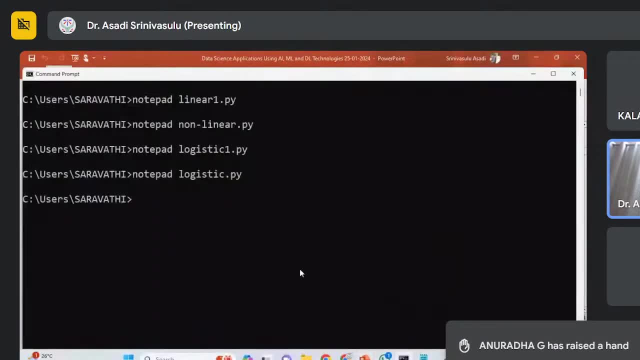 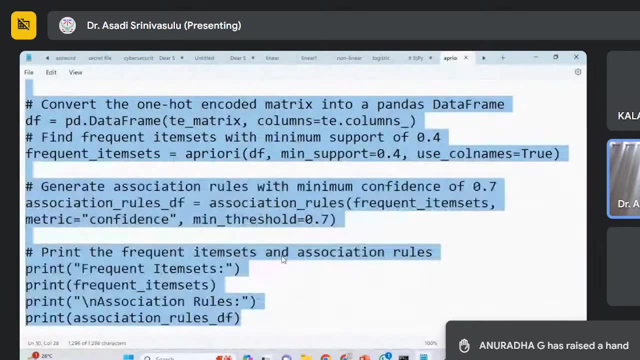 This is the results. Now I am going to demonstrate that one. Please see here what is the file name I have given. the file name is Apriori, dot. okay, See now notepad space: Apriori. see, this is the program. now I am demonstrating go. 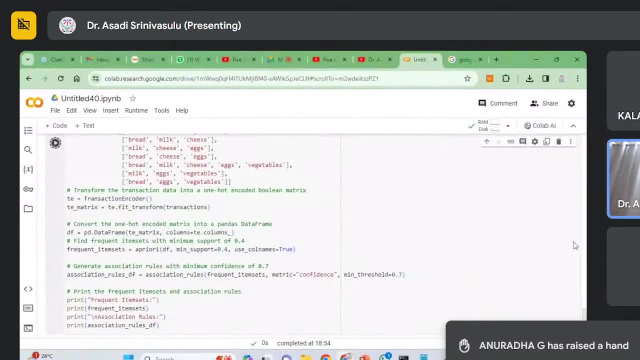 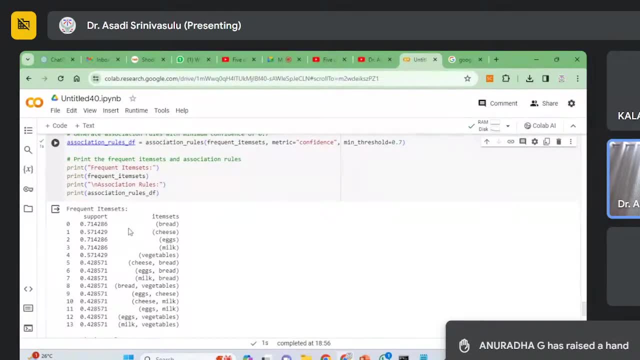 to code here: paste: see Now. I am generating the output. see now the item sets. please, my dear friends, 71% support. I am generating the output. See now the item sets. please, my dear friends, 71% support. 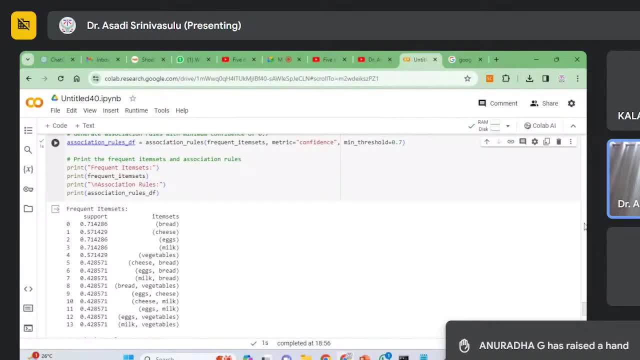 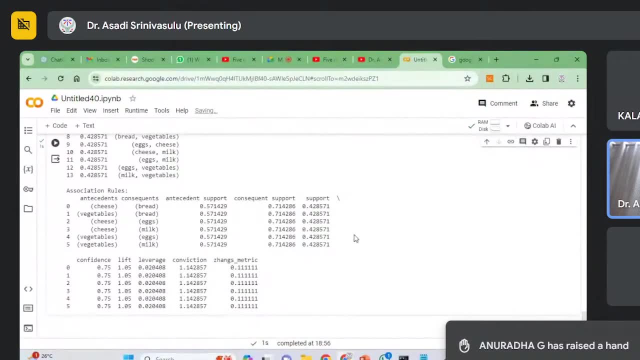 See now the item sets, please, my dear friends. 71% support. See now the item sets, please my dear friends: 71% support. burnout: yes. possible results: Bread cheese: 57% eggs. frequent item sets. 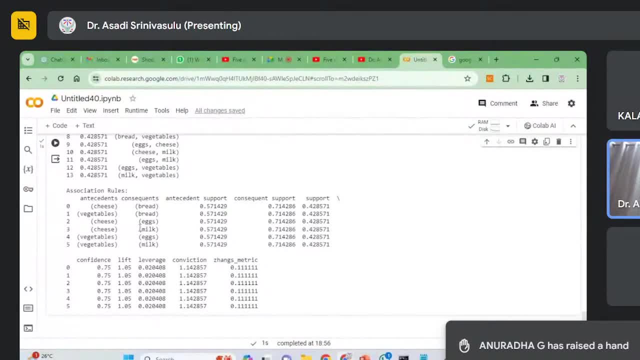 Can you see the association rule mining? what is the first combination? we got it Highest accuracy. Can anyone Please see here: bread and cheese, best combination. Then association rules: we got it best. five rules I have generated. My screen is visible. my dear friends, 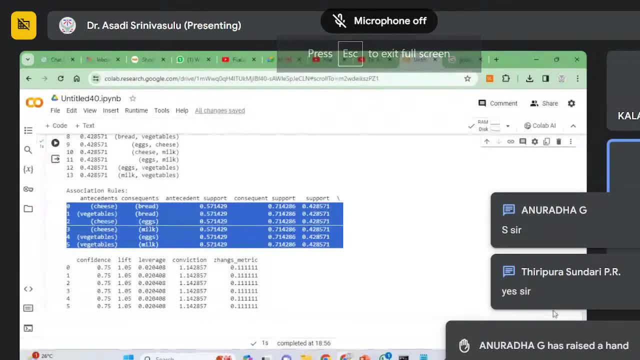 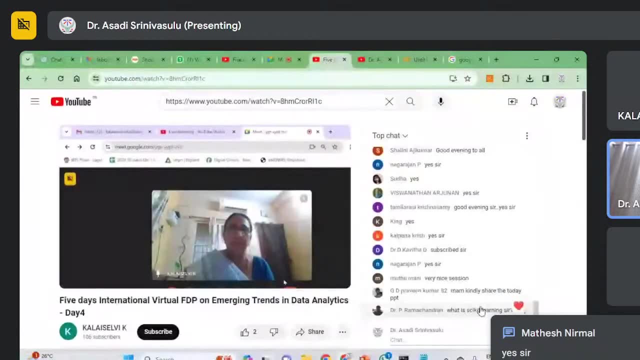 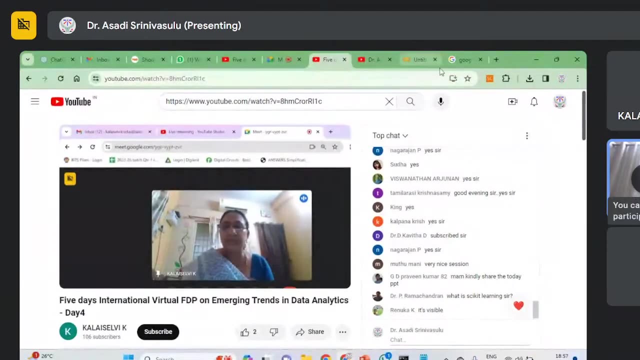 Hello. Yes, Sir. Any doubt, please ask me. Only three minutes is there. I have another meeting with my University of Newcastle. Please ask any queries. if you are having Demo, if you are having any doubts, please ask me. I am going to clarify. 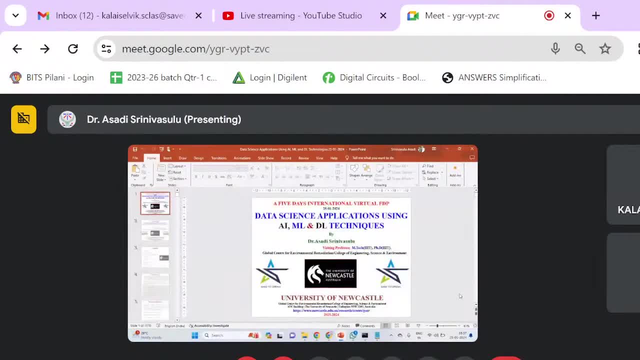 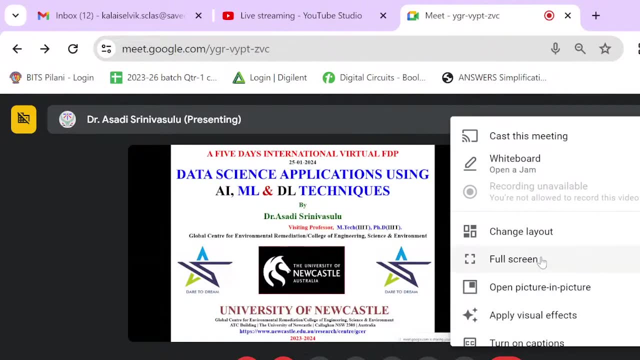 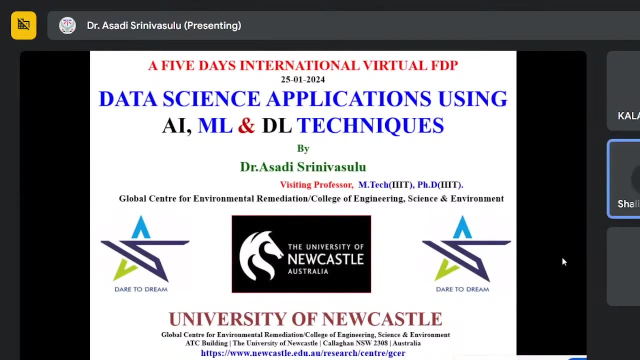 Madam, Hello, madam Sir, Yeah, yeah, Demo. please See, I am going to do many tasks, like I am preparing SEI papers, COPUS papers, If you want help in preparing research articles and thesis. also I am doing parallelly with my corporate training. 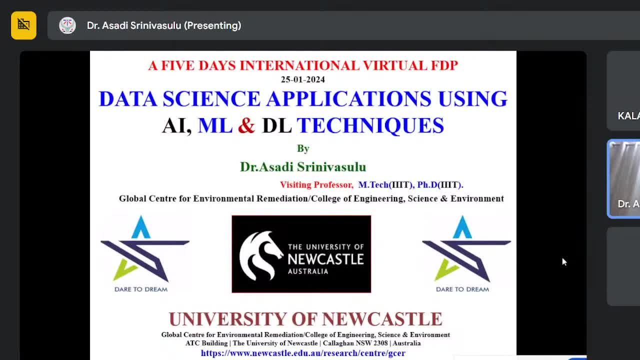 If anybody wants, I am going to publish research articles in SEI, COPUS Thesis, Thesis preparation. If you want help, I am going to help you With collaboration. I am going to help you. Yeah, please ask me any doubts. 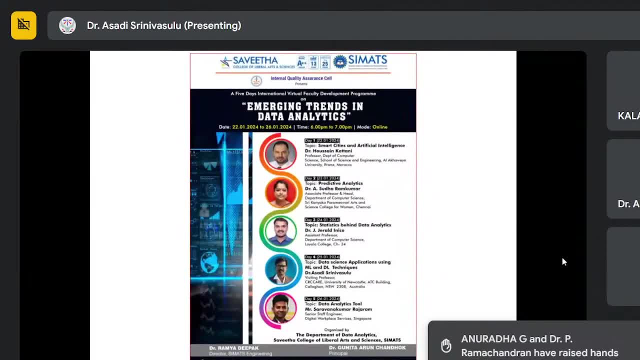 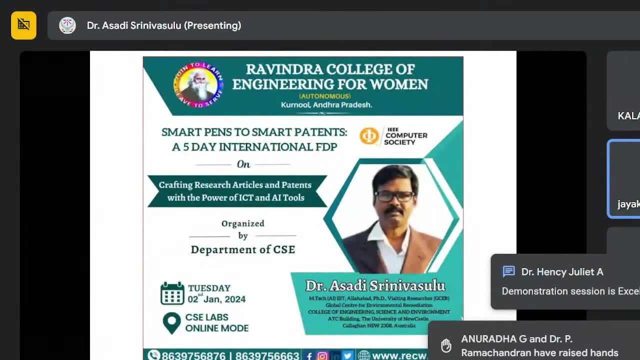 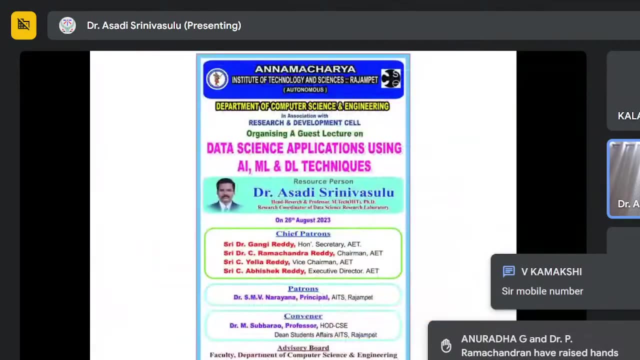 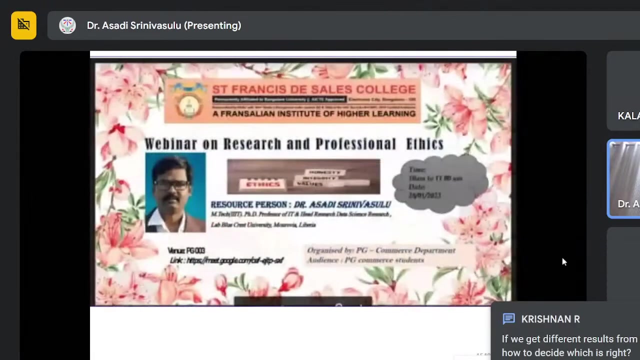 See, this is your Samhita Samhita, College of General Arts. Thanks. Recently I have conducted, Yes, I have conducted, I have conducted 175 webinars and seminars and workshops. See, these all are Various webinars, seminars, all over the world. I have created cyber security. these many 175. 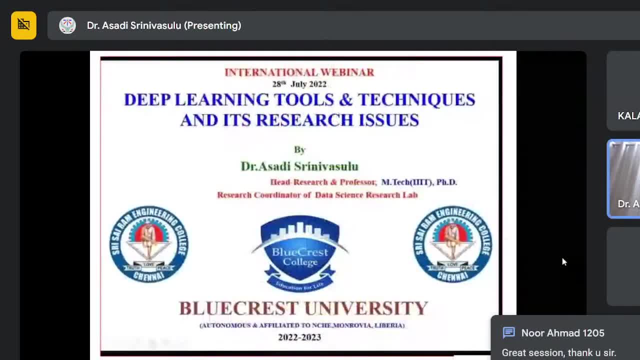 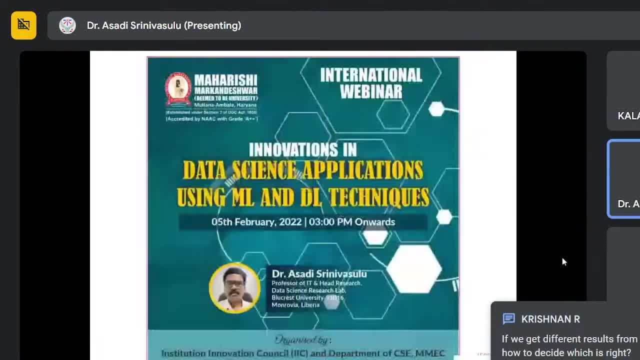 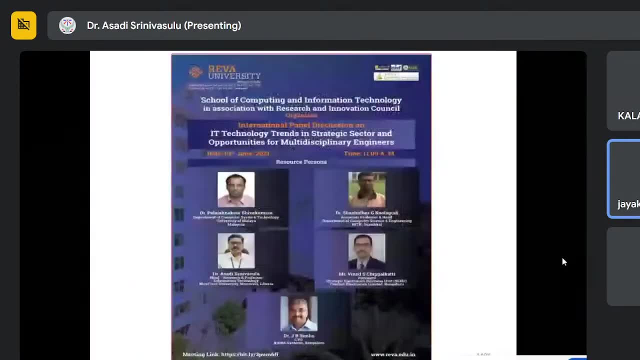 Within three years, I have conducted 175 physical and virtual workshops. I have conducted. Dear friend, if you are having any doubts, please ask me. I am going to clarify, Please. Hello sir, Yeah, yeah, please ask me. 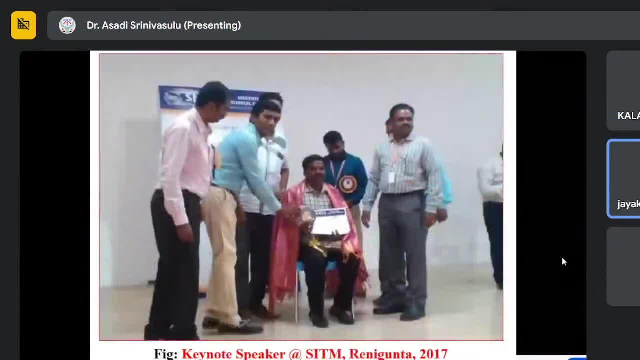 Sir, it's time. it's time. Hello, Sorry, Yeah, I am Jay. I have a doubt, sir. Yeah, yeah, please ask me, sir, Whether the Python only enough to exhibit all the concepts. what are you doing? Sir, if you are strong in Java, also see Java and Python are competitors nowadays. If you are strong at coding skills, then go for Java. Sir, I don't have that much coding skills, then go for Python programming. I am going to clarify. 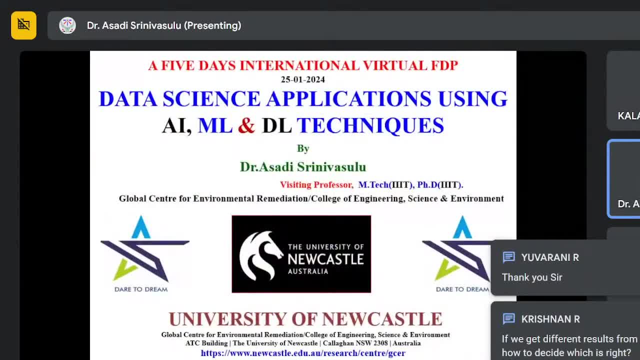 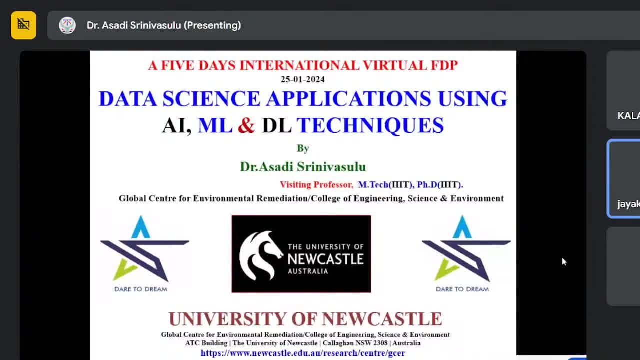 Why Python is so popular? Because of libraries are presented. Some lakhs of libraries are presented. So if you are strong in Python, then go for Python only. sir, Okay, okay, sir, okay, Thank you, Yeah, yeah. 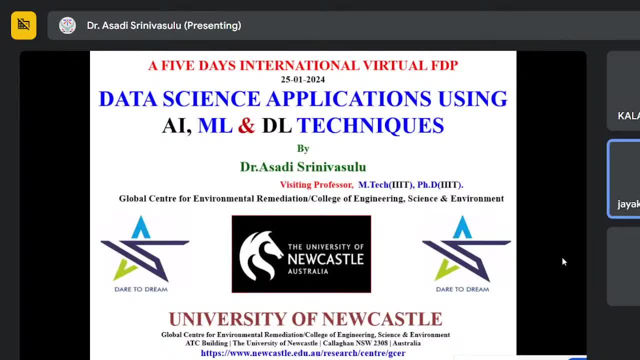 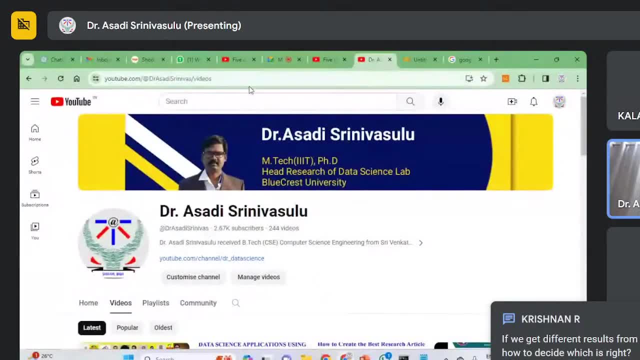 Hello sir, Your name, Hello sir, Yeah, yeah, I am Jay Kumar from Chennai. Yeah, Yeah, Very good, Very good, Very good question. Next, Anyone, Any question? Hello sir Ramachandran from Chennai. sir. 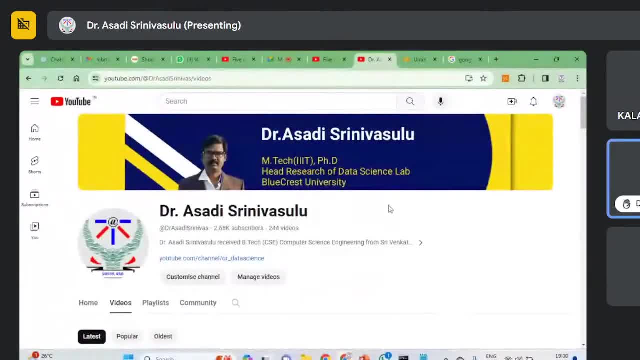 Yeah, yeah, please ask me something: Scikit-learn- What's the meaning for Scikit-learn? Scientific, see all machine learning algorithms like classification, clustering, association, rule, mining. if you want to perform machine learning approaches like supervised, unsupervised, reinforcement learning algorithms. 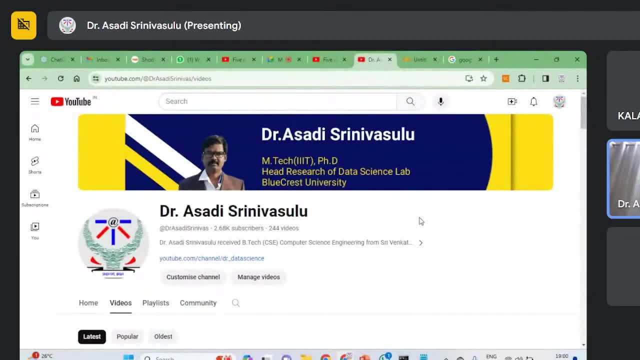 go for Scikit-learn. That is called a SK-learn. It is a library, It is a package, It is a framework In order to classify the data, in order to clustering the data, in order to perform association rule mining. 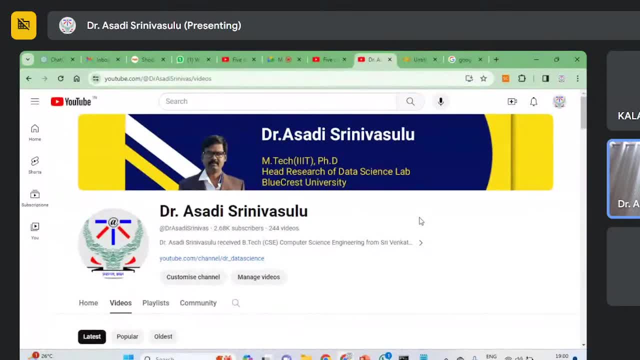 in order to perform outlier detection. we are going for a SK-learn That is called Scikit-learn. It is a framework, It is a library. Very good question, sir. Any doubt? Thank you, sir. Yeah, yeah. 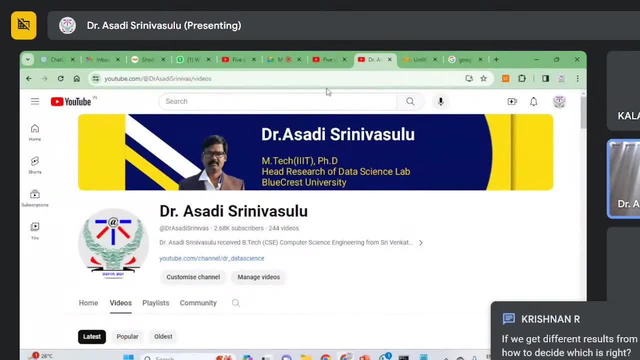 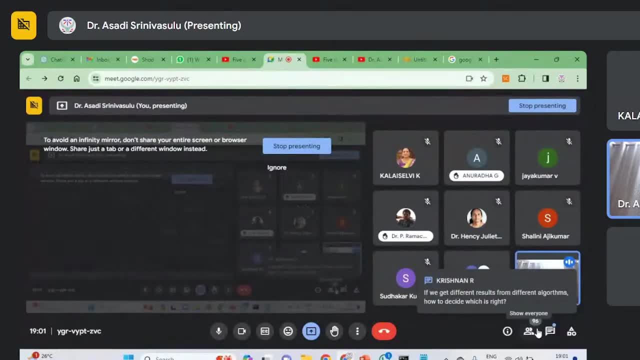 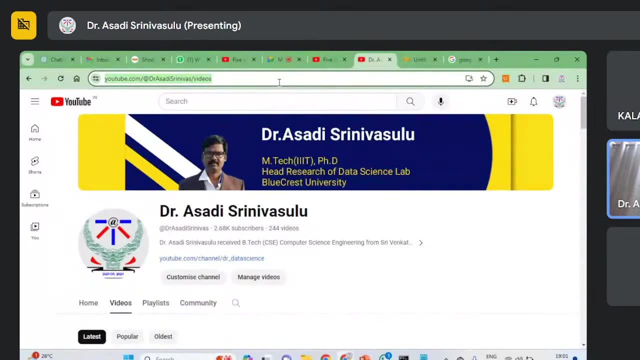 Please subscribe Only AC. So far, 24 members only subscribed. What happened to remaining 96 members? are there? Can I expect 96 members? at least 90 members? Please go to my channel and subscribe. I am not using any money purpose. 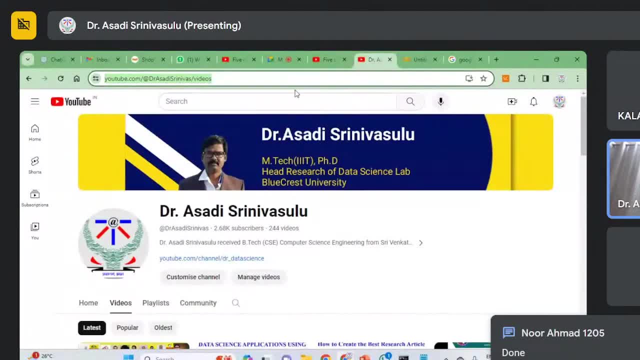 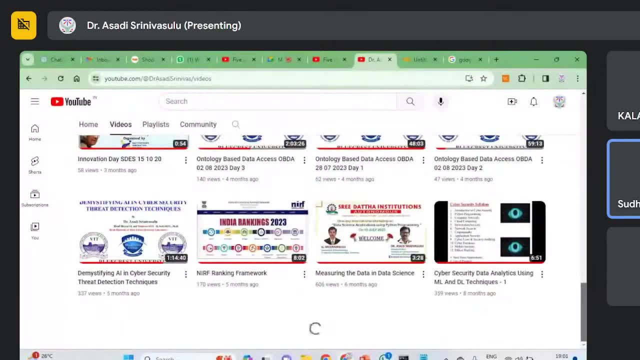 Just if you want to listen, you can listen. No problem, Sir, excuse me, sir, Sir, one doubt sir. Yeah, yeah, please, I am Suzhakar here. I have a small doubt, Sir. what about the reliability? 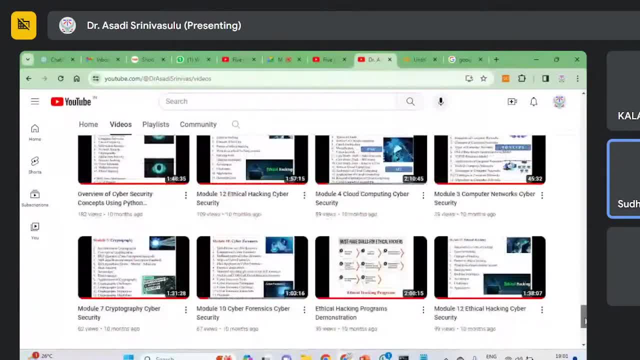 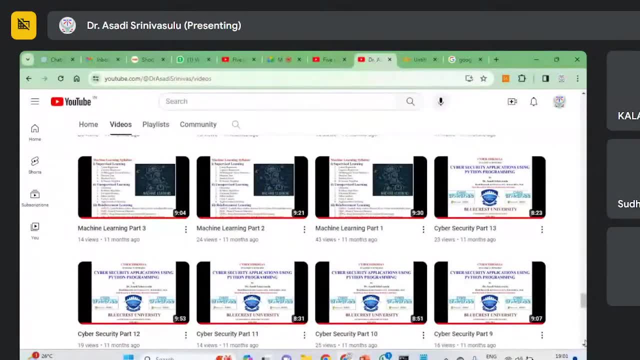 While Using confusion matrix for the support electron machine or navies, bays, whatever like that, Or logistic regression also. Yeah, yeah, See confusion matrix we are using for to find out the accuracy, How many items are correctly classified. 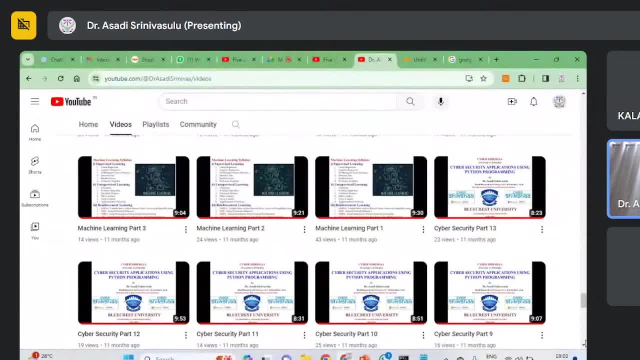 How many items are wrongly classified. For that purpose we are using confusion matrix. If you use for classification, clustering, confusion matrix, it gives accuracy. So the reliability, see, depends on the data set, what you are taking, So automatically you can apply confusion matrix. 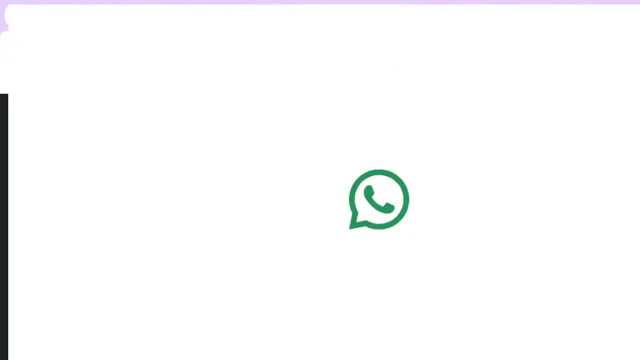 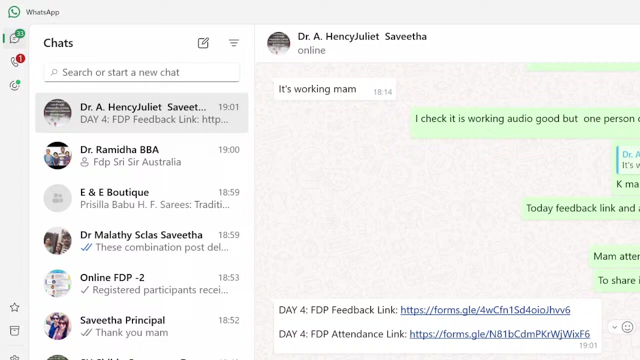 You can generate confusion matrix. Suppose 200 item sets you have taken, So it classified only 100 correctly classified and 100 wrongly classified. That means the confusion matrix says that false positive, false negative. Okay, true positive and true negative. 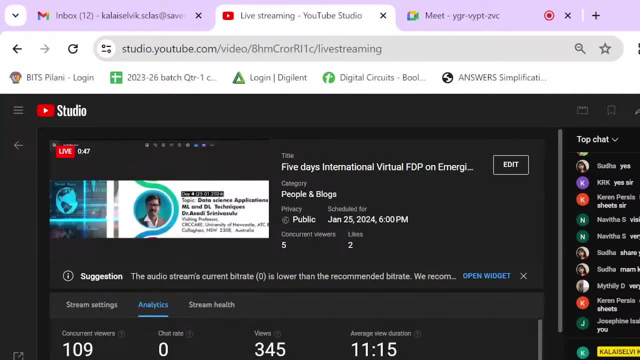 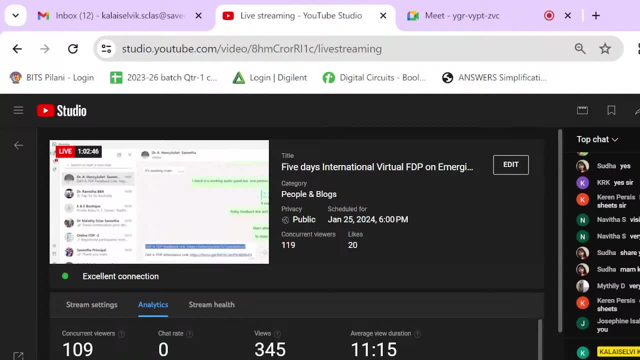 So it calculates the, The, The, The, The, Correctly classified by number of total items. That gives the accuracy of the proposed model. Very good question, sir. Very good question. Thank you sir. Thank you, Thank you sir. 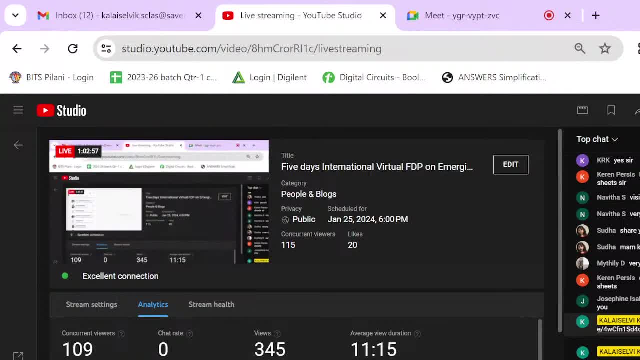 Yeah, Yeah, please. Any doubt, please ask me. So far, only 34 members, sir, subscribed my channel. Any doubts, please ask me. Dr Asadi Srinivaslu, if you type, you will get it. 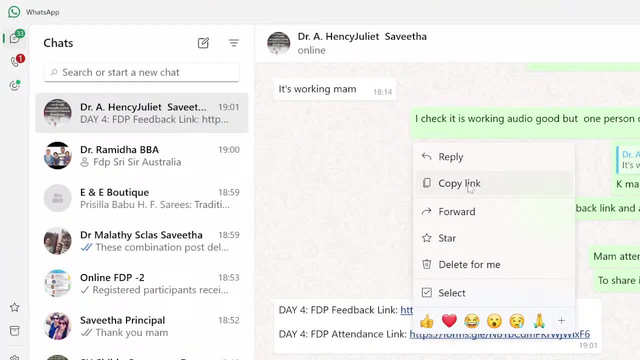 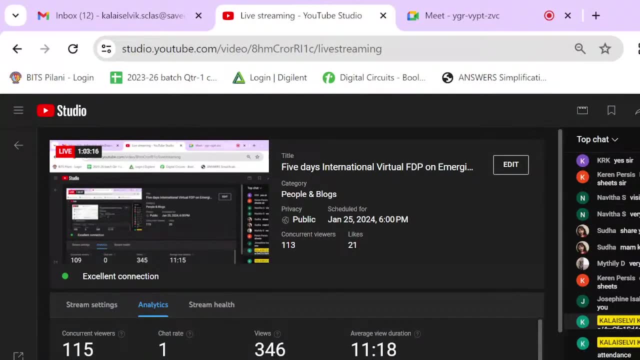 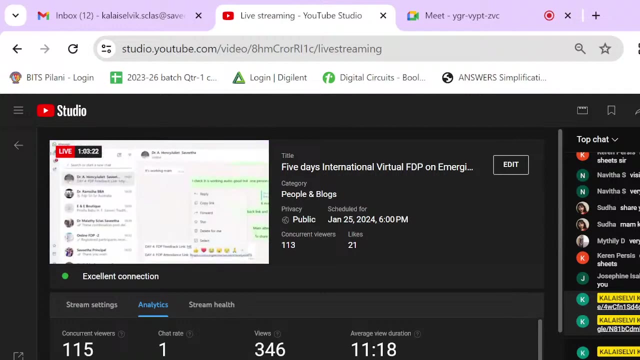 Madam. You ask, madam, Is there any, Any other doubts they are having? I am going to clarify. Please, My dear friends, no hesitation If you want any collaboration with me. research article preparation: See. recently I have conducted how to create the best research article by using AI and ICT tools. 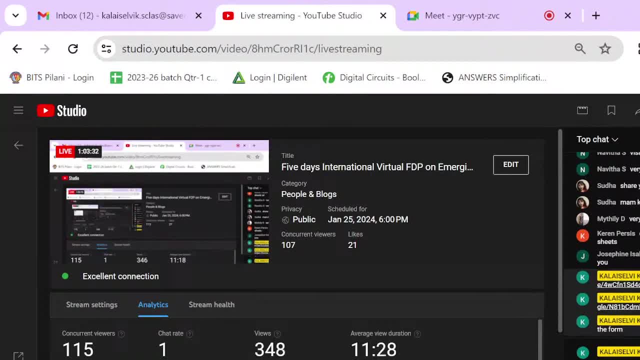 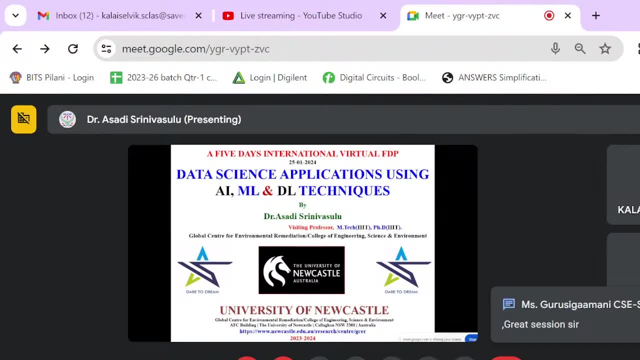 So one day it is enough for me to create the best research article and we can upload And in SCI and Scopus journal. That workshop I am going to do, physical. Okay, Yeah, Anyone, please? any doubt? please ask me. 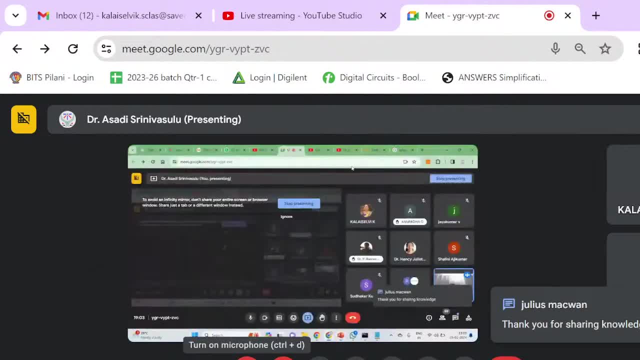 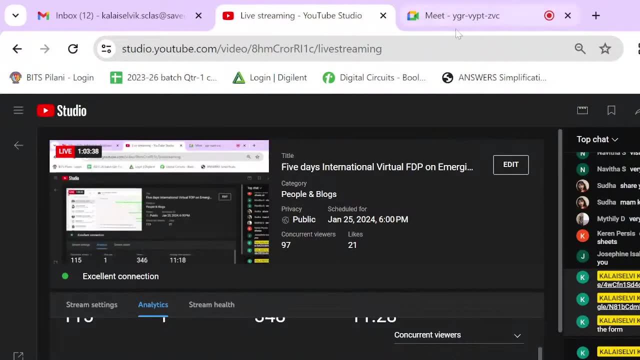 My dear friends. madam, Anyone having any doubts, please clarify Participants. if you have any doubt, you can clarify your doubt now. Yeah, Hello, Hello sir, Good evening sir. Yeah, please, madam, Tell me. 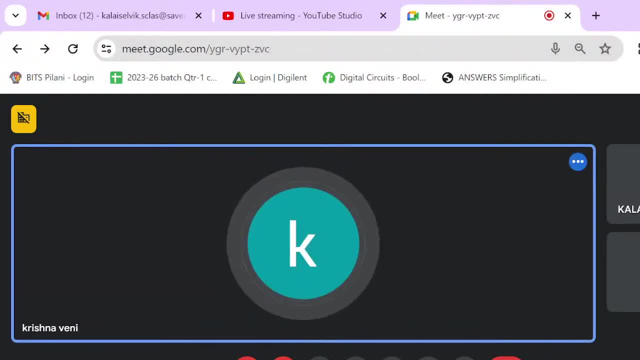 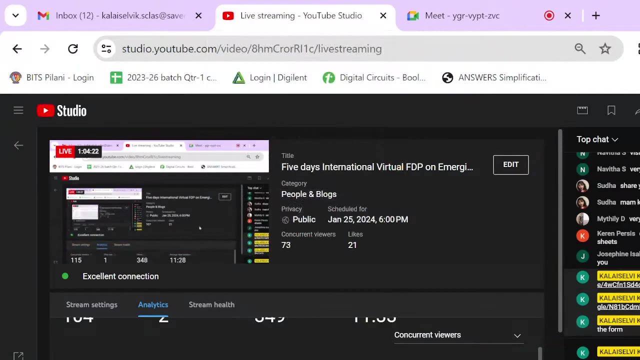 Yeah, Sir, actually In a research paper, if you can take some of the content- I mean ideas from the AI tools, Yeah, correct, Something to be like that. But if you can, The same thing, if you can write in the research paper. 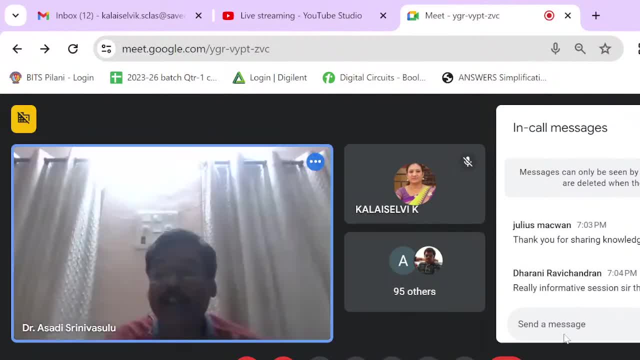 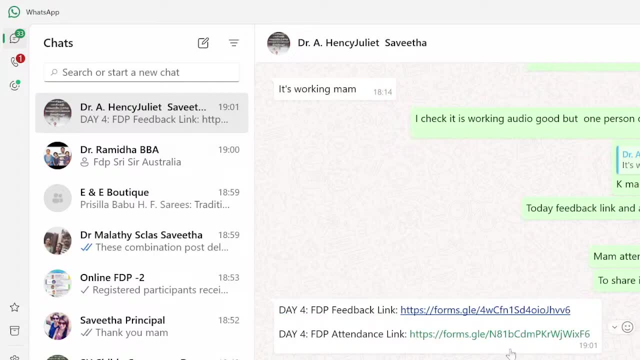 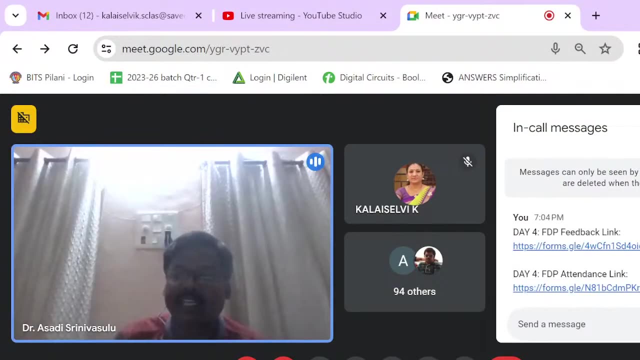 No, there are AI plugins. are there? Be careful while using AI tools. It will show you 100% plagiarism. That's why. That's why there are some tips and techniques. if you use, We can create the best research article by using AI tools. 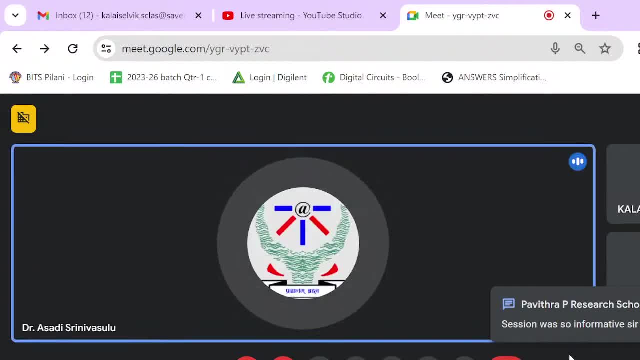 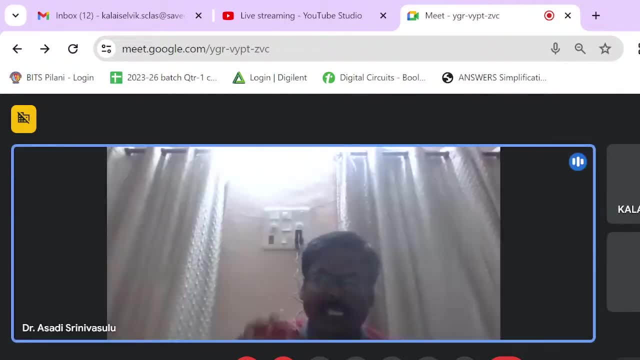 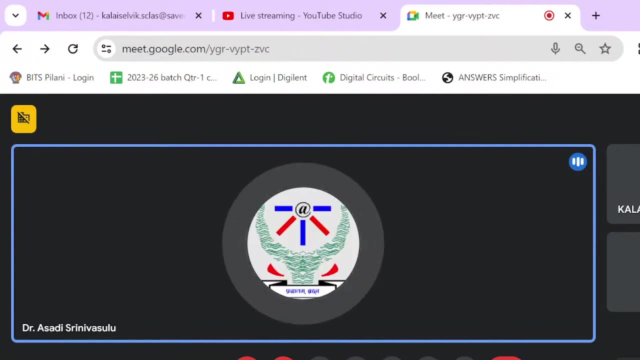 But don't go for copy and paste exactly whatever it is giving. There is a plugin. There is a plugin called AI plugin is there in the Turnitin software. It will catch where you have copied and pasted And it will do, while doing that, copy and paste. 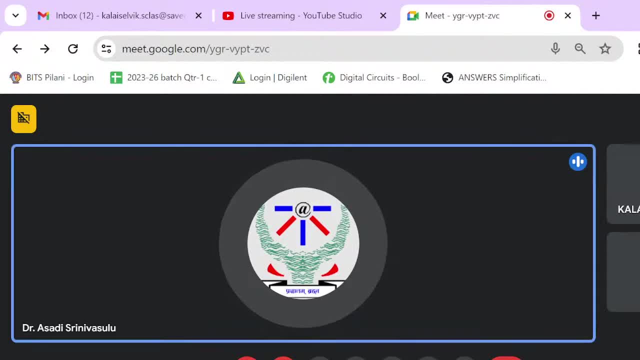 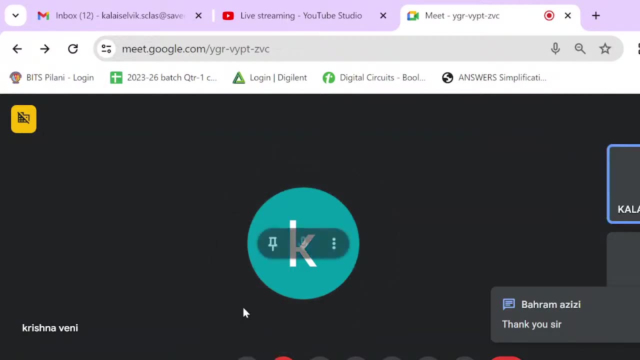 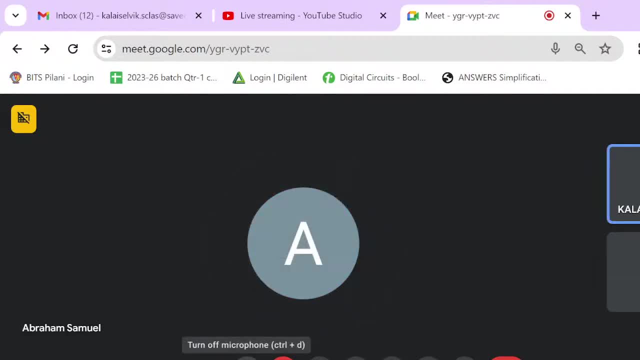 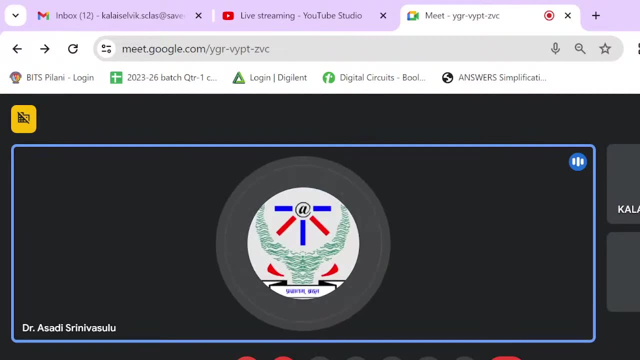 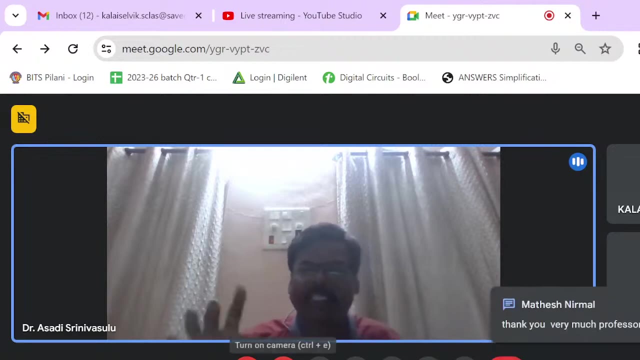 Okay, Okay, Okay, Okay, Okay Okay. There is a feedback form in the group chat. Please fill up all of your feedback. All of you come in to the video so that the coordinators will take the picture and they will prepare the report. 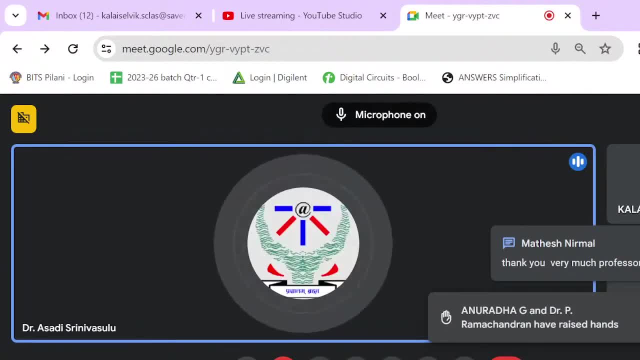 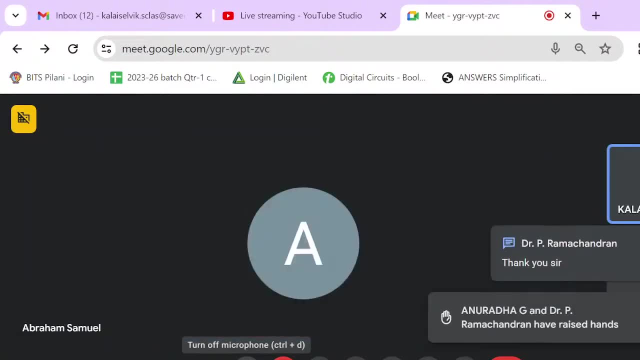 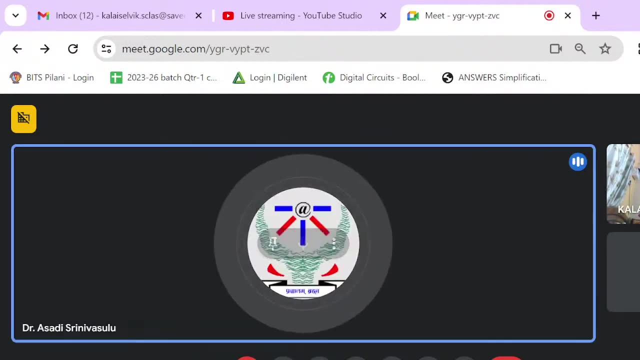 This of all of you, all cameras. they will take a snap shot so that the Madam I have conducted a numerous. The camera is not able to. The camera is not able to. Okay, Please open your camera and take. the coordinators will take snapshot and they will prepare. 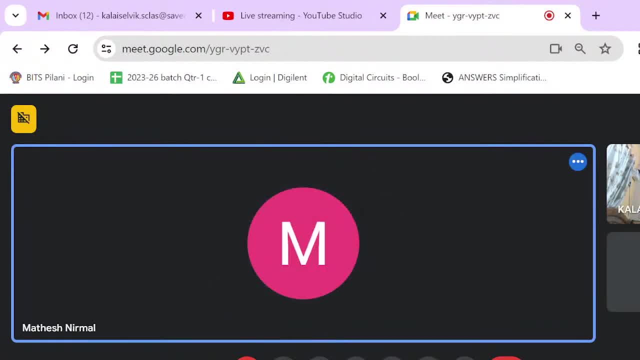 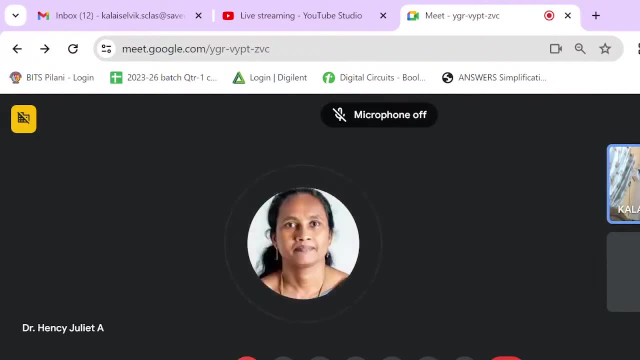 I hope that the coordinators has been blocked. They will do it themselves For the video. No, sir, Please come in the video. Yeah, please take madam's snapshot. Yes, sir, It is blocked by user for using your camera. 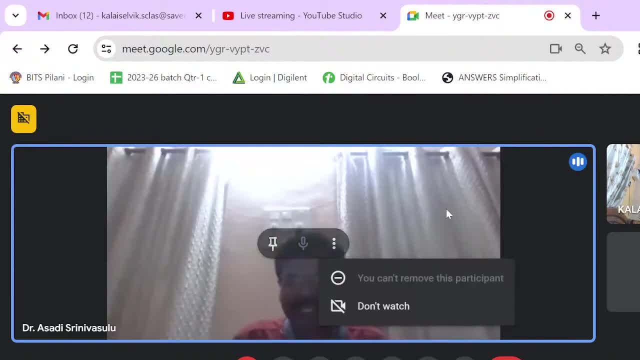 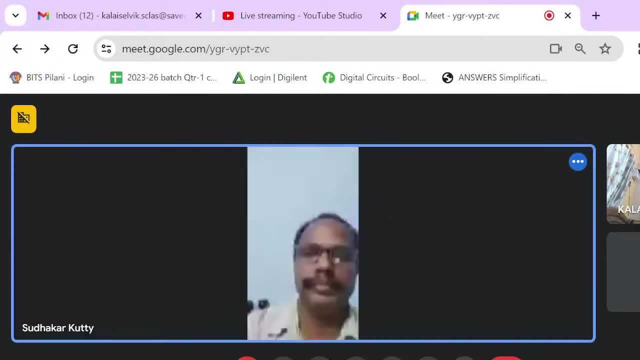 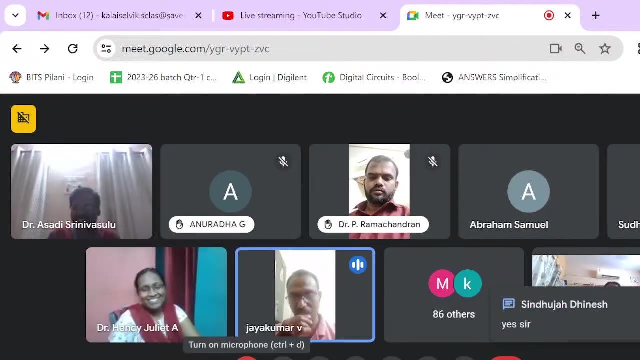 Any doubts? my dear friends, Do you like the session? Please give open feedback. I would like to see open feedback. Do you like my session or not? Yes, Yes sir. It is really sir. Yes sir, Yes sir. 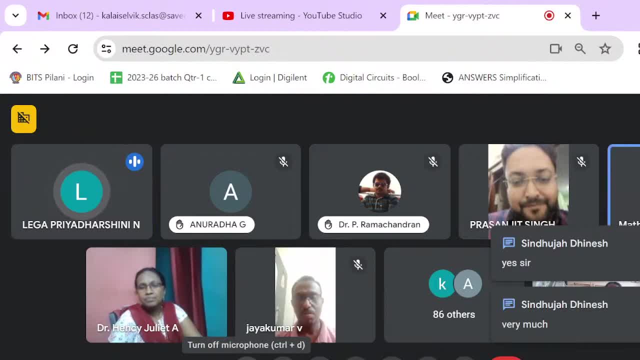 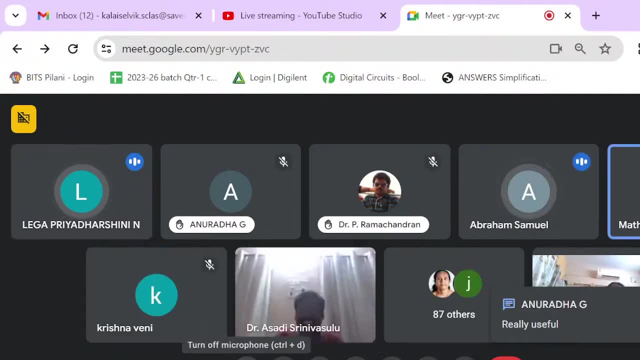 It is really. Yes, sir, Yes sir, It is very good and really excellent. sir, I am PVirmadhar from SESV University of Kanchipuram. Within a short duration of the time, you have given lot of information regarding the research. 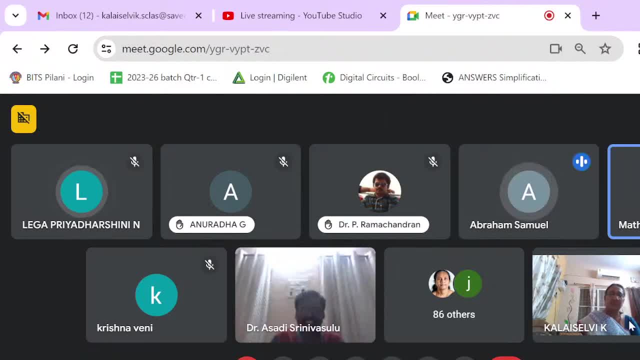 in what way that you want the implementer in AI. Yes, sir, And how to prepare over the paper also Very excellent. Thank you very much for your short time of duration. Thank you, sir. Thank you sir. Thank you, Mathis sir. 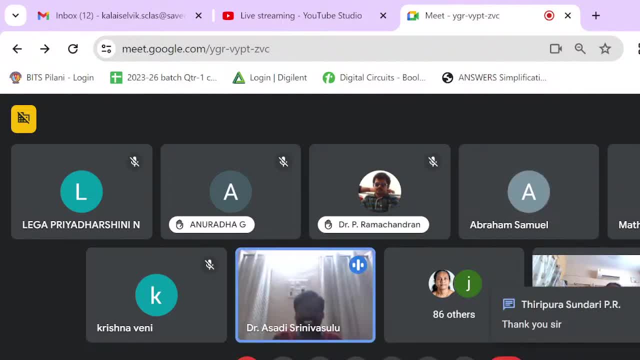 Thank you. Any open feedback, please? No problem, Your session is very interactive, sir. Thank you, sir Sudhakar. sir, Thank you. Thank you, sir. Yeah, Yeah, Sure, Yeah, Sure Yeah. 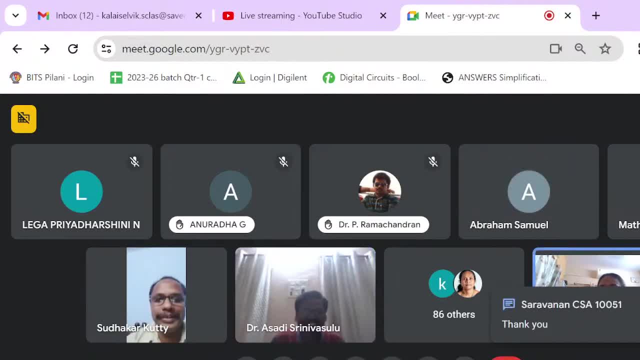 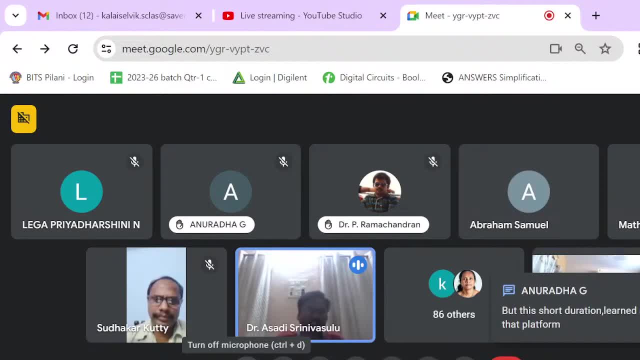 Recently, I have conducted 10 to 15 colleges, universities all over the world. I have been doing these. Surely we will invite you, sir. Yes, surely, Yes, Okay, I am going to share with you my PPT also. 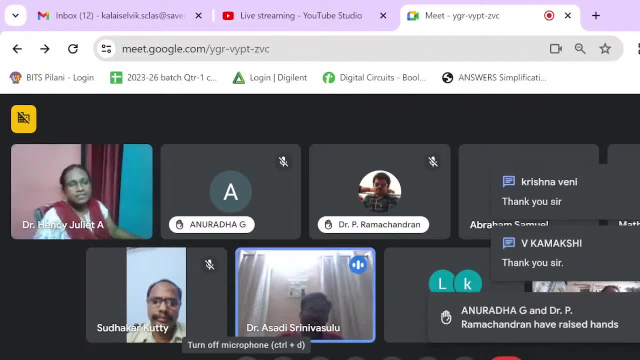 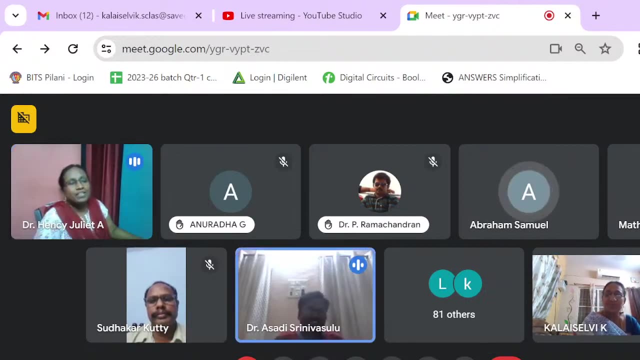 You can explore yourself and you can gain knowledge. Thank you so much, sir. More and more sir, More and more sir. Thank you. Most of the participants are asking: can you share the PPT? Yeah, yeah, So reply to the question. 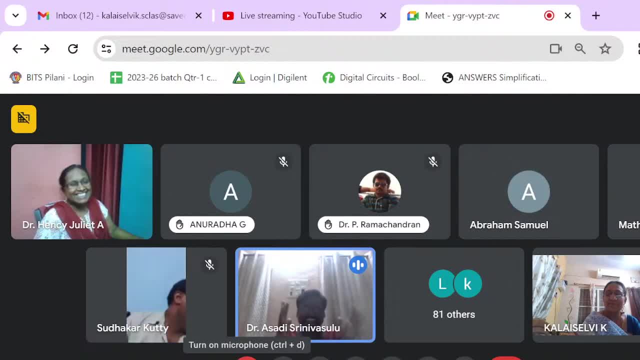 Without asking you. I am saying, madam, this is knowledge, sharing knowledge. I am not hiding anything. I will give you, Don't worry, Thank you. Thank you so much, sir. Yeah, If no, queries coordinators will give feedback on this one-hour session.